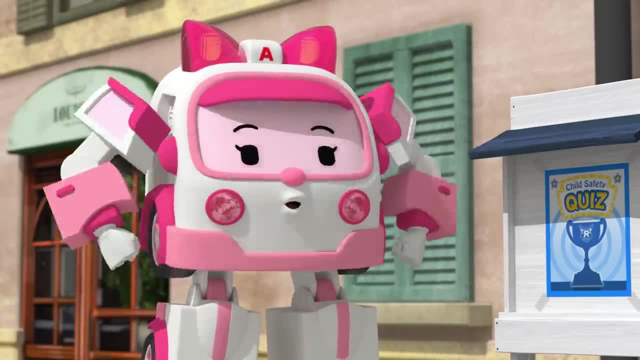 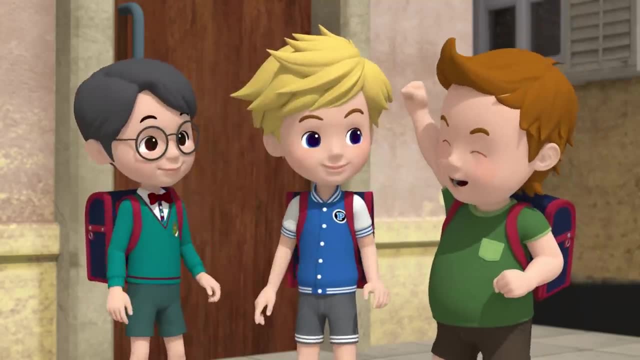 That's not true. Think of all the safety lessons that you've learned and you'll do fine. Heh, that's a lot, Guys. should we do it? Sure, Sign us up. Citizens of Broomstown, welcome to our first kid safety quiz competition. 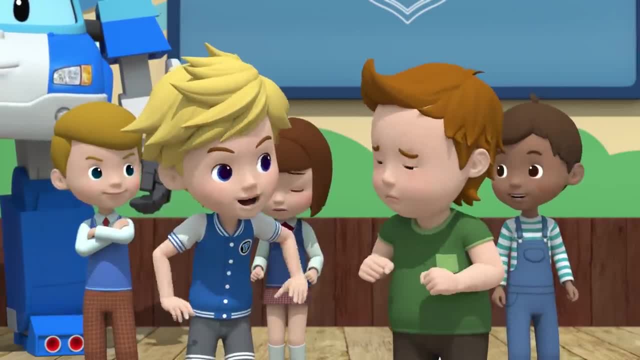 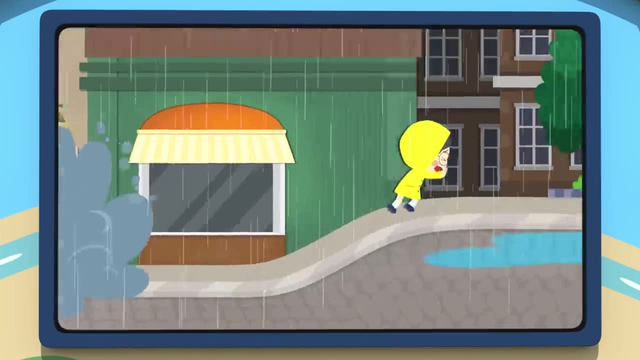 I'm so nervous. Don't worry, We've been through so much, We'll be fine Alright. the first question is: In a storm, is the safest option to find the highest point of land and stand by a pole? Stand by the O for yes. 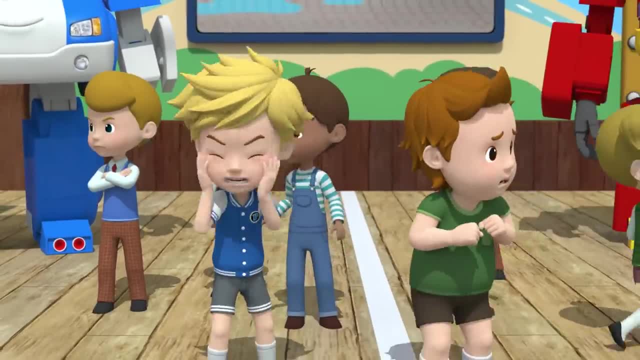 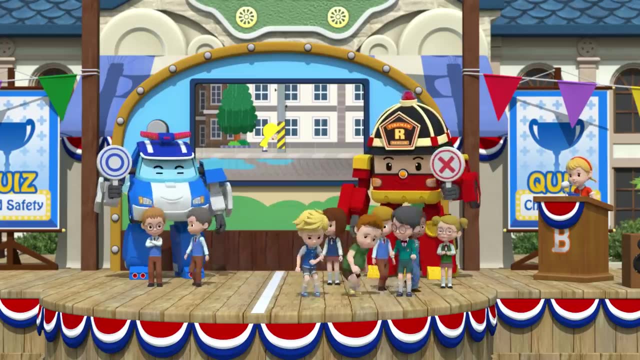 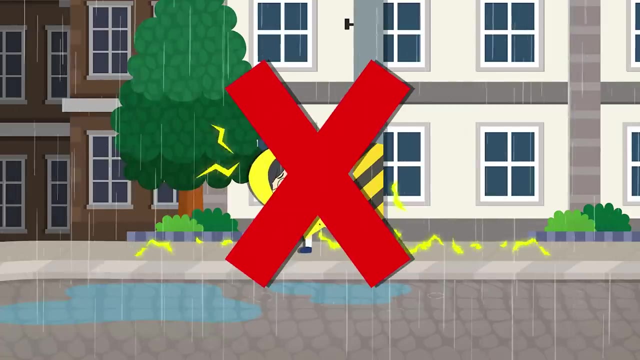 And the X for no. What, the what? How am I supposed to know Which one's right? X, Let's go to X. And the answer is X, for no Lightning is more likely to strike a tall metal object. I knew that. 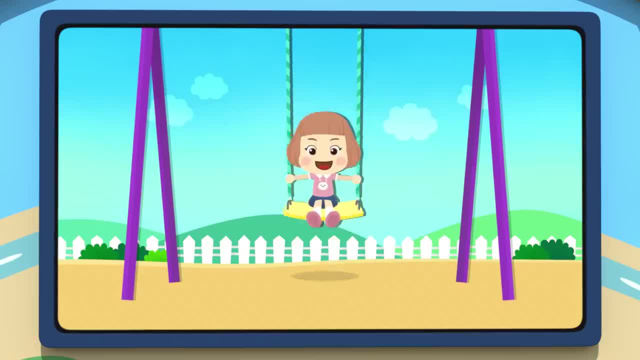 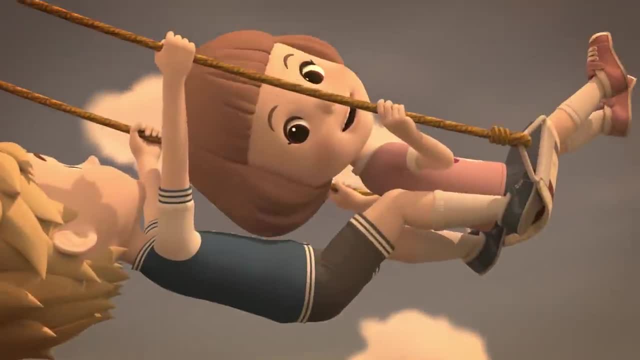 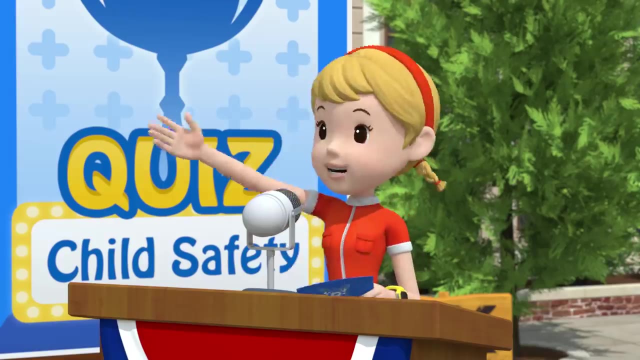 We just made it. The next question: When you're on a swing, always hold tight with both hands, Not if you're really good at it. Although There was that one time, I think I'll go with. yes, The answer is. 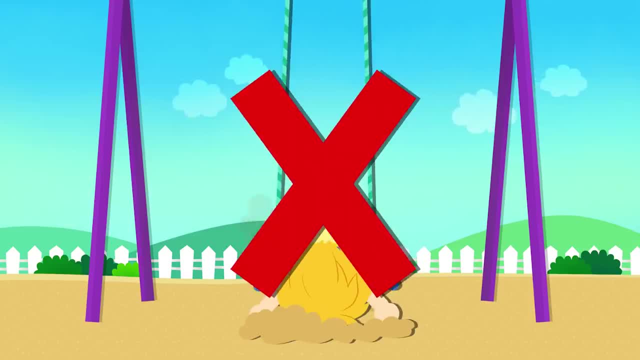 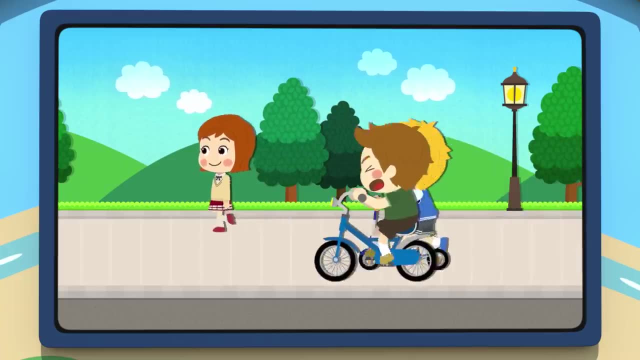 Yes, If you're not holding on, you could fall and get hurt. Be safe and hold on tight. I almost blew that. The next question: Is it dangerous to race your friends on your bikes when you're riding down the street? Stand by the O for yes. 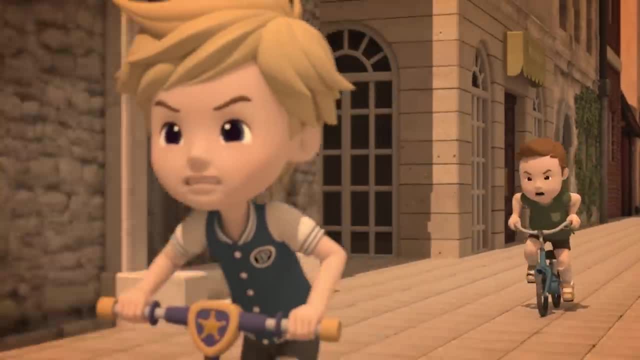 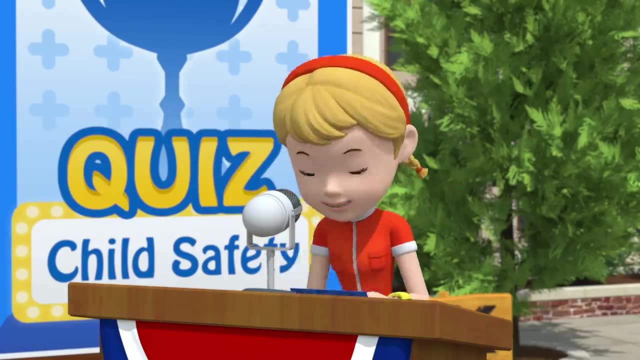 And the X for no. There was that one time I was racing Johnny on my scooter and I totally wiped out. And the answer is Oh for yes. If you're too focused on winning, you can really get hurt. I got it right. 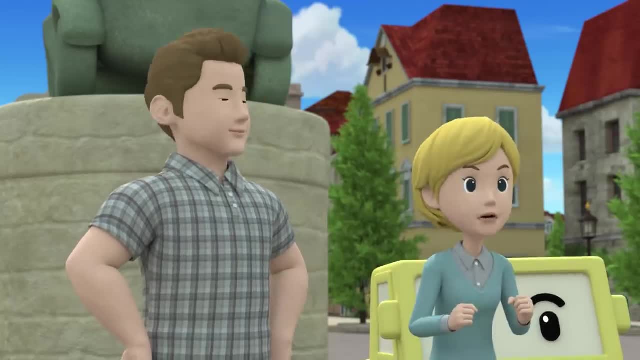 I knew it. Oh my gosh, Peter keeps getting them right. That's my son. Watch this video and choose the right answer. Who is using the stairs correctly in the following examples? Option one: the children playing as they go down the stairs. 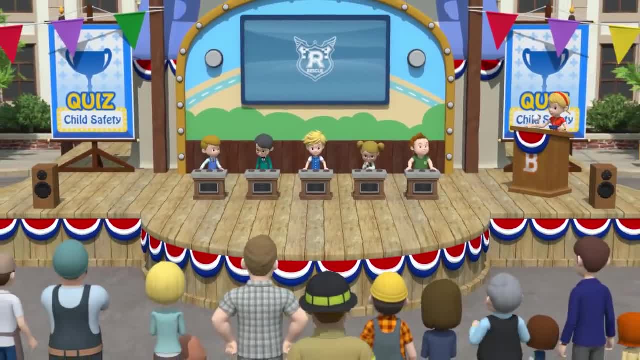 Option two: the child sliding down the handrail. Option three: a kid playing with a game board. Option four: a kid on the bike. Option five: a kid on a bike. Option six: a kid on a bike. Option seven: a kid on a bike. 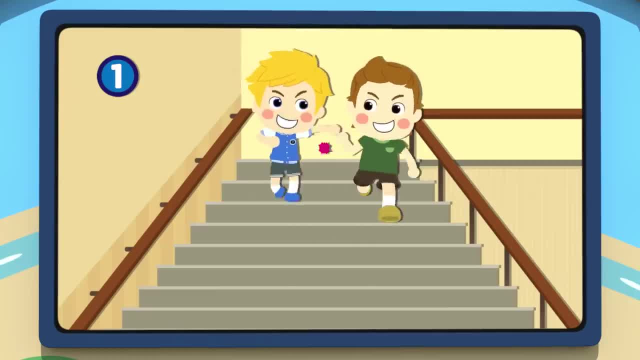 Option eight. a child on a bike Option nine. a kid on a bike Option 10, a kid on a bike Option 11, a kid on a bike Option one. the children playing as they go down the stairs. 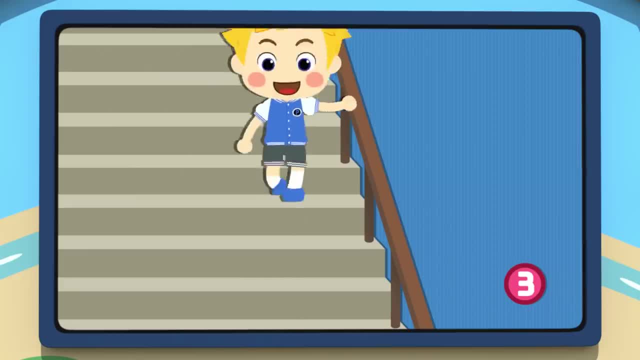 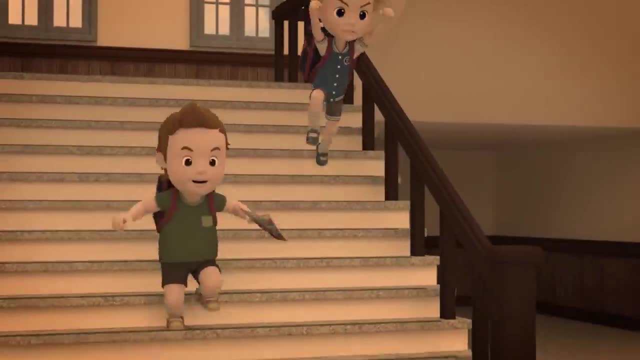 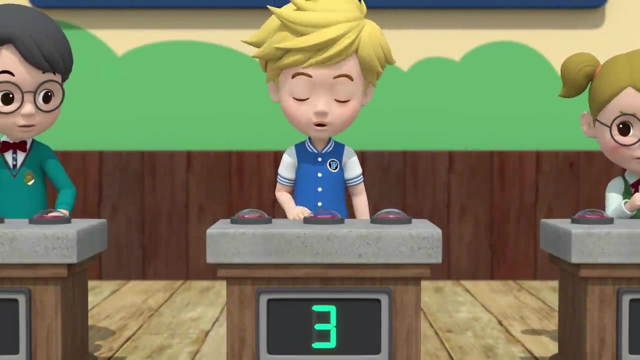 Option two: the child sliding down the handrail. Option three: the child holding the handrail as he walks. Oh, those times that Johnny and I were playing around on the stairs, I almost got really hurt And the answer is option three. 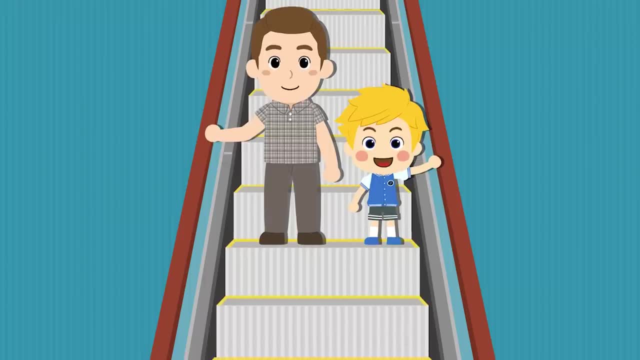 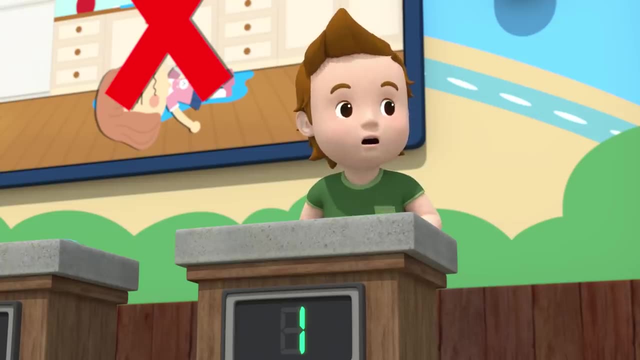 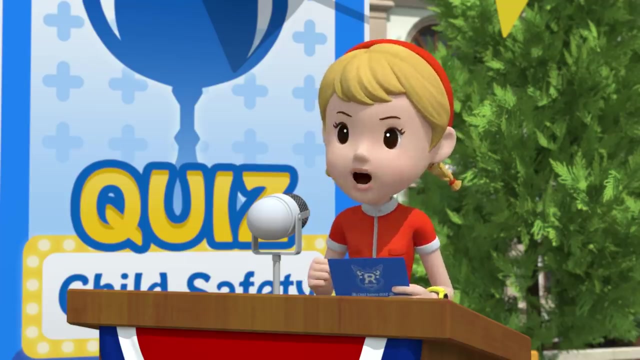 Why didn't I pick that? The answer is one: always hold the handrail when you're on an escalator, Right? The answer is two: clean up spilled liquids immediately. And the answer is two: ha. Water and electricity never mix. 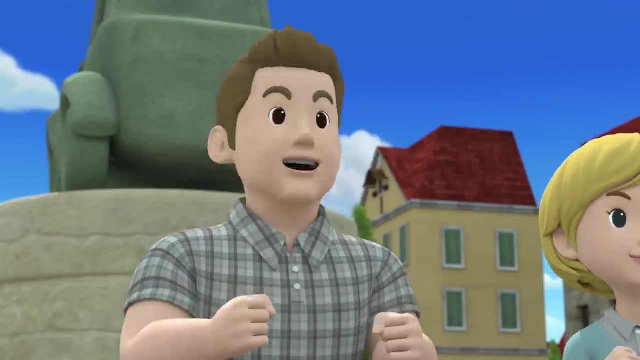 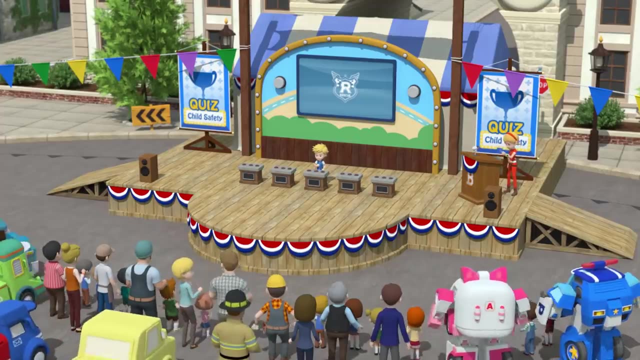 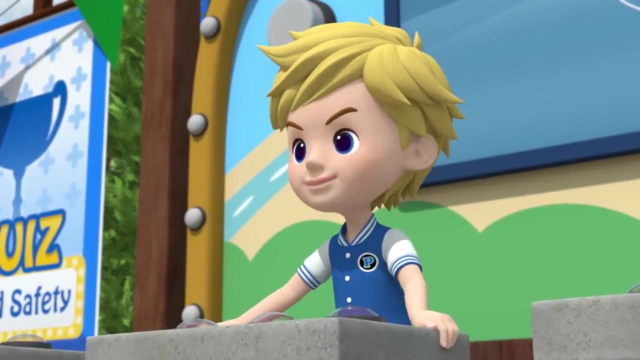 Yahoo, Peter might actually win this thing. What do you mean? might Peter, Peter, Peter? And now we come down to it. The last question of the competition. If I get this, I'll be the champion, and the question is: what should you do? 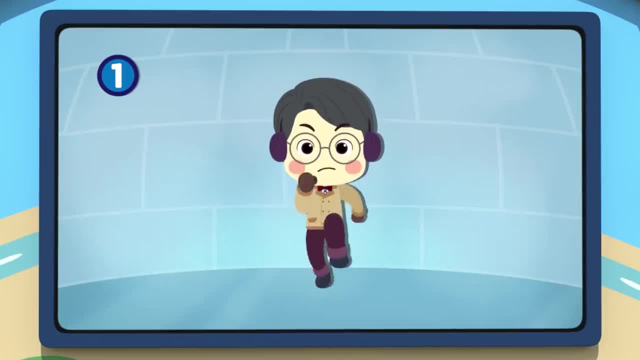 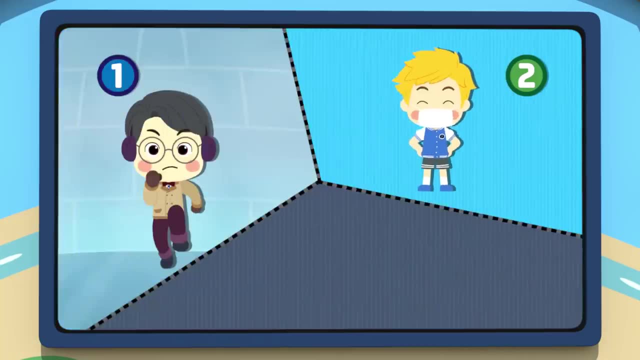 if you're outside in extremely strong winds, Should you: one, move your body to keep your blood flowing? Two, wear a mask to help prevent the spread of germs? Or, three, seek shelter in the nearest building? Hmm, or ask the rescue team for help. 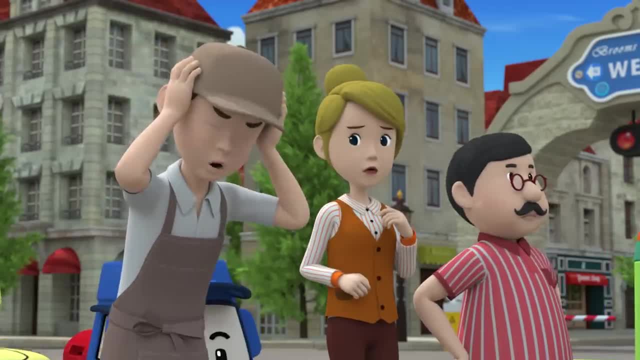 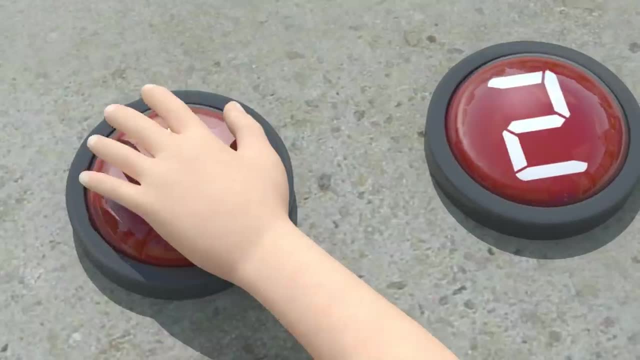 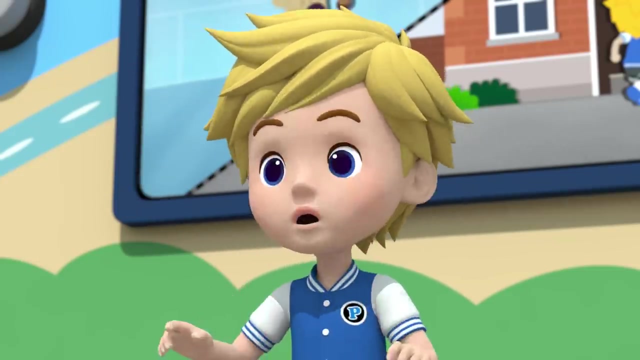 Johnny, that's not one of the options. That's a really tough one. I don't know which to pick. Is it one, is it two, or it could be three. They all seem to be right. Peter, you got this. 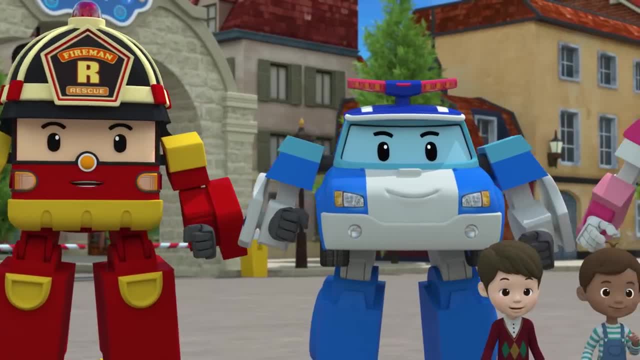 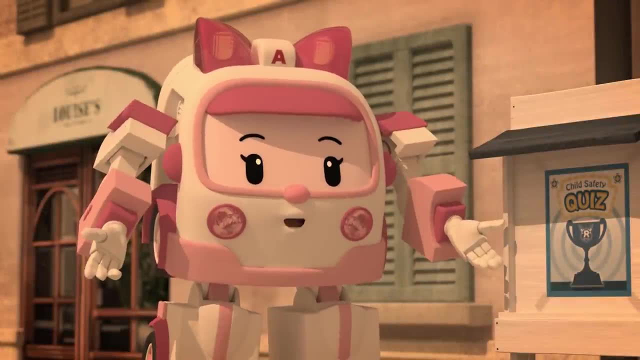 Just take your time. I know you can do it. It's the last question. We're rooting for you, Peter. you can do it. Think of all the safety lessons that you've learned and you'll do fine. Amber's right. 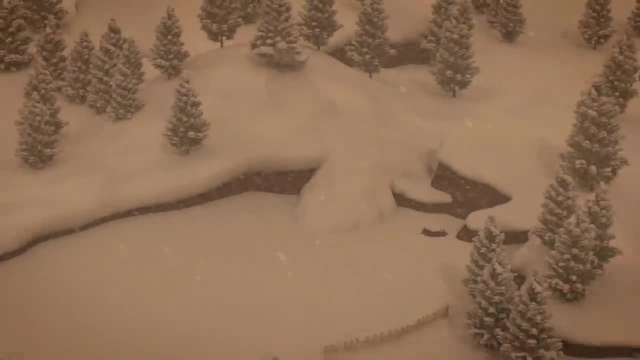 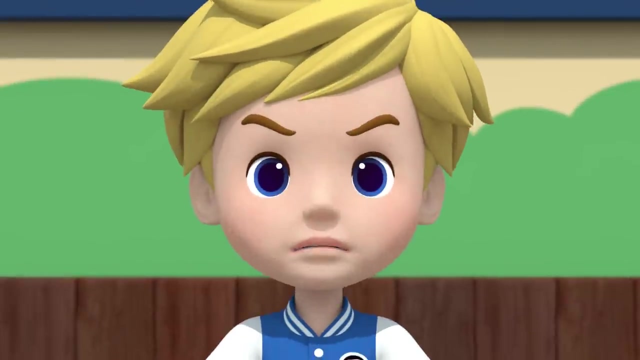 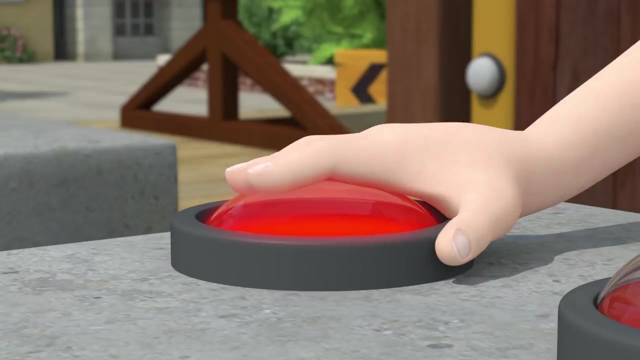 Moving your body around in cold temperatures helps keep you warm. Wearing a mask helps prevent germs from spreading around Wind: Strong winds are dangerous. If you're outside in a strong wind, you should seek shelter in the nearest building. Answer is three. 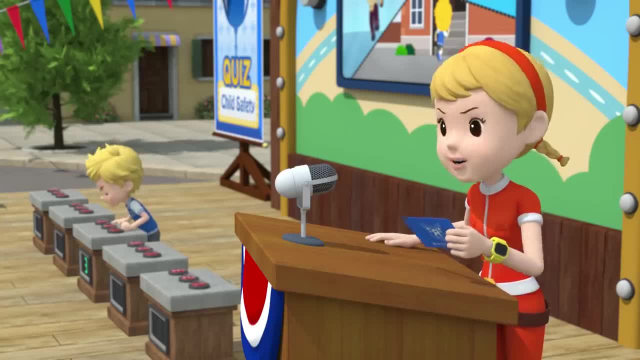 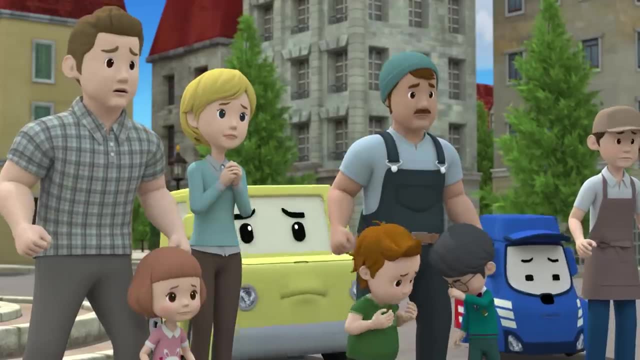 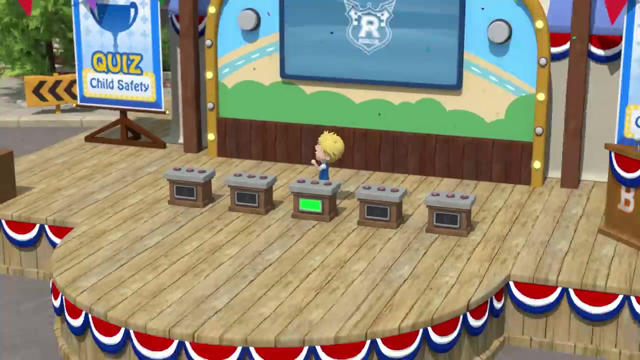 Seek shelter from the wind, find the nearest building and go inside. Is that answer correct? Please be right, I don't know. Is that the right one? I can't even look And the answer is three. I did it. Peter is our safety quiz champion. 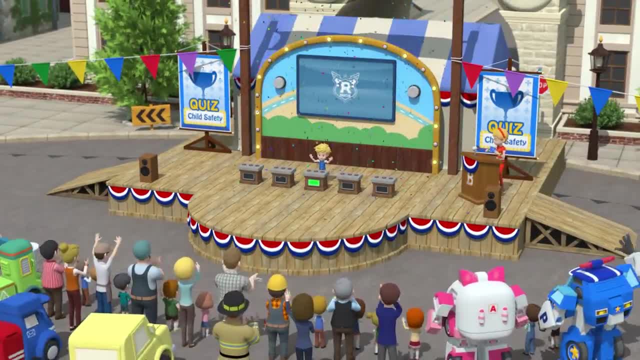 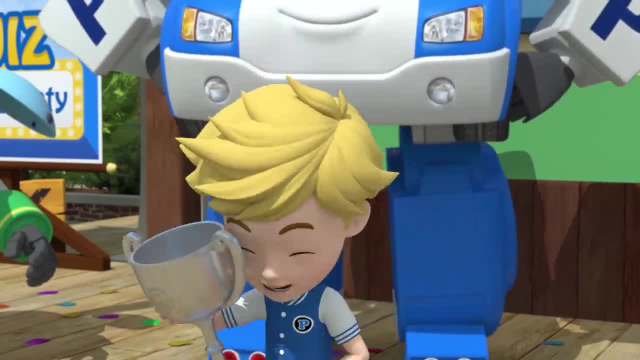 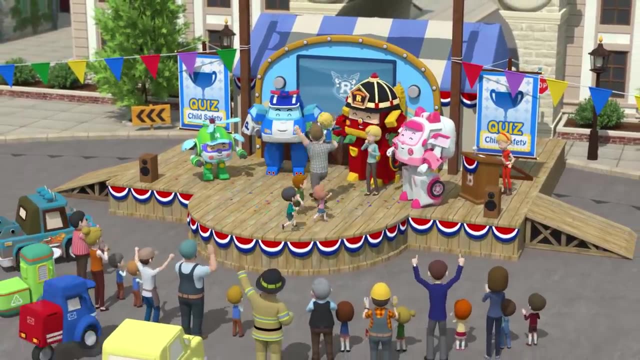 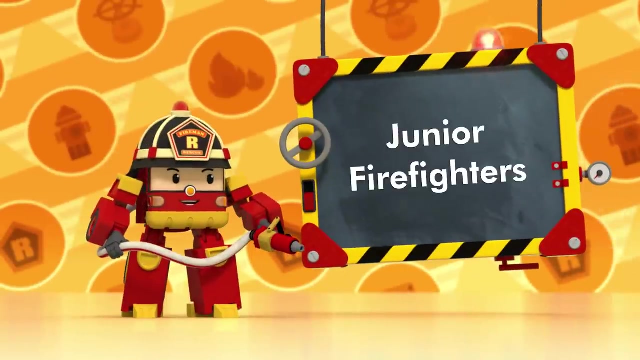 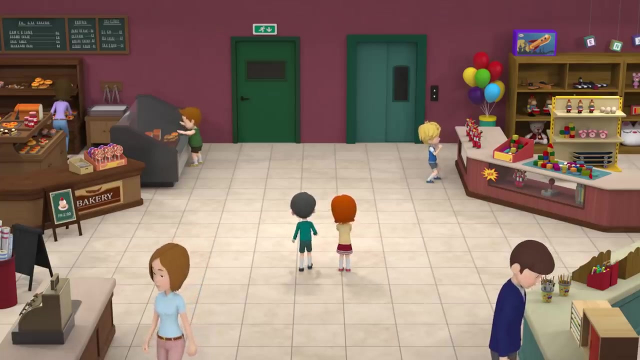 Yeah, Yeah. Good job, Peter, congratulations. Thank you, Amber. Yahoo, I'm the safety quiz champ. I give you the champion. Junior Firefighters: Wow, They have all of the Super Dragons ever made. I want every muffin ever made. 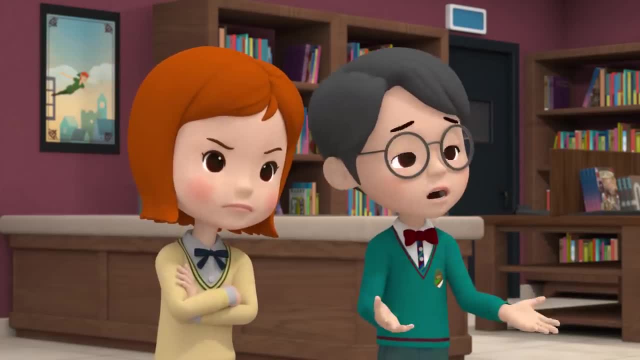 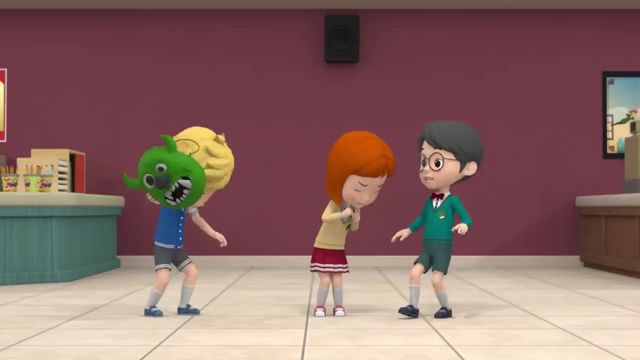 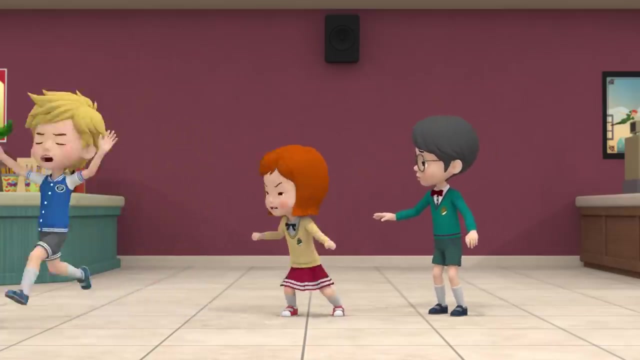 Come on, We're here to get the flowers for Parents' Day, That's right, And we have to get back. so come on. Huh, Got you guys. You were so scared. Look, Peter, You better run for your life. 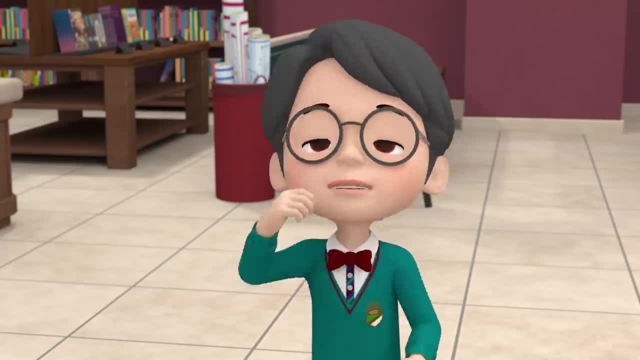 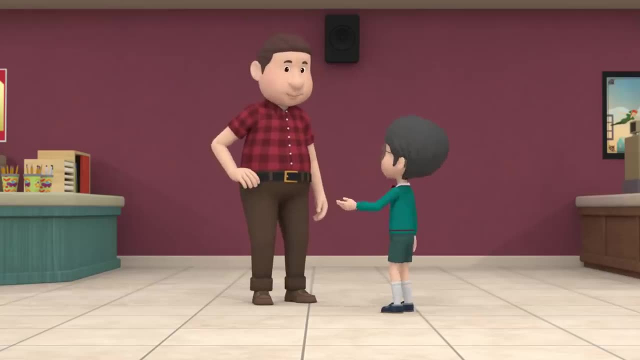 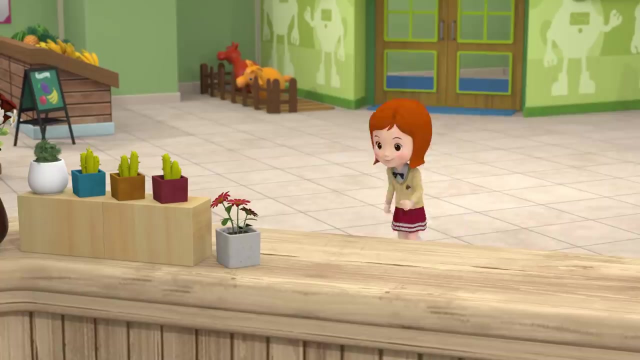 Excuse me, Could you tell me where the flower shop is? I'm pretty sure it's on the fourth floor. You can take the elevator right over there. Great, Thank you so much. Huh, There it is. Wow, They're so pretty. 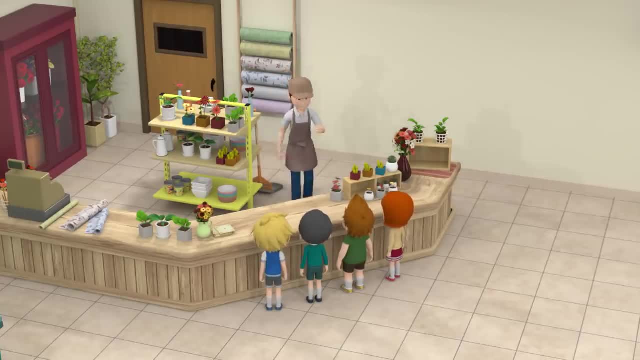 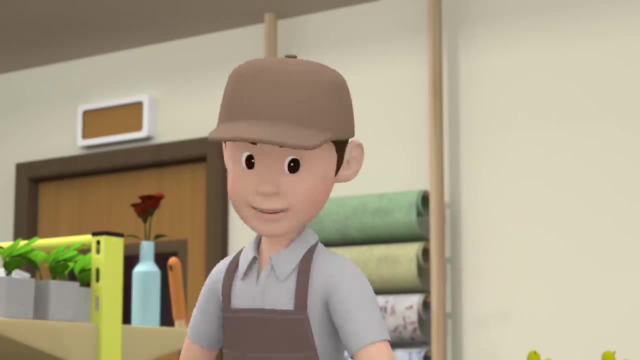 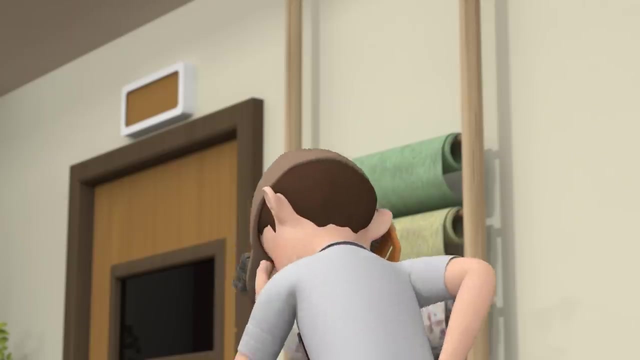 Hey there, kids, What can I help you with? Mister, do you sell carnations here? Aha, I'm guessing you need them for Parents' Day? Wait right there, Huh, Oh no, Are you alright, I'm fine, I'm fine. 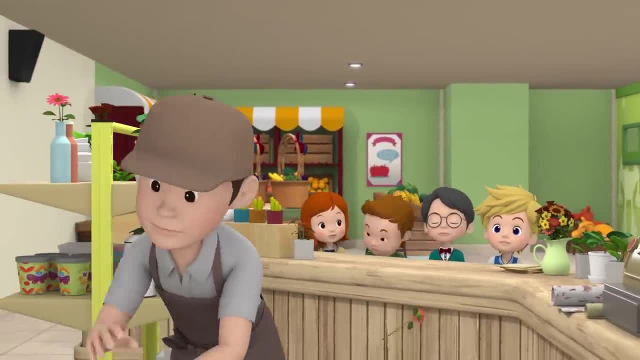 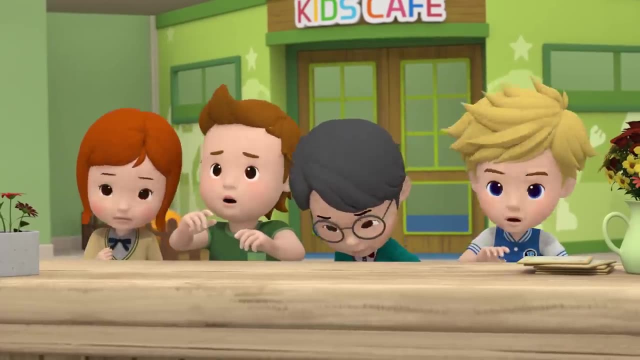 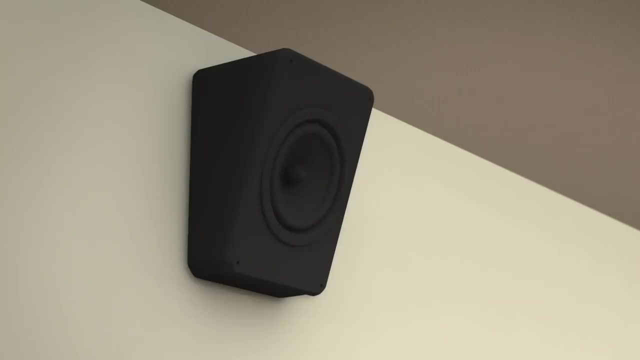 That's a rose, That's not. it, Not that one. Here we go Way in the back A bunch of Huh. What Sir? That's the fire alarm, What A fire. Attention shoppers Due to a safety concern. 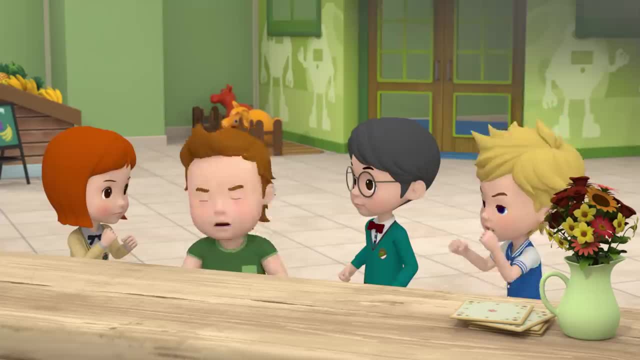 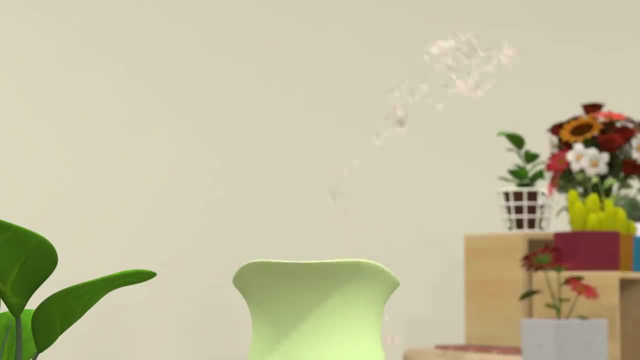 we will immediately evacuate the building using the closest emergency exit. Our exit's by the elevator. Attention shoppers: Please consult a member of the shopping. The smoke's starting to come in. if you need help exiting the building Here guys. 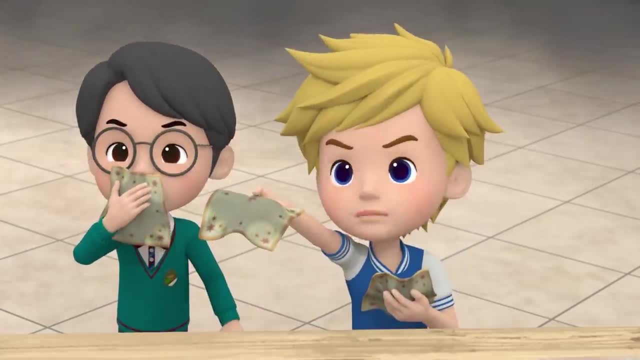 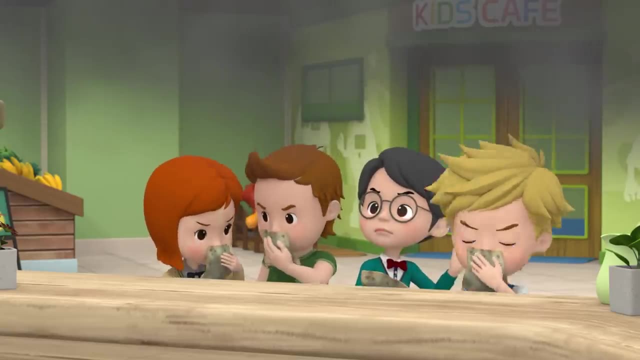 Here. Use this to cover your nose and mouth so you don't breathe in any smoke. Thanks a lot. Hold on My bag. No, wait, Don't worry about your bag, I have to go now. Okay, go, I'm behind you. 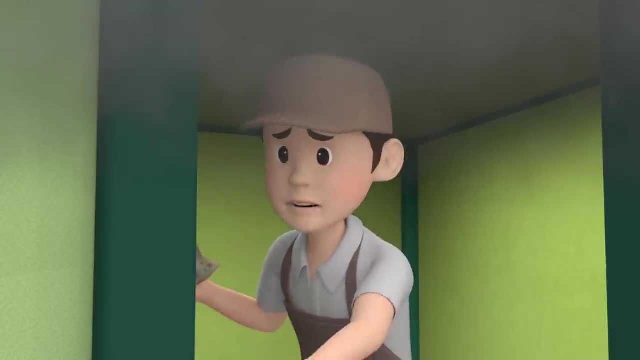 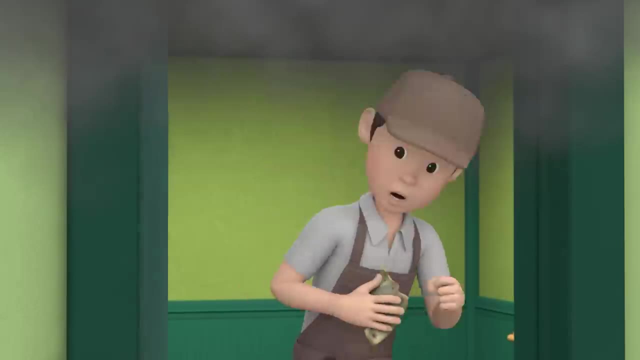 I can't get this to open. Come on, We'll take the elevator. Huh, No way. If we take the elevator and the power goes out, we'll all be trapped in there. What? Oh? thanks for letting me know about that. 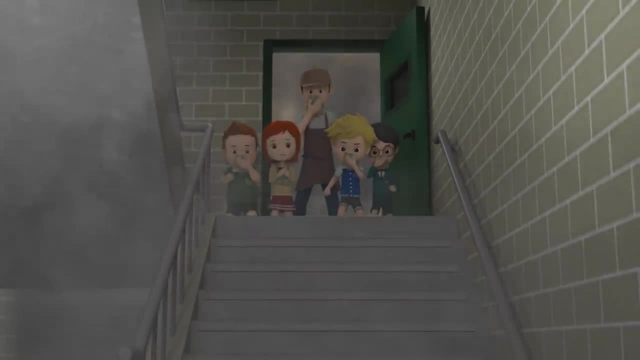 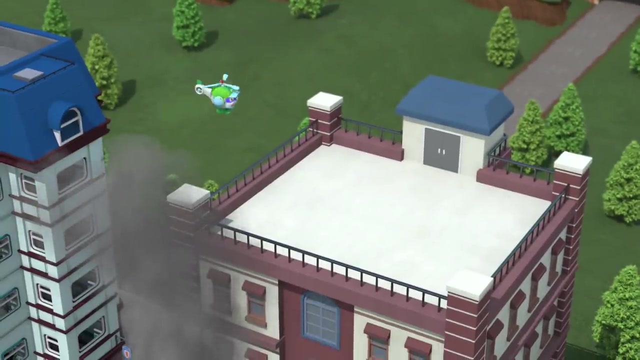 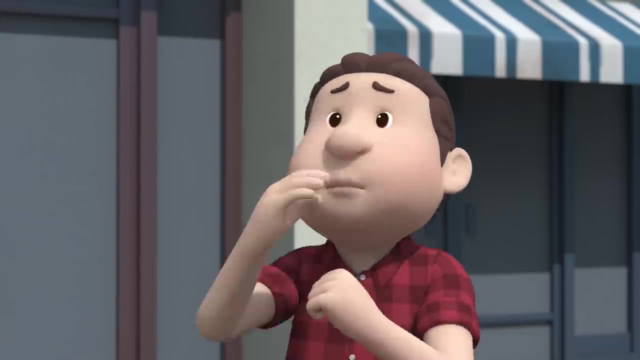 We can't take the stairs with all that smoke down there. Then we're gonna have to go back and look for some help. Everyone get somewhere safe. Roy. Some kids were in there. I don't know if they got out in time. 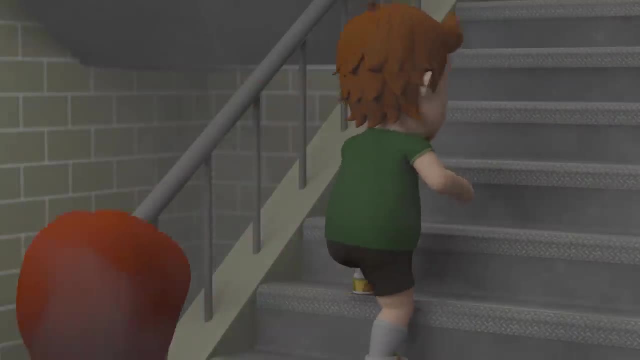 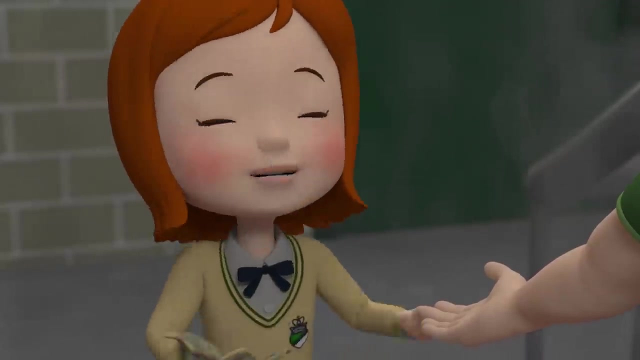 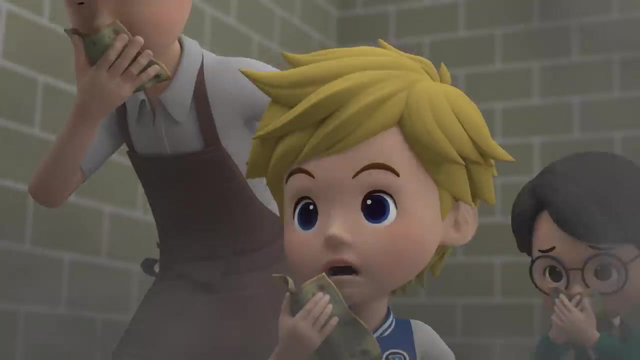 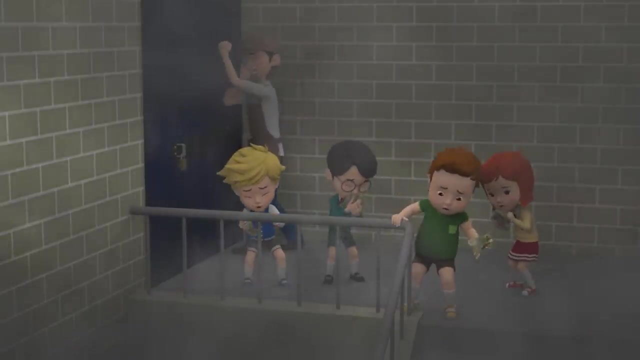 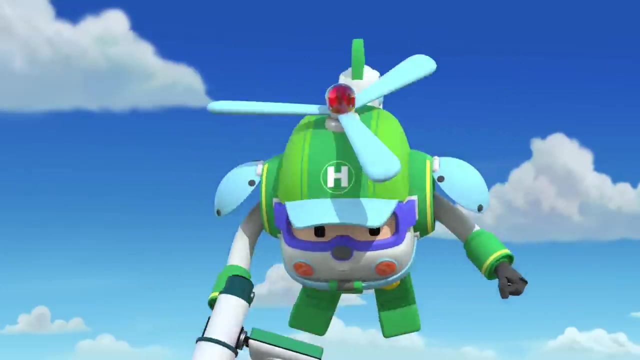 Kids. Just take my hand, Cindy, Okay, Johnny, Huh. Guys, the door is locked. Now the smoke is coming up on the landing. Please, somebody help us. Please help us. Huh, Roy, I found the kids. 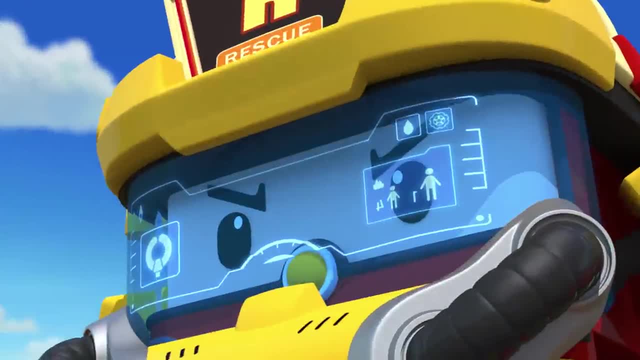 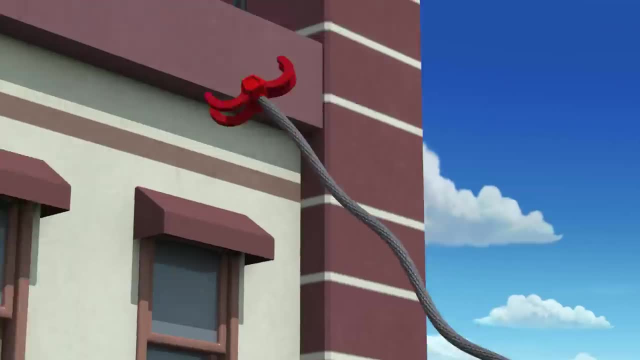 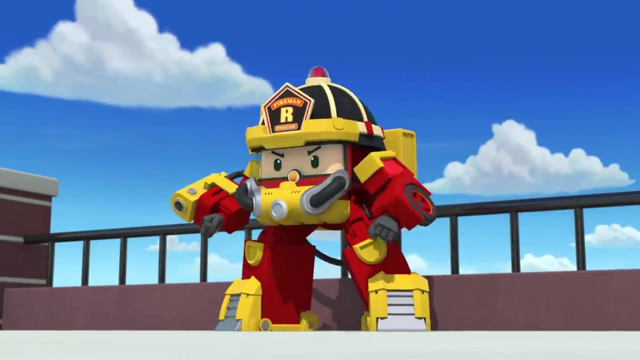 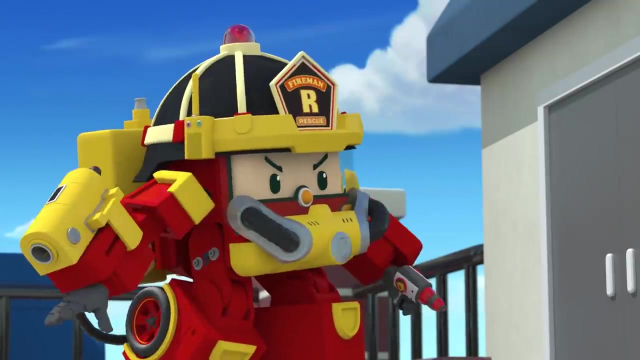 They're in the north stairwell. Good work, Heli. I'm going in. Hmph, Hmph, Hmph, Hmph, Hmph, Hmph, Hmph Kids Guys, I hear Roy, Roy, I'll get you out, Just step back. 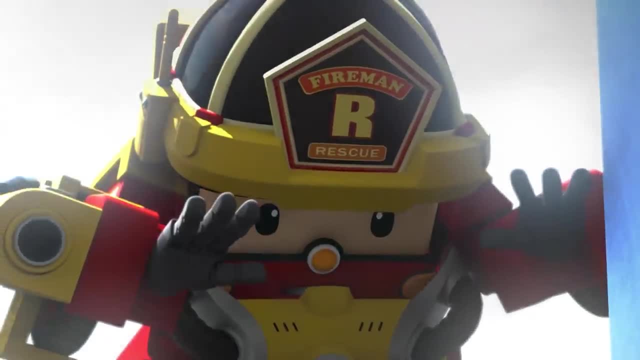 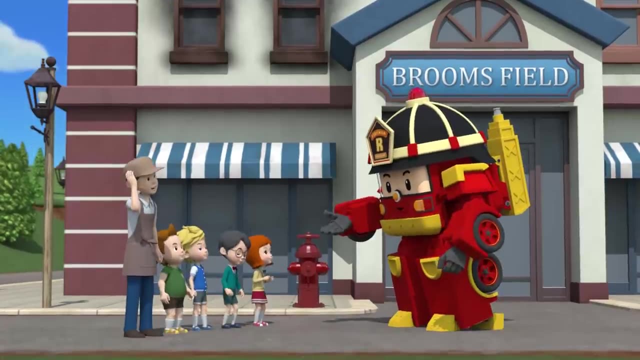 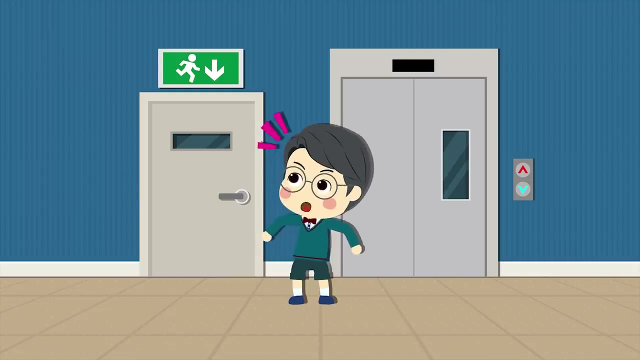 Okay, Here goes Hmph. Is everyone alright? Yeah, Roy, You did what you were supposed to do. You handled that exactly right. Since you never know when a dangerous situation might happen, you should always know where the emergency exits are. 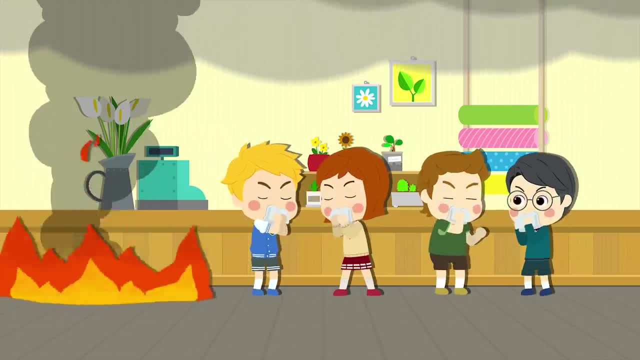 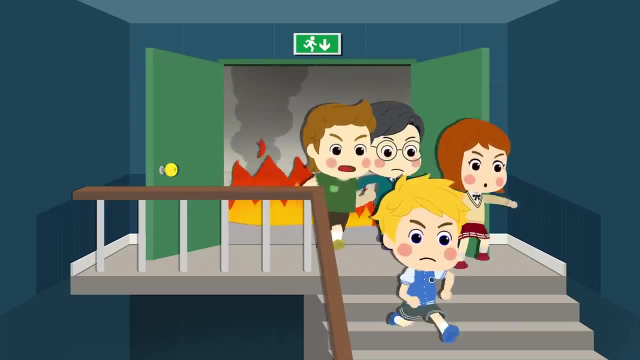 If a fire does break out, cover your nose and mouth, stay close to the ground and get away. Elevators will not work if the power goes out, so use the nearest stairway instead. If you're on a lower floor, go right outside. 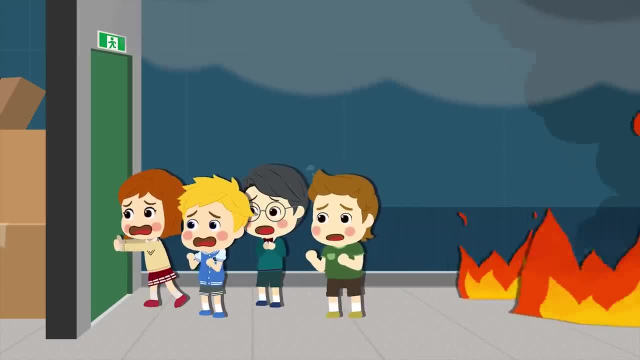 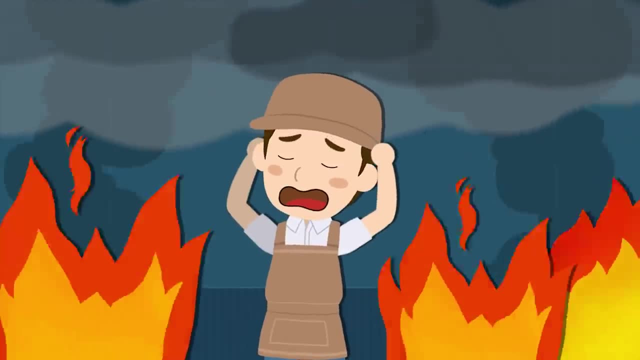 If you're on an upper floor, exit to the roof, Never lock stairwell doors or store items against them. And, most importantly, stay calm and try not to panic. Thinking's the key. Stay calm and try not to panic. Stay calm and try not to panic. 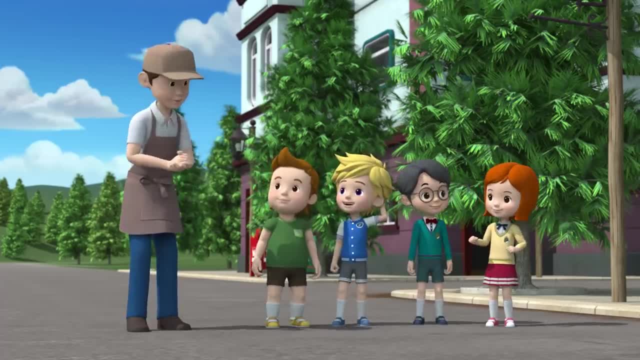 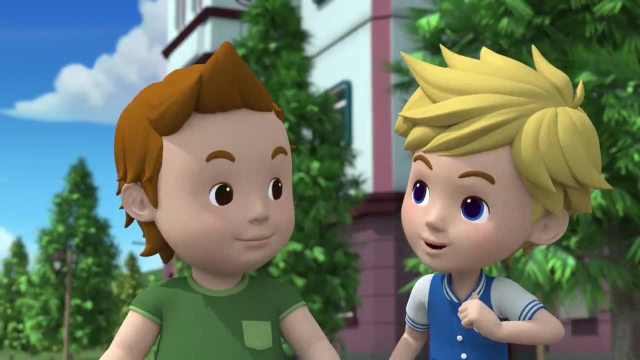 Oh man, I didn't handle that situation well. Thank you, kids for everything. No, it's all good. We've just been through fire safety. training is all. You're looking at an honorary firefighter right here. You're looking at an honorary firefighter right here. 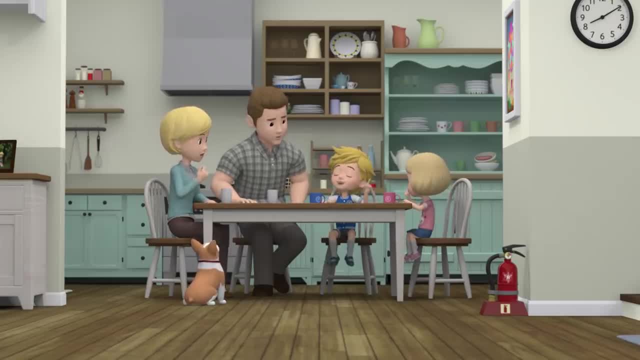 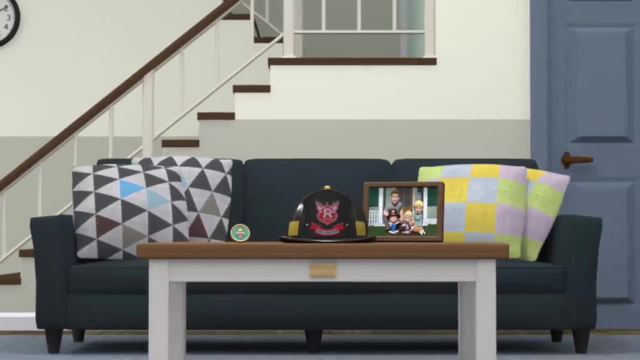 Then the smoke started coming and I let everyone out of the store. Way to go. I'm proud of you. Wow, Peter, you're like a real firefighter. Wow, Peter, you're like a real firefighter. Wow Peter, you're like a real firefighter. 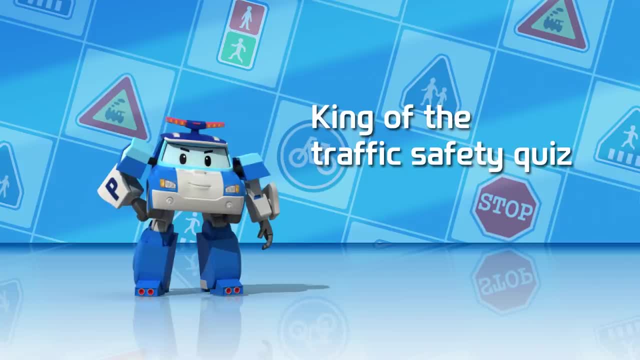 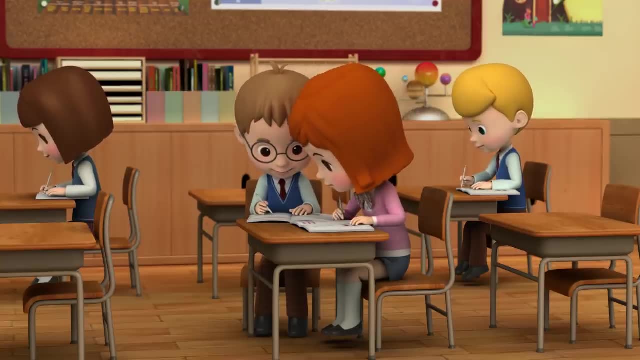 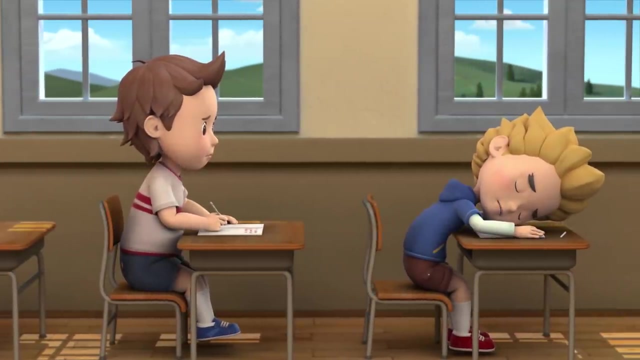 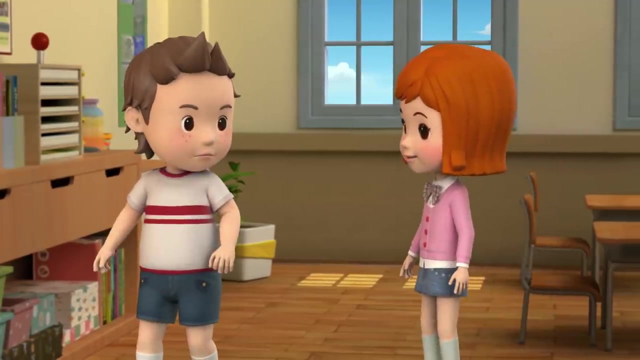 King of the Tropic Safety Quiz. To solve this, you just do that. Ah, Like that, That's it. I give up. Huh, They're having a traffic safety quiz. They're having a traffic safety quiz. Are you going to enter it, Doug? 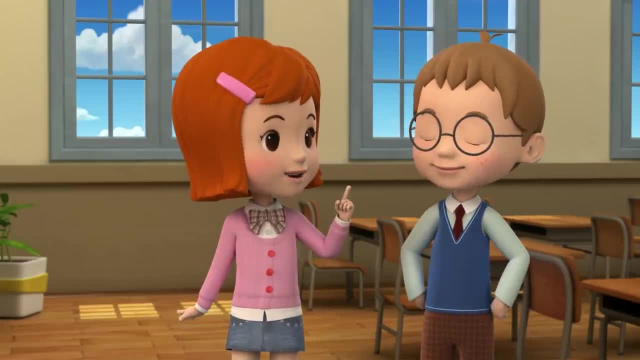 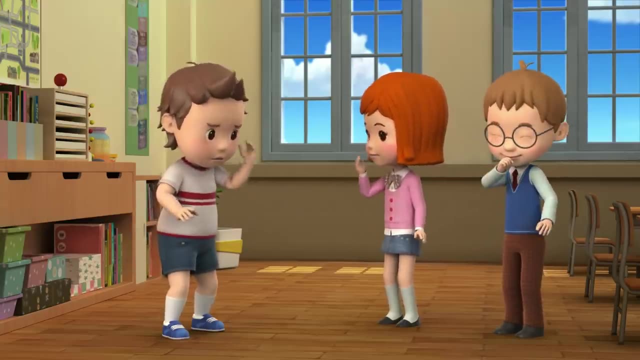 Yeah, uh-huh, Awesome. Tim and Toby are going to enter as a team, Are you? Uh, I'm with Kevin, Kevin and you. Good luck, I've got a feeling that you'll need it. Good luck, I've got a feeling that you'll need it. 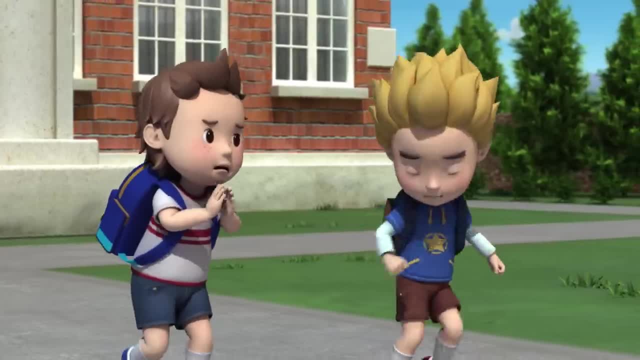 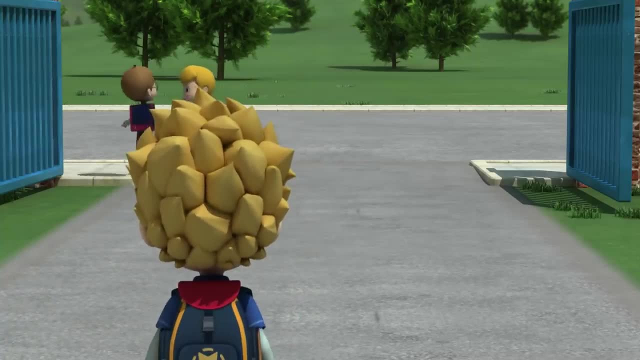 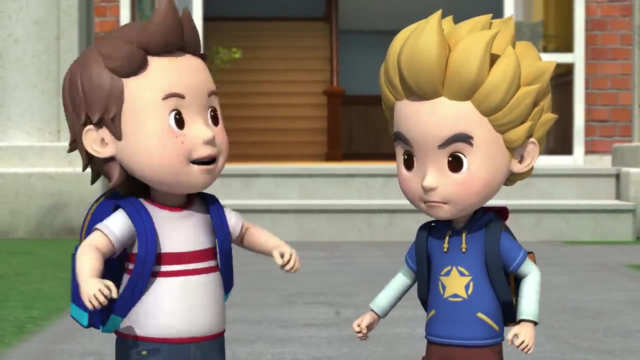 Kevin, do the quiz with me Please. I'm not here to take a quiz, Kevin, Are they really entering? Yeah, somebody's got to win last place. Yeah, somebody's got to win last place. I'm in Huh. 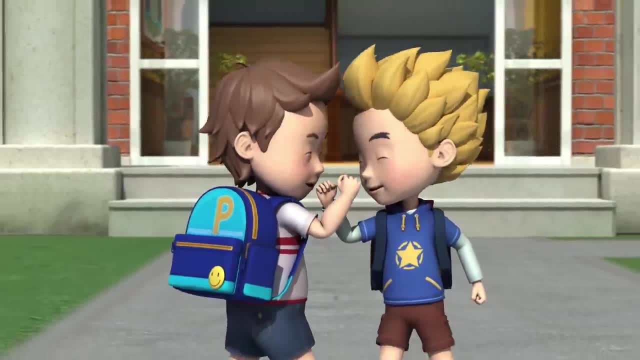 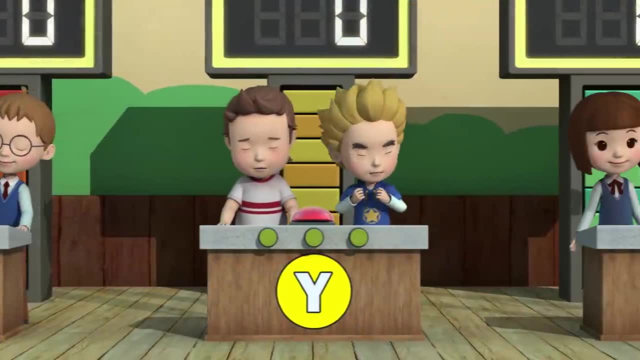 The Traffic Safety Quiz, Kevin, And we're going to win it. Oh yeah, Good afternoon, lovely citizens of Poomstown. We will now begin the Children's Traffic Safety Quiz competition. We will now begin the Children's Traffic Safety Quiz competition. 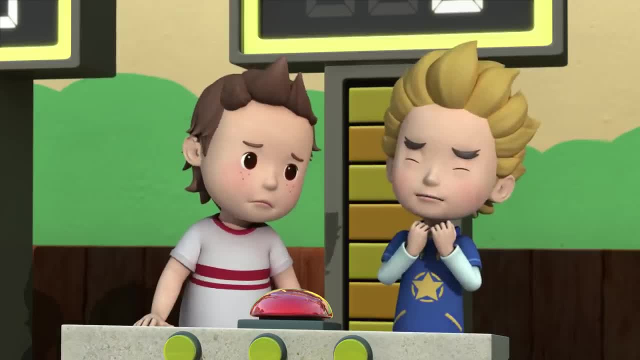 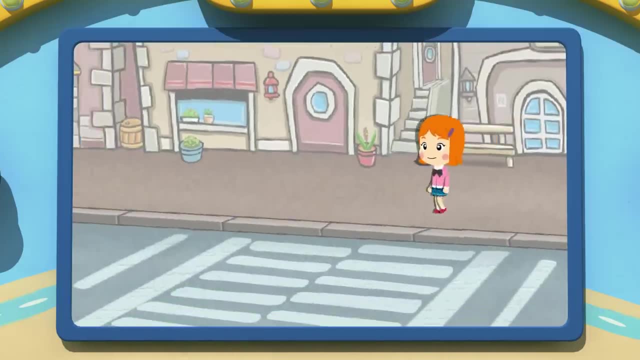 What Shaking am I? Yeah, Whoa, I'm nervous. And now here's question number one: How do you safely cross at a crosswalk? How do you safely cross at a crosswalk which does not have a signal? 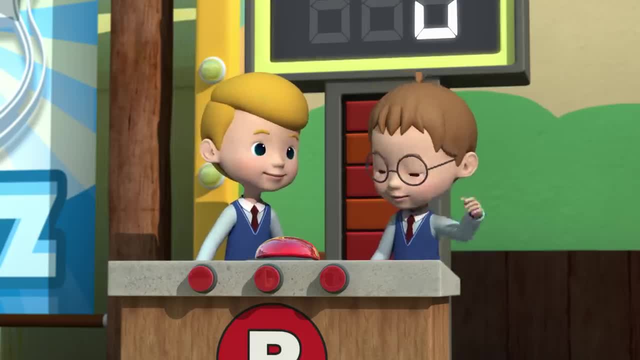 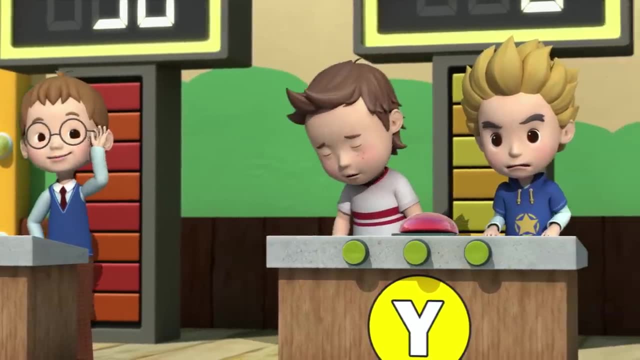 Answer: You check to see if there are any cars coming. you wait for them to stop, then raise your hand and cross. Yes, That is correct. The red team now has 50 points. Okay, The next question is If you are on a bicycle. 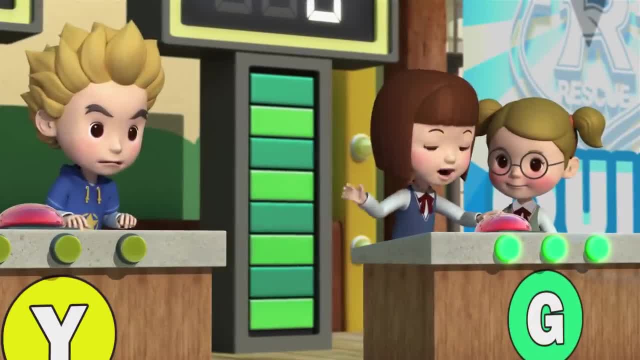 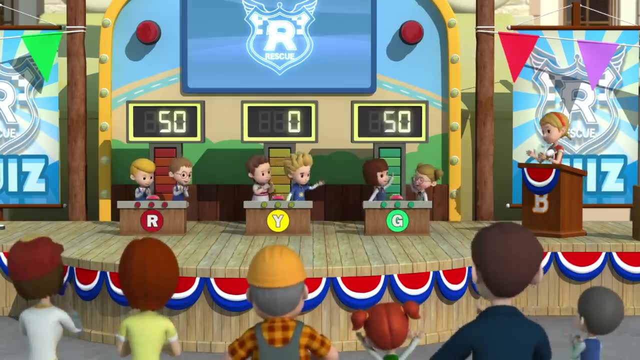 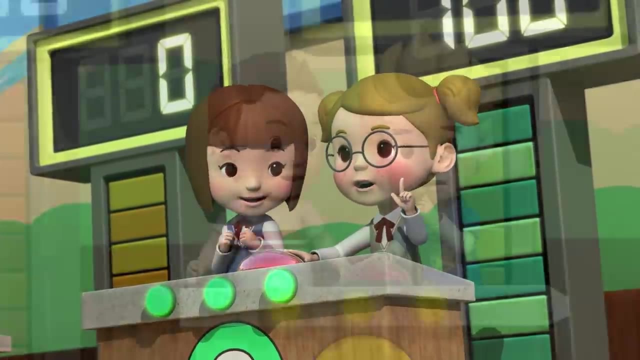 and you want to cross the road. what do you do? You get off your bicycle and you push it across the street. Green team. Correct Cars can't stop right away because it takes them some distance to brake. You must always wear a seatbelt. 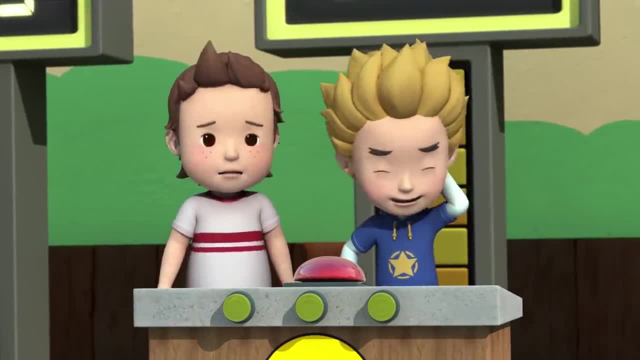 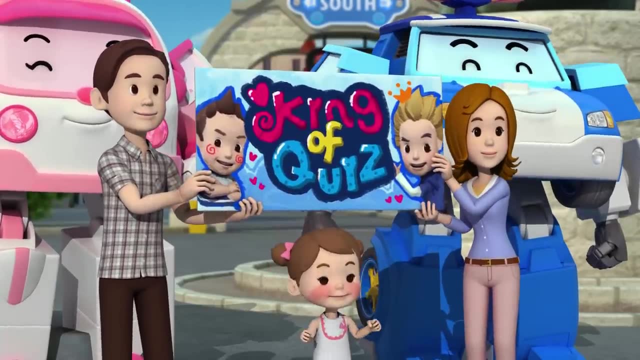 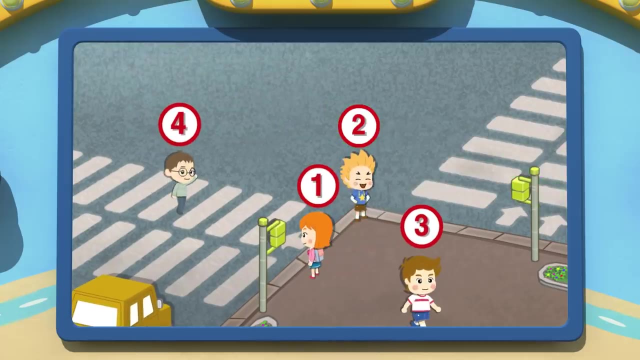 every time that you ride in a car. I pushed a button by mistake, Kevin Doug. Come on, Come on, guys. Next question: Who is in the most dangerous situation? Answer: Four: Wrong, I'm sorry. Yes. 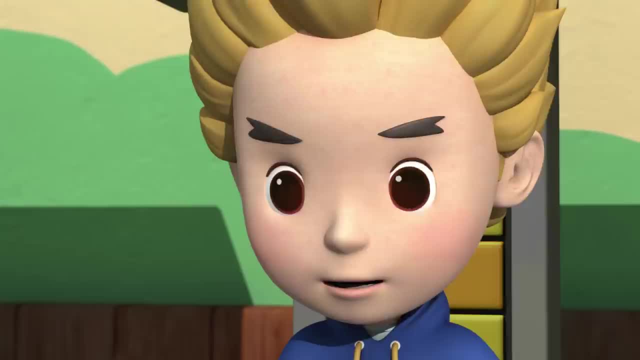 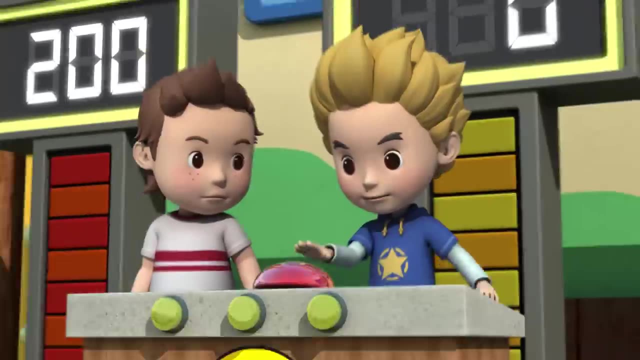 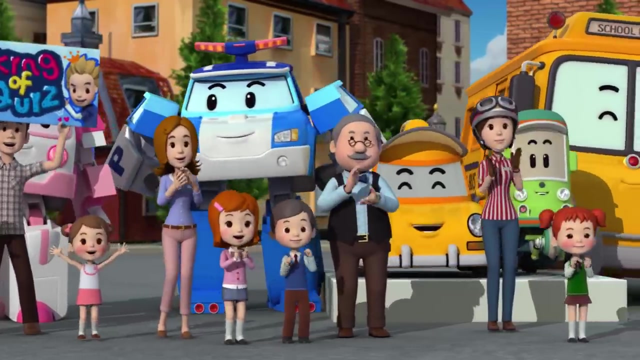 Yellow team. No, That's right. I remember Polly rescuing me when I was at the corner of the street. Yes, The answer is number two. The corner is most dangerous, That's right. Yellow team now has 50 points. 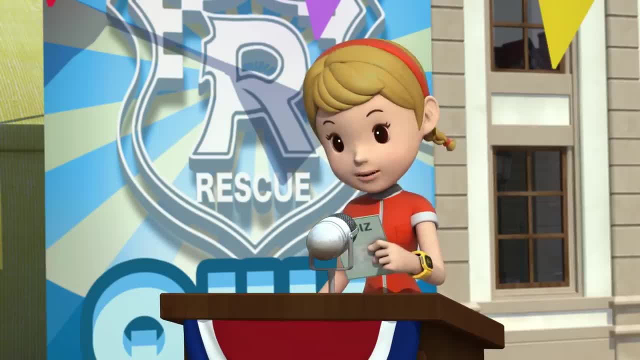 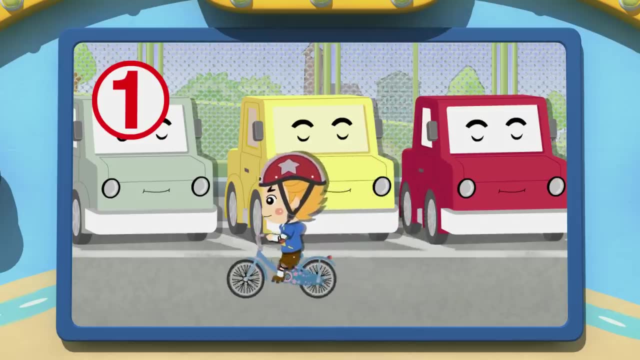 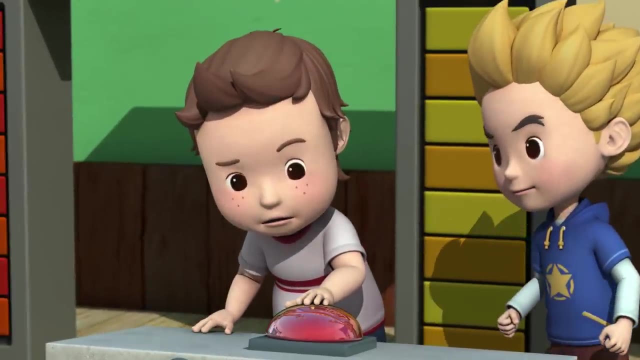 Now the next question: Where is the proper place to ride your scooter or inline skates? 1. The parking lot, 2. An alley. 3. A construction site. 4. The playground. Yes, yellow team, Can they get this one right? 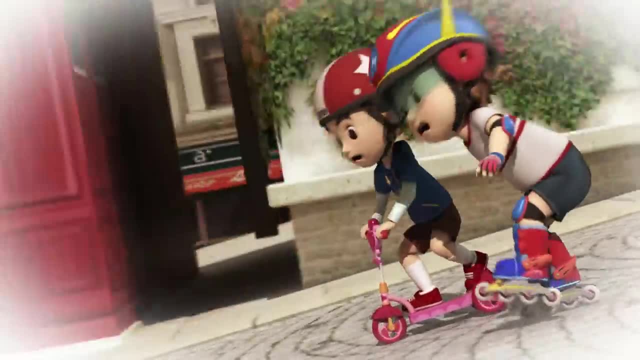 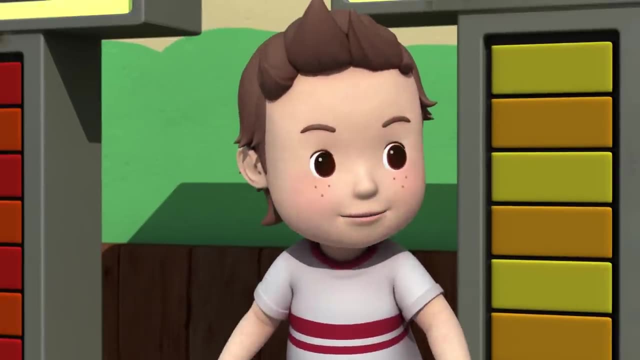 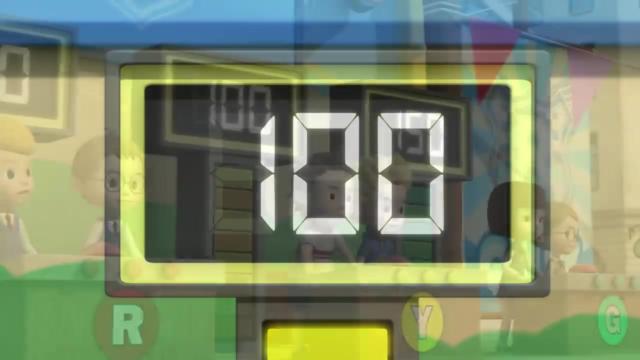 I remember Even an alley or side street with less cars on it can be dangerous Because there are no cars. Answer: Playground, Because there are no cars there. That is correct. Okay, Here comes the next question: When it snows? 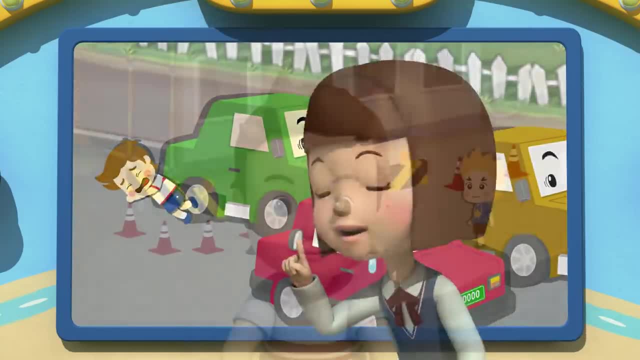 Don't wear white clothes and keep your hands out of your pockets, You are 18 times more likely to get into an accident. so don't do it. Avoid the road in front of the construction site and take the other route. Wow, It's a very close game. 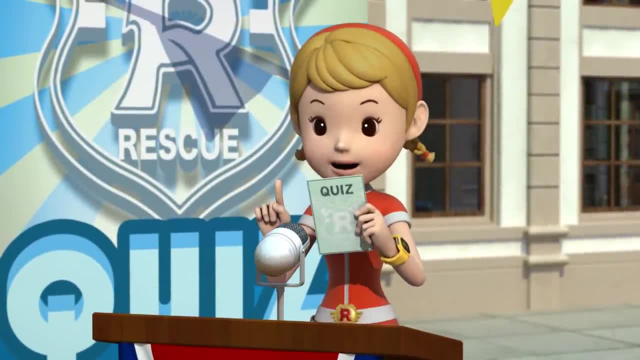 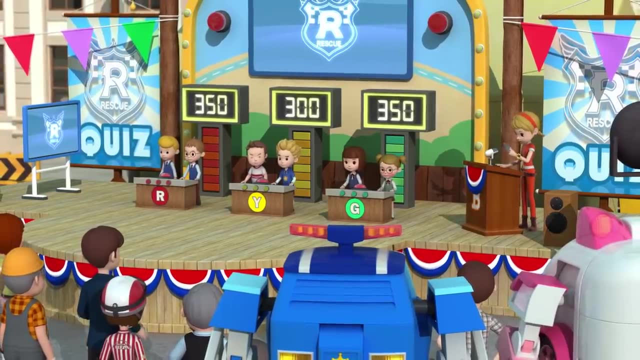 And now it's time for the final question. And now it's time for the final question. This question is worth 100 points. Whoever gets this question will be the winner. Whoever gets this question will be the winner. What are the three most important things? 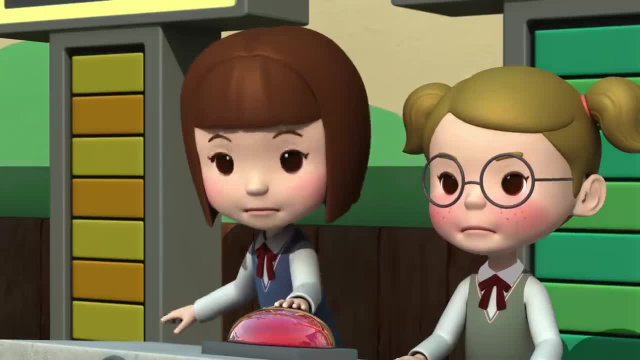 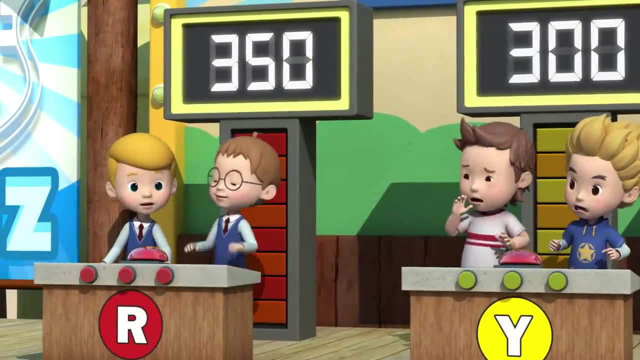 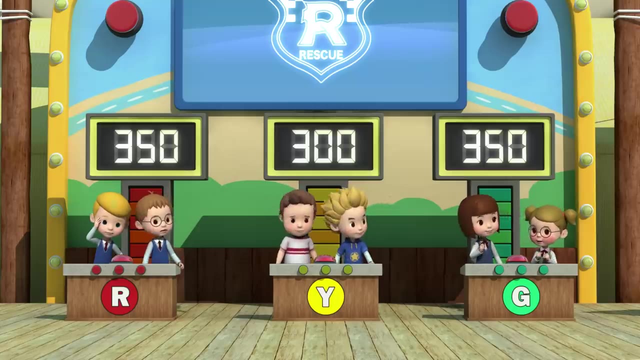 you should know, in order to avoid car accidents. you should know, in order to avoid car accidents: Yes, green team. Okay, the red team has a chance now, When you're crossing at the crosswalk and the green light is flashing, Oh, no. 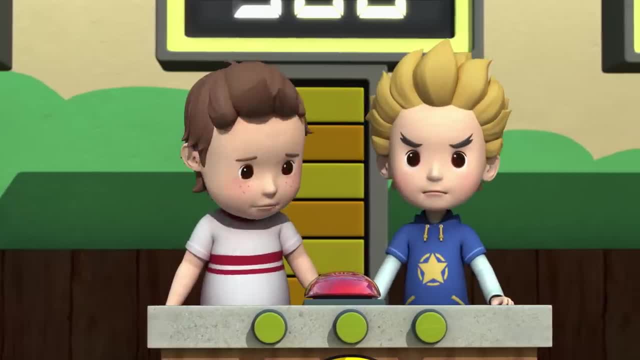 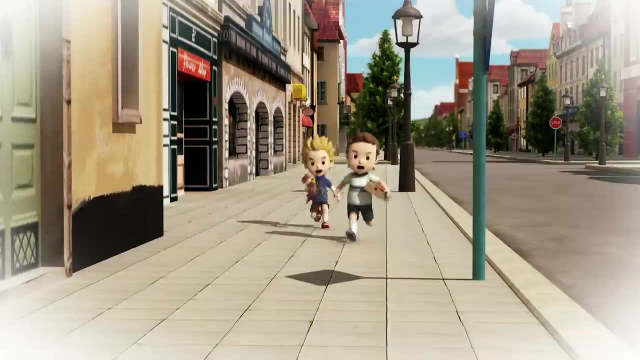 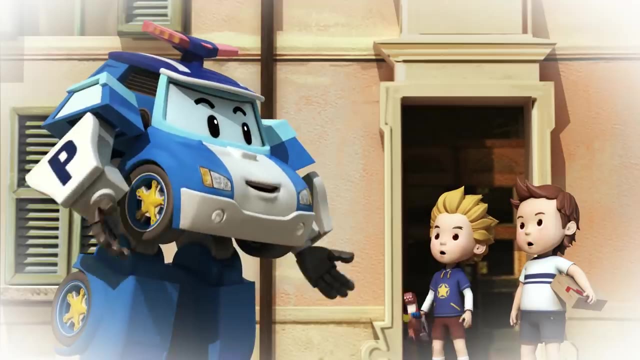 That is not a correct answer. The yellow team has a chance. Kevin, Doug, Good luck, That's right. Remember we were running to Jenny's house? We almost got into an accident while crossing the road, Yeah, And then Polly taught us what to do. 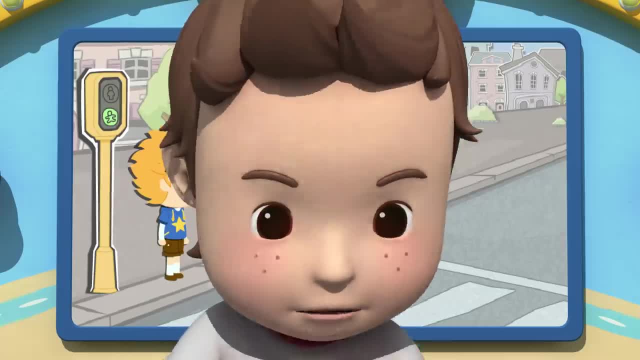 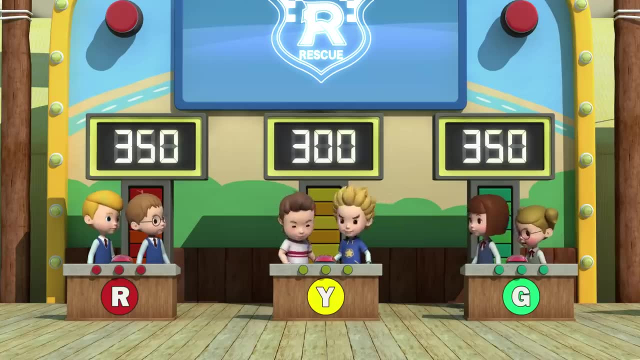 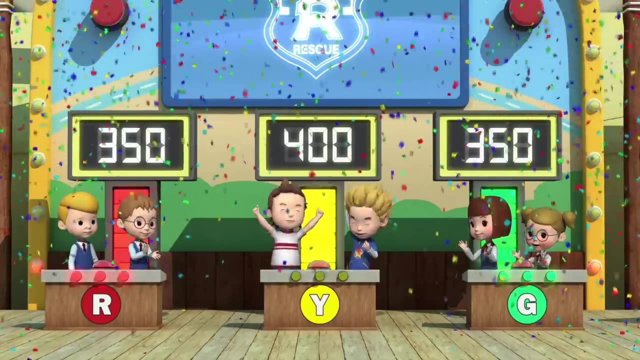 Number one: Get in the habit of stopping. Number two: Make eye contact with drivers. And three, Always keep your eyes on the car while you're crossing. Congratulations, Oh, you're so proud of me. We won. Yeah, We did it. 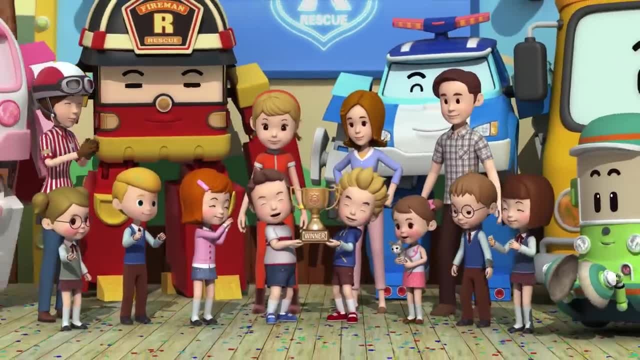 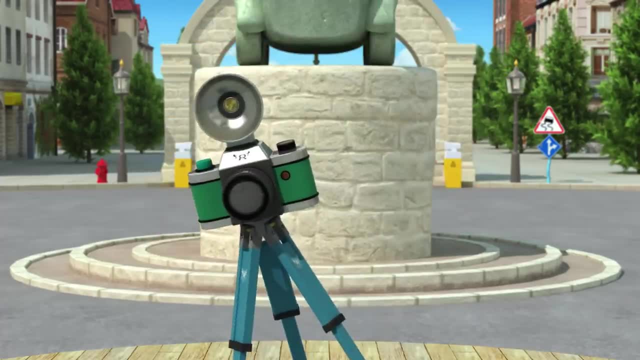 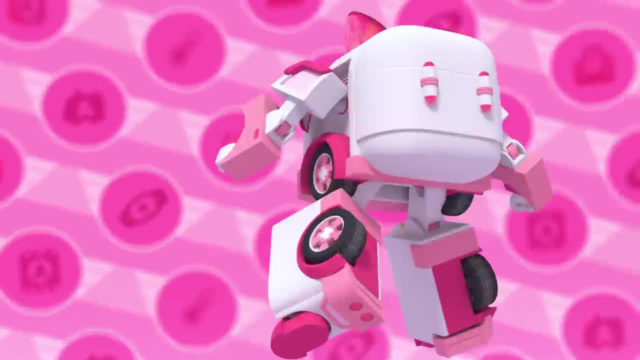 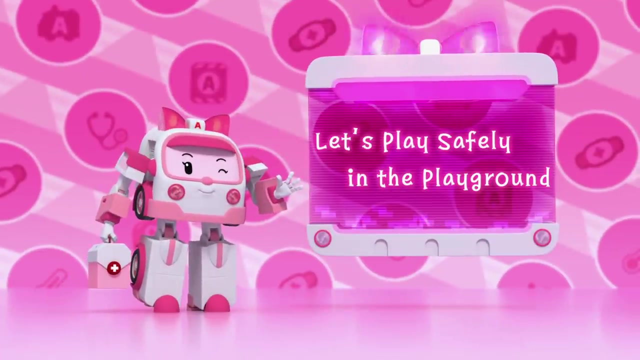 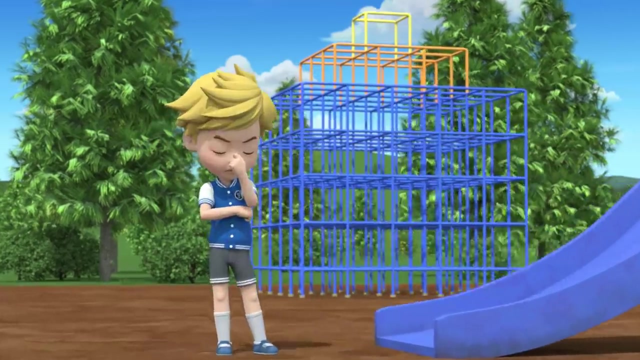 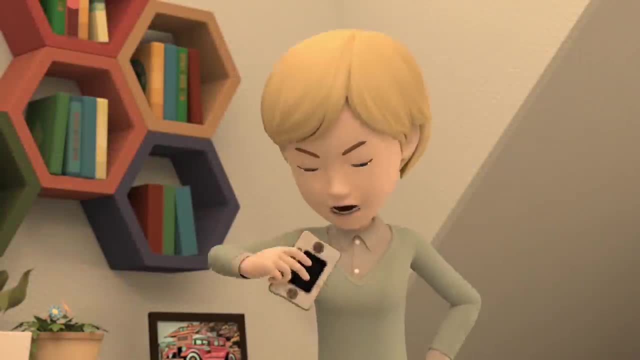 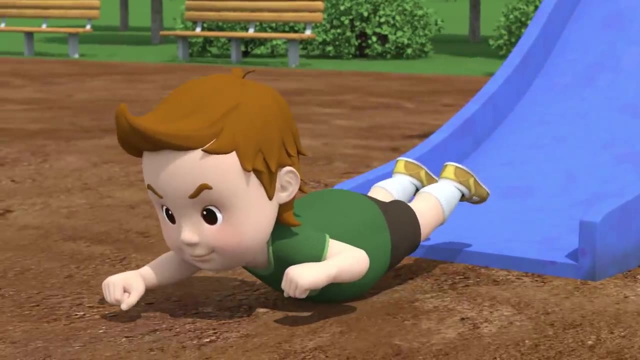 You get the game machine back after you watch your sister. You get the game machine back after you watch your sister, Super Dragon. Yeah, Wasn't that pretty sweet? Wasn't that pretty sweet, Mm-hmm, Super Dragon. 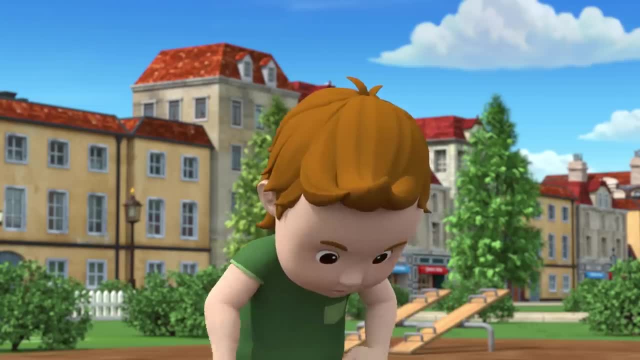 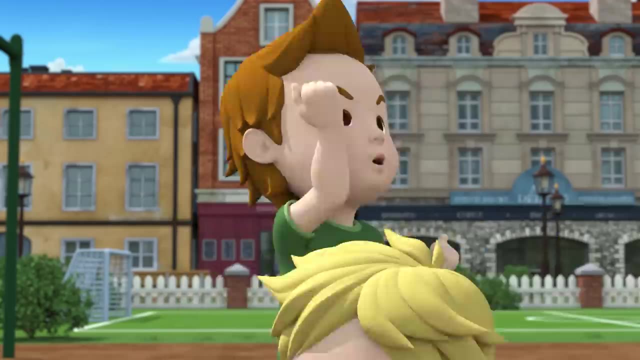 Lucy, you can't slide head first. Yeah, only a Playground Master can slide like that. Playground Master- What's that? A Playground Master is brave and fearless And awesome and wise. Playground Masters are heroes that have mastered every single Playground skill. 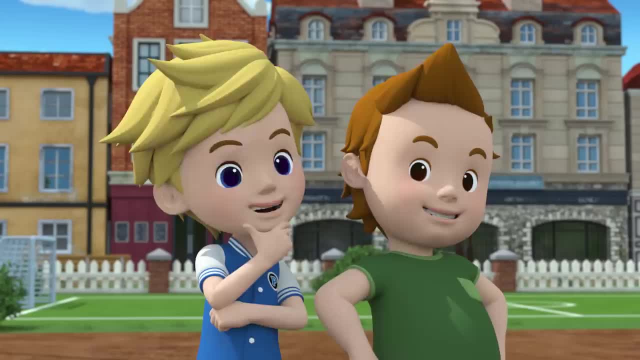 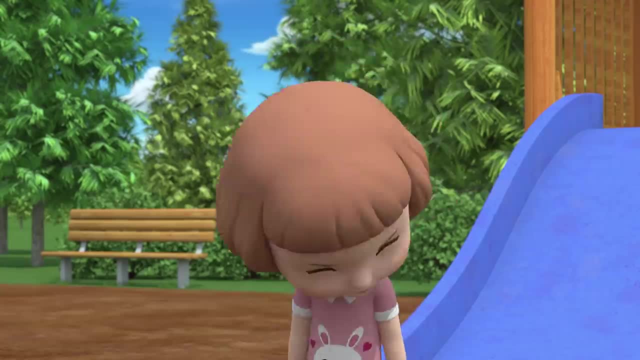 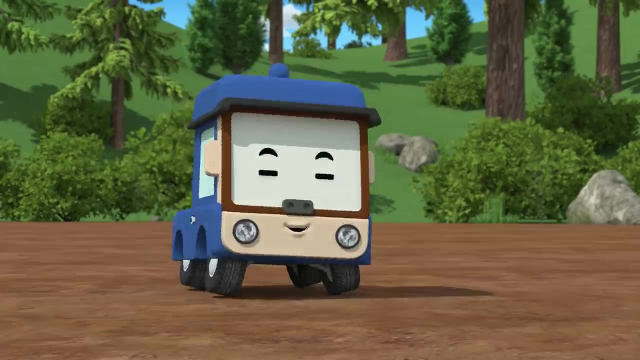 Heroes like us. I wanna be a brave Playground Master. Uh fine, If you promise to follow all our commands, we'll give you some training. Yep, I'll do what you say, Captain Yay Woo Ta-da. 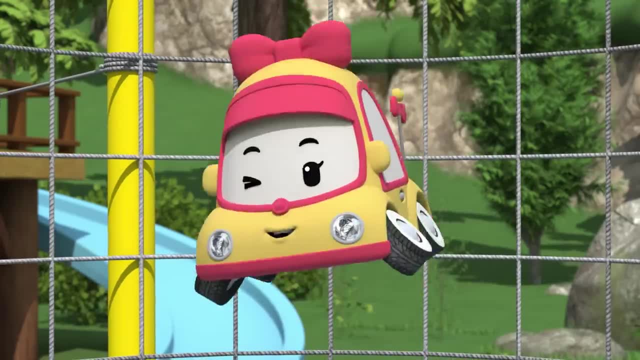 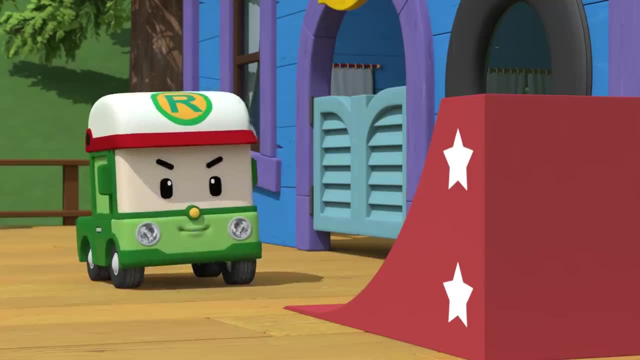 Wow, you're the best. It's amazing, right? Not everyone can bounce like this, you know, Hey guys, Uh-huh, Rudy, what's up? The trampoline is way more fun if you do a super high jump. 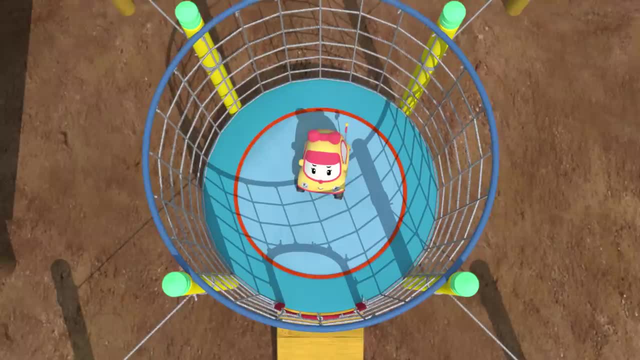 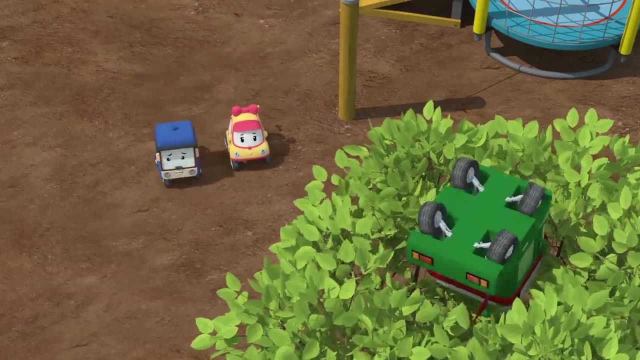 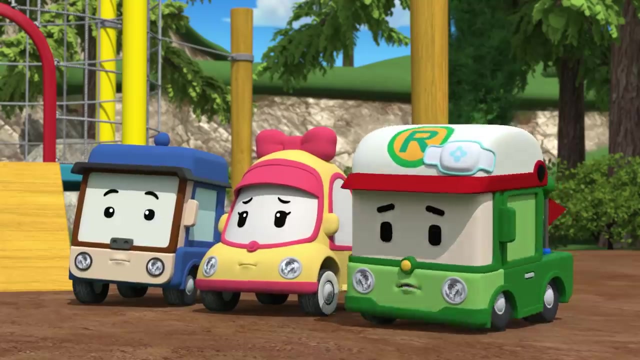 Ready set go. No, Whoa, Whoa, Rudy, Ugh, Ugh, Guys, help me. Uh no, Oh, Rudy, that was quite a dangerous thing to do. I'm sorry, Roy, I just thought it would be fun and awesome. 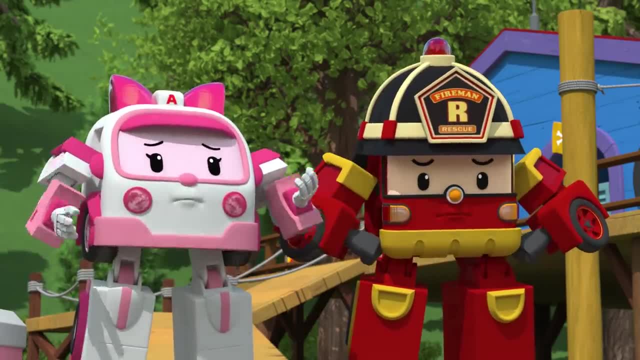 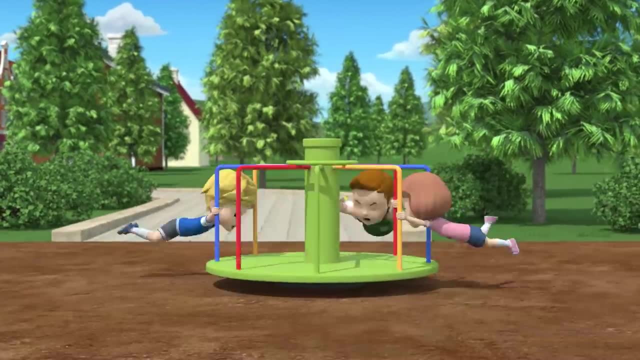 Children. trampolines are fun, but you should never jump too high or try to do dangerous tricks. okay, Yes, we promise we'll remember. Ah, Ah, Ah, Hold on tight. We're in a grueling test of will. 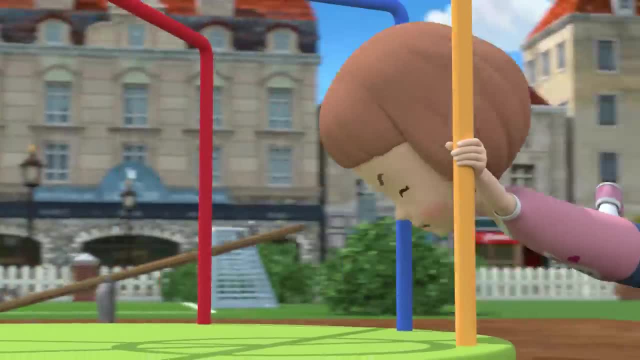 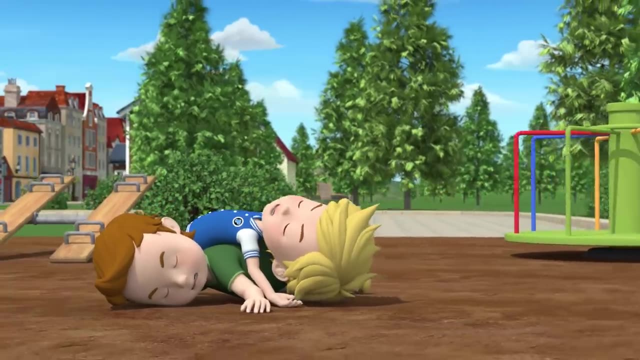 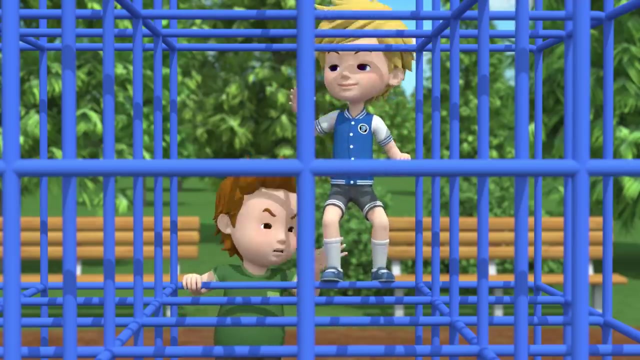 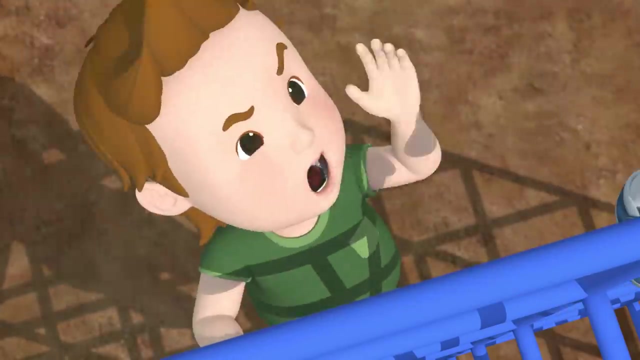 Yes, sir, Captain, Ah, John, no, no, Ah, Ah, Captain, I'm gonna beat you to the top. No, you aren't, I'll beat you. How do you like this? Oh, come on, Peter. 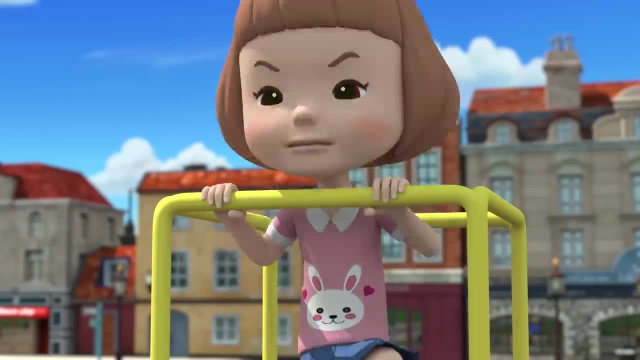 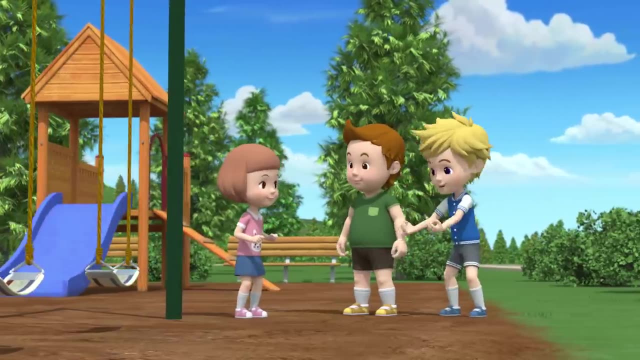 Ah, Victory is at hand. Ah, Ta-da Made it to the top. Captain, Whoa Huh, Lucy, you passed the training with a perfect score. He's right, You were just awesome. You're a Playground Master, It's official. 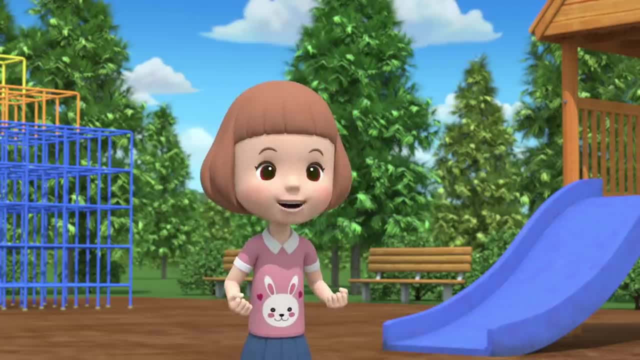 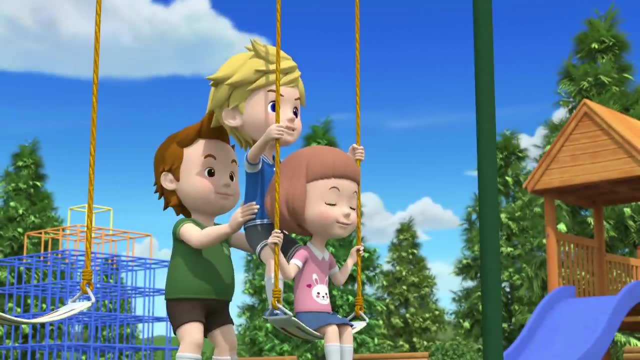 Great job, Lucy. Woo-hoo, I'm a Playground Master And now I can tell you about the secret game I invented. I call it the Big Swing. Let's fly. Ah, Woo-hoo, Whoa, Ha-ha-ha-ha. 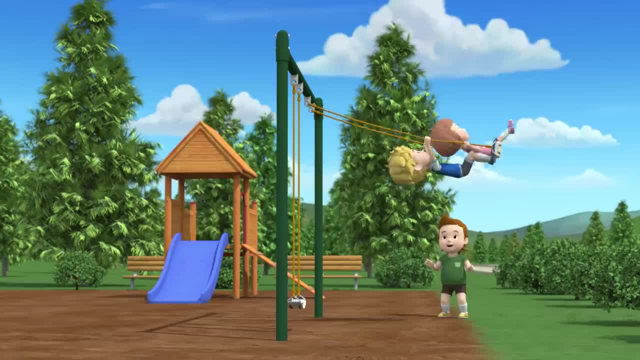 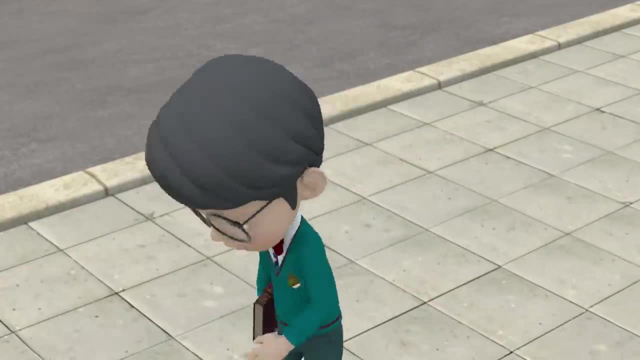 We're really high. Ha-ha-ha-ha, Right, So much fun. Ha-ha-ha-ha, Woo-hoo, Whoa, Hey, look, it's Charles. Hey, Charles, Huh, Hey there. 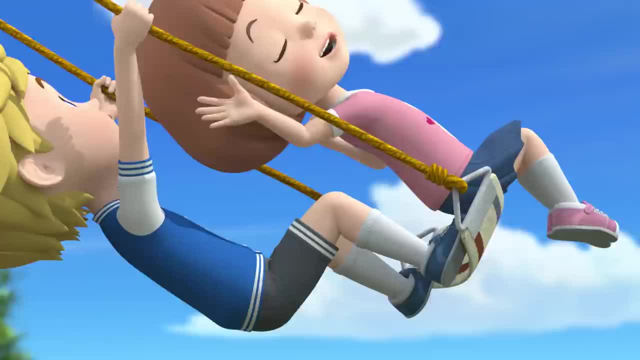 Uh, be careful, Ha-ha-ha-ha. Uh, no hands, Ha-ha-ha-ha. Huh, Lucy, Ah-ha-ha-ha. Oh, no, Ah-ha-ha-ha. 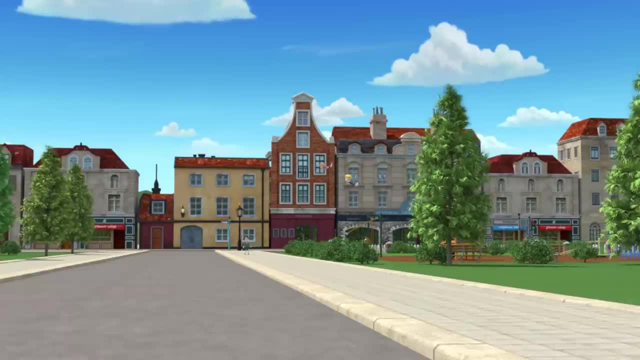 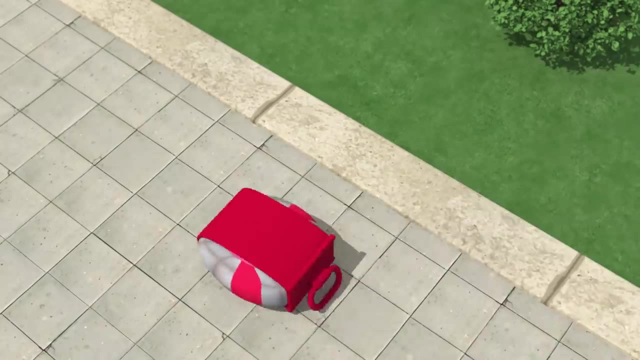 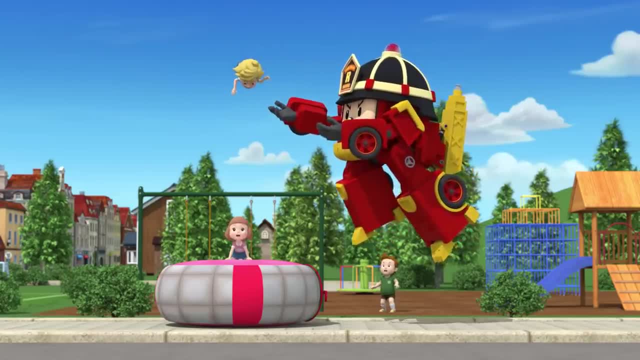 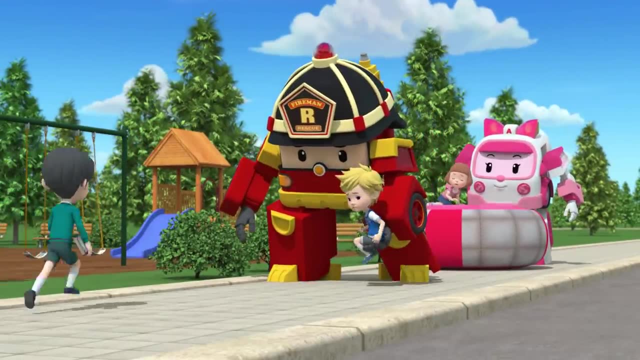 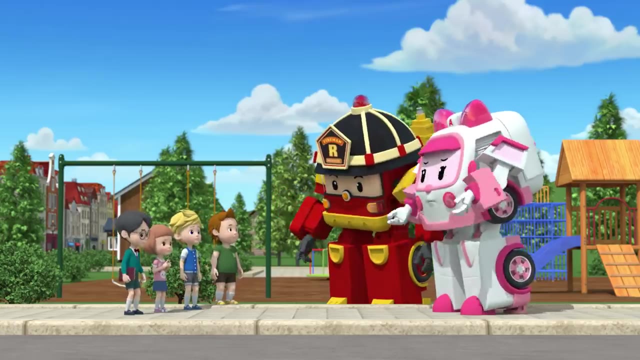 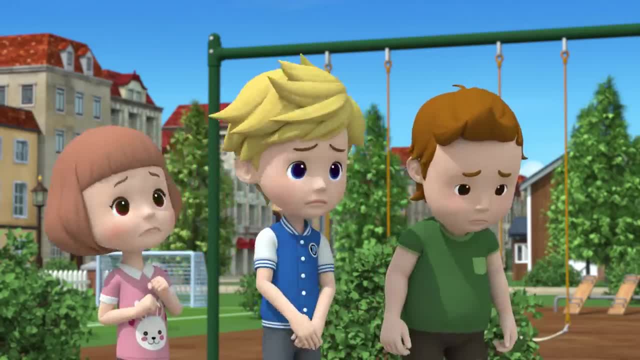 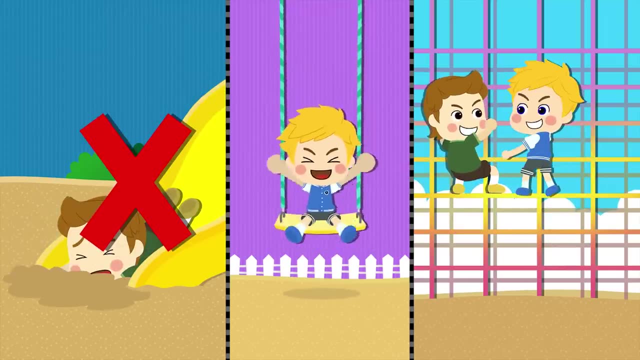 You should have followed your teacher's call. Sorry, We didn't know it was dangerous. Let me tell you how to play safely on the playground equipment. Listen up, Don't ride a slide in a dangerous pose. Don't jump off the swing. 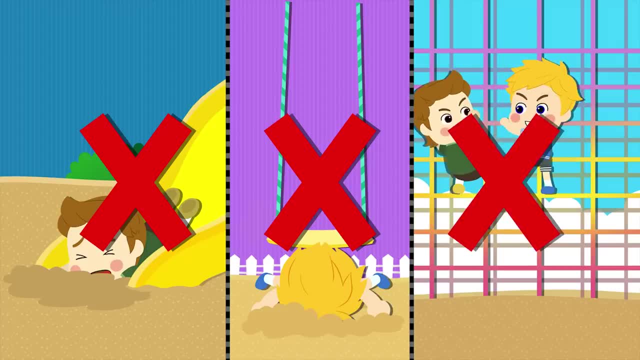 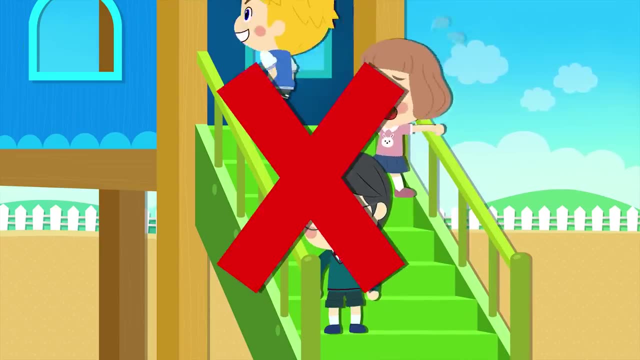 Don't prank each other while you're climbing. Hold the rope tightly with both hands and play safely. Don't try to cut the line to ride first. Never try to push your weight to the front of the line. If you follow all the safety rules. 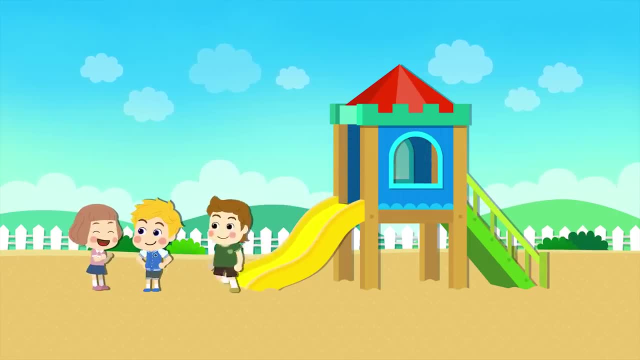 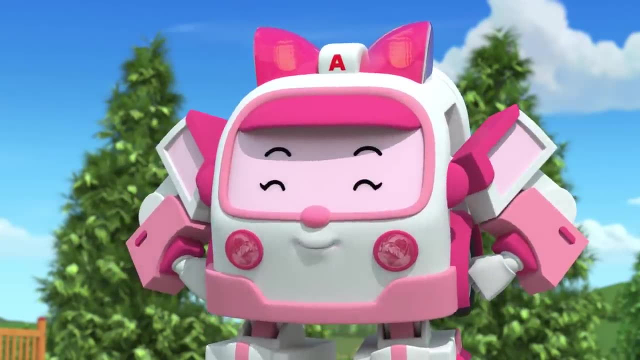 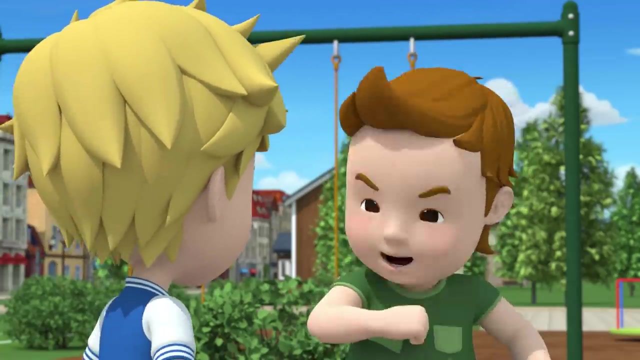 the safety rules, you and your friends will have a wonderful time at the playground. having fun safely will always be the nicest way to play. okay, kids, we promise amber, Lucy, Johnny will be playground safety masters. great, we'll have even more fun that way. Lucy, here's the book that you asked to read. Wow, the. 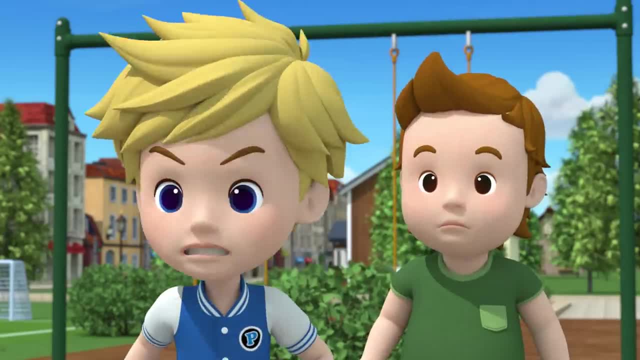 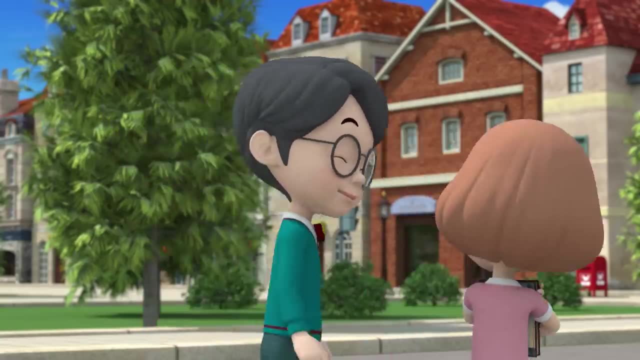 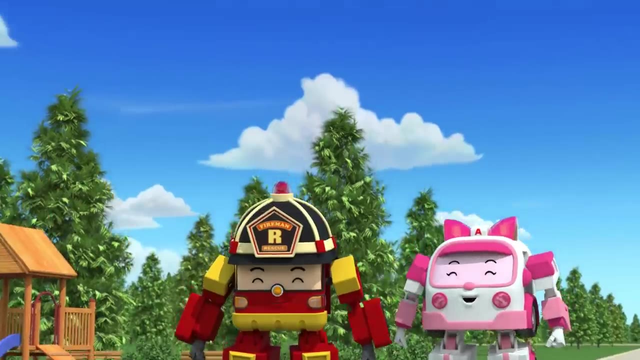 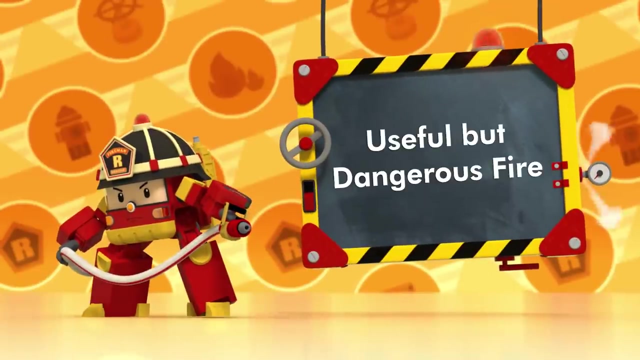 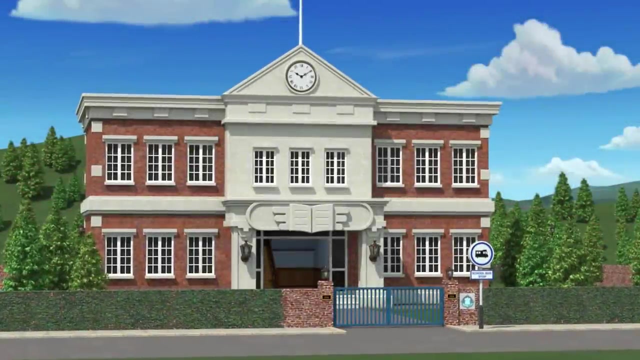 fairytale one. I'll read it now, Lucy, what about us? I've mastered the playground and now I want to read the book that Charles gave me. haha, Lucy, stay and play with us. stay, Lucy, useful, but dangerous fire. fire is useful, but it can be very dangerous, so we must always be careful. now we will. 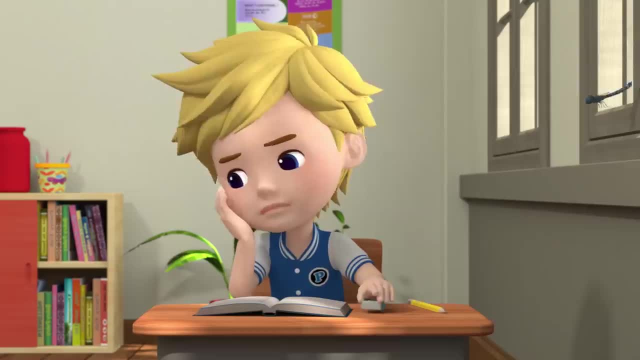 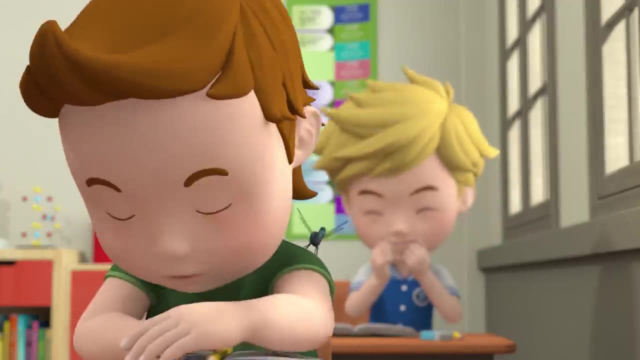 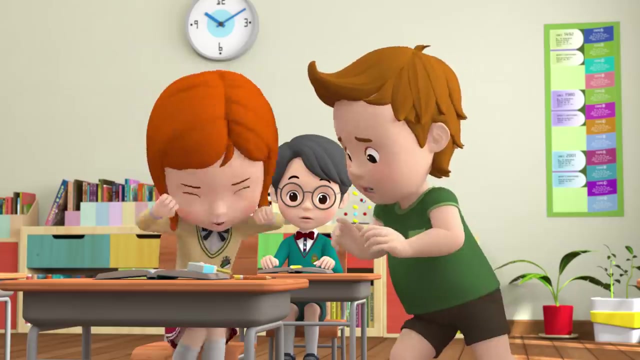 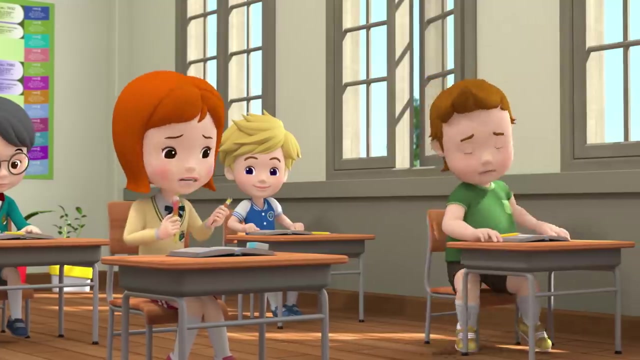 always be careful. now, we will always be careful. now, we will always be careful. learn what to do in case of a fire. so boring huh, Johnny, Johnny, sorry, Cindy, class quiet down, focus on the lesson. Oh, mr pencil tragically struck down. guys, Guys, we have a problem. 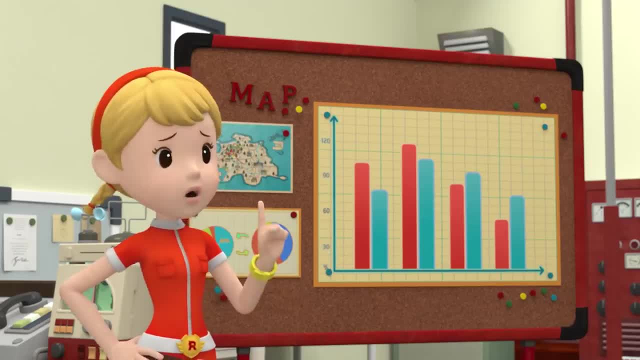 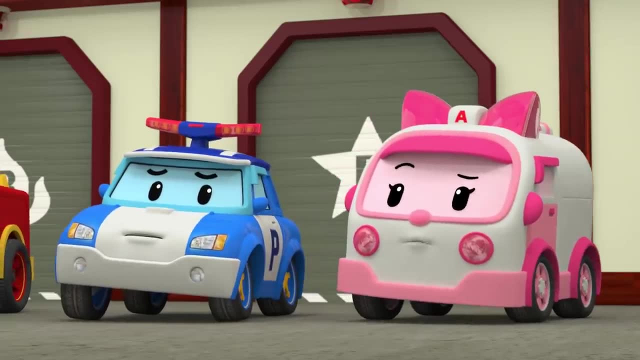 If the results of this survey are right, lots of Broomstowners haven't been taught fire safety. This says some houses don't even have fire extinguishers. Looks like people just aren't aware what causes fires or how to prevent them. 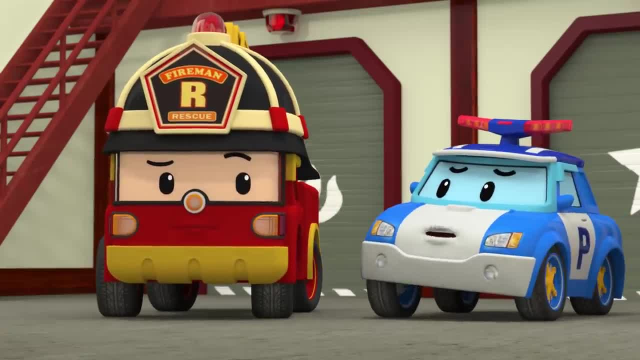 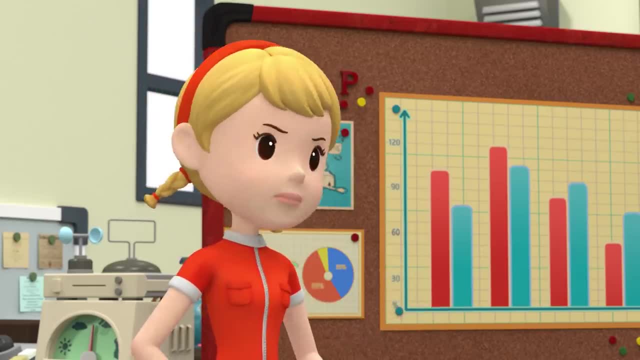 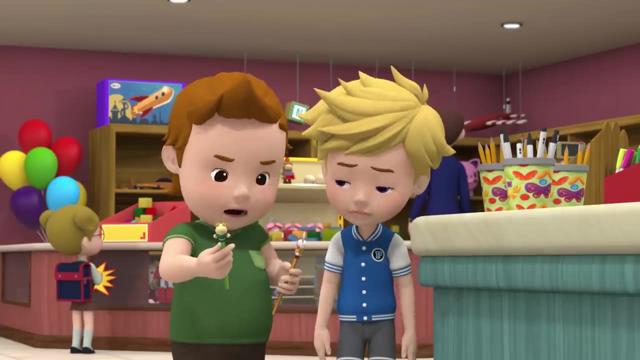 Seems people might not be taking fire safety seriously. Sounds like a serious problem. Yes, it is, And we seriously need to do something about it. We must start teaching people fire safety now. Hmm, the bunny or the doggie, Which one? 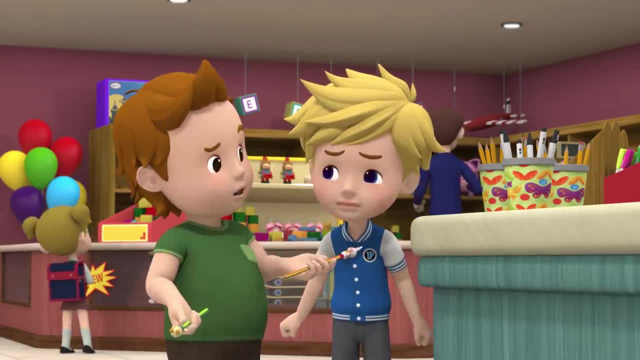 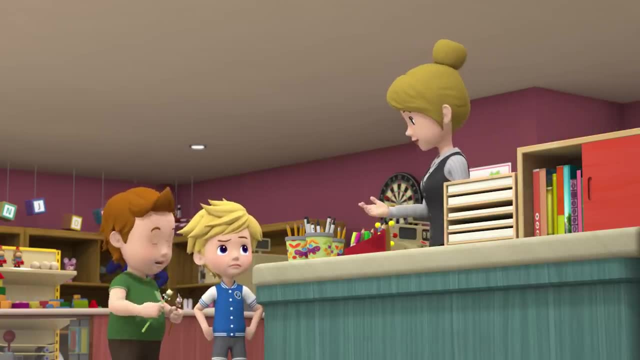 Johnny, let's go to the toy store. Just hang on, Peter, I haven't figured out which one. Do you need some help? Uh, hello, Need help finding something. Yes, I'm just trying to figure out which pencil to get a girl. 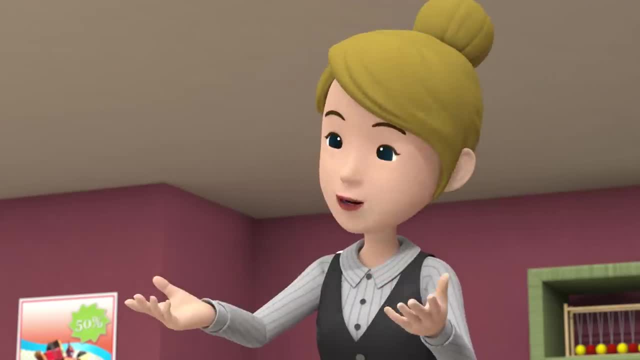 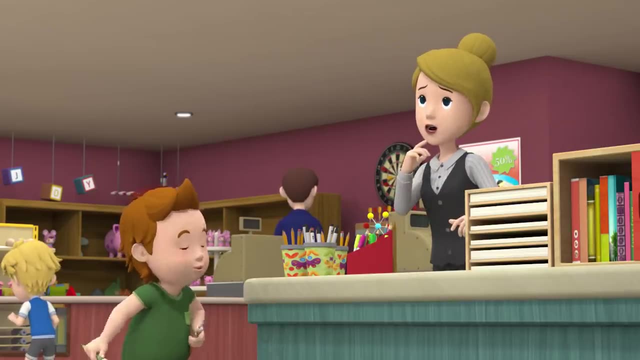 I'm torn between these two. Well, I think she would be happy with either one. Hmm, do you have one with a gorilla on top? A gorilla. I think there might be one in the back. That would rule. I'll just go get it. I'll be back in a sec. 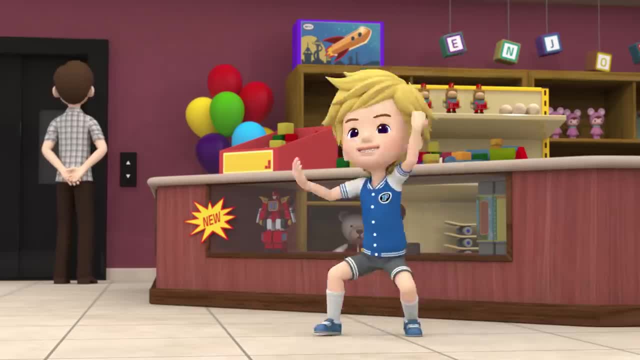 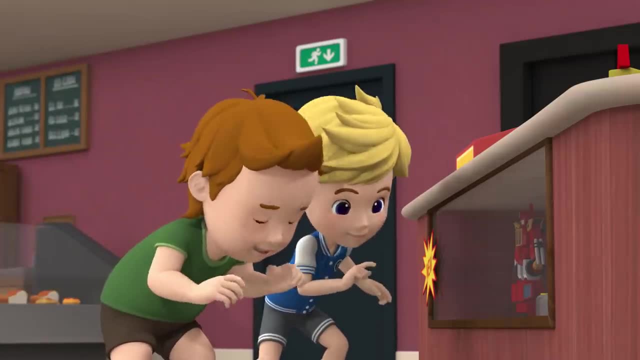 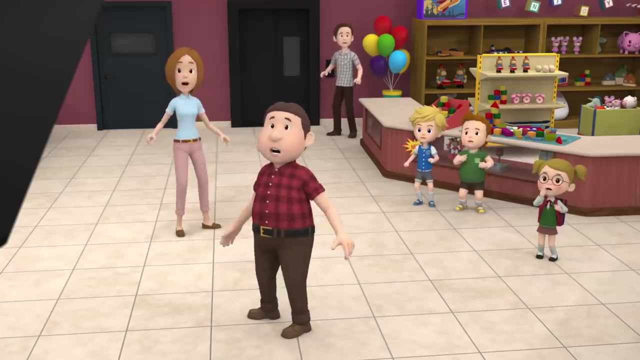 Great, Hey, thanks a lot, Johnny. look A super dragon. Wow, It's awesome. Oh, wow, Wow, Huh. What's that noise? Attention customers: A fire has broken out on the third floor. Please follow the staff and safely enter the building. 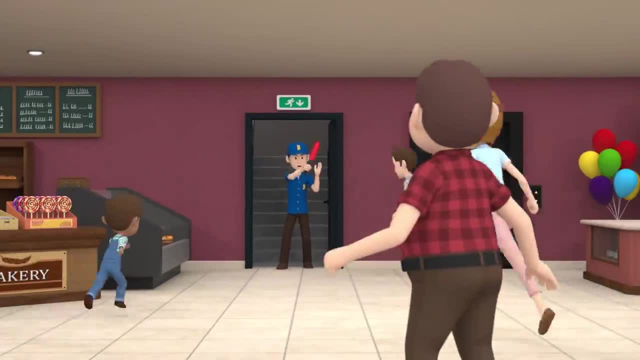 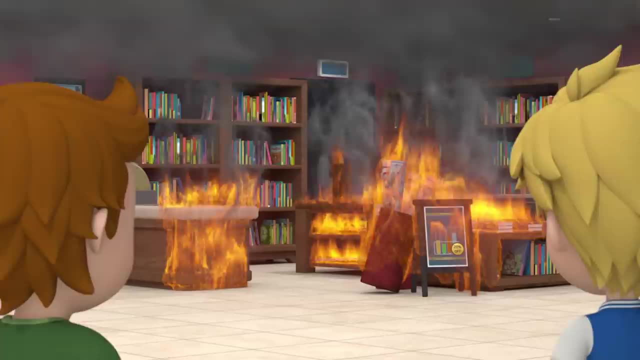 Again. please follow the staff and safely enter the building. Come on this way. everyone Over here, Everyone be careful. Everybody out Be careful. Oh, come on, Peter, look, there really must be a fire. Whoa, I've never seen a real fire. 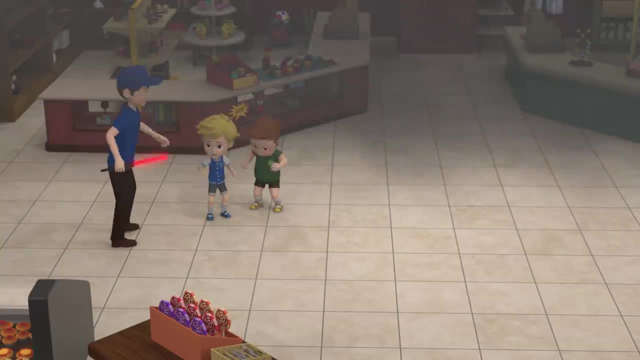 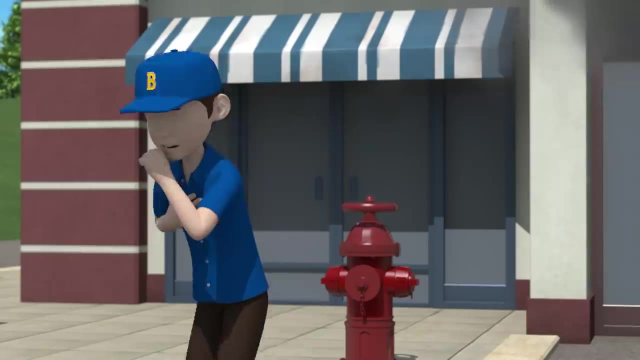 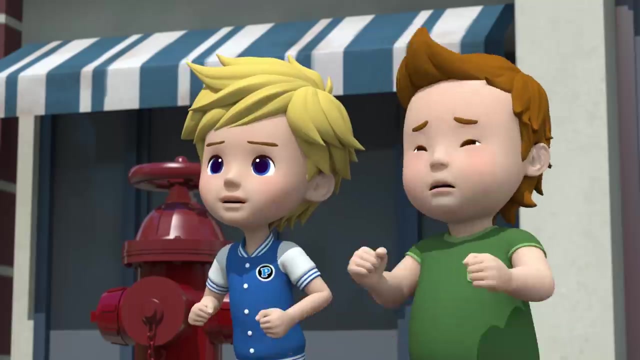 I can't breathe. It burns my eyes. Boys, you're in danger. Follow me, Okay. Children, are you all right? Am I Amber? It's dangerous here. Go somewhere safe. Uh-huh, Ah, Ah. 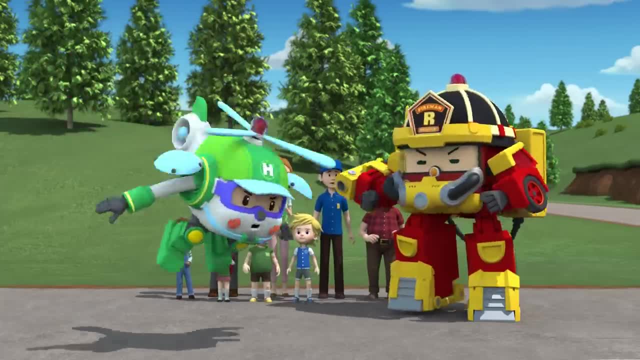 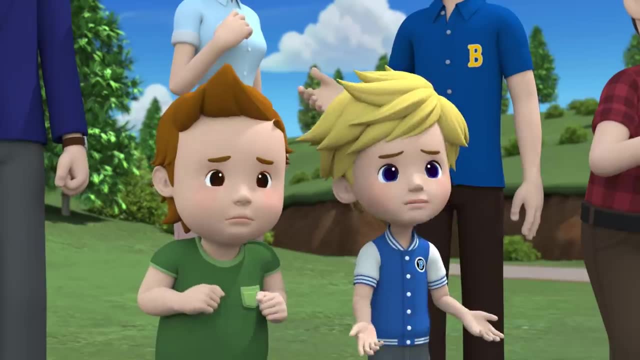 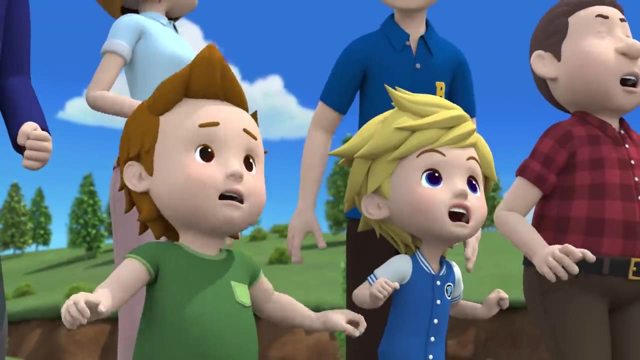 Heli put out the fire on the top floor On it. Who knew fire could spread so fast? Fire is really scary stuff. Ah Huh, Help Up here I can't get out. It's the gorilla clerk. 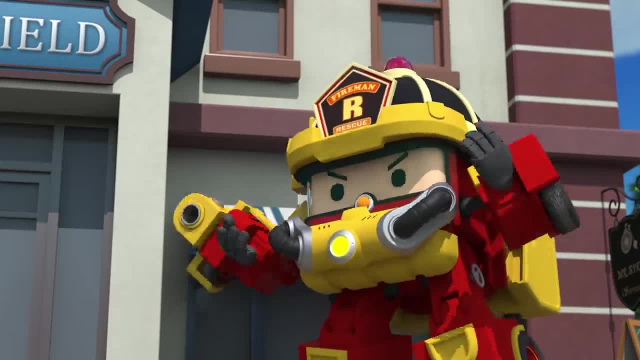 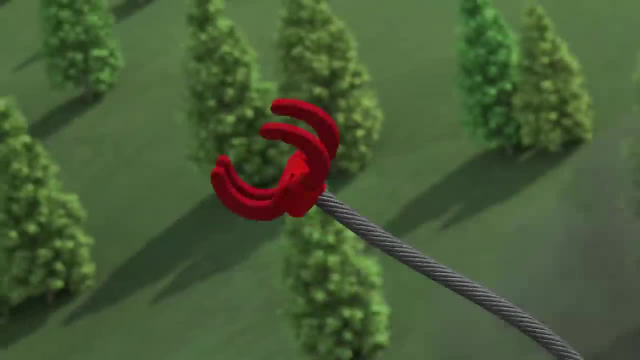 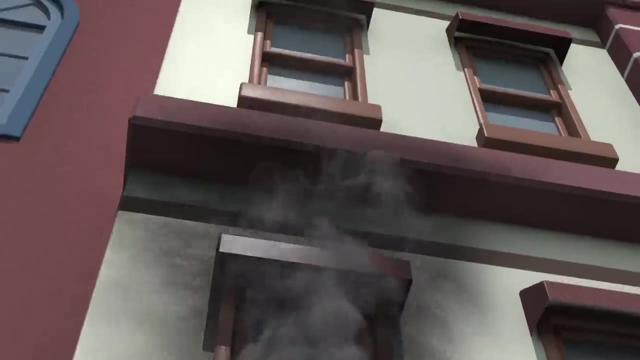 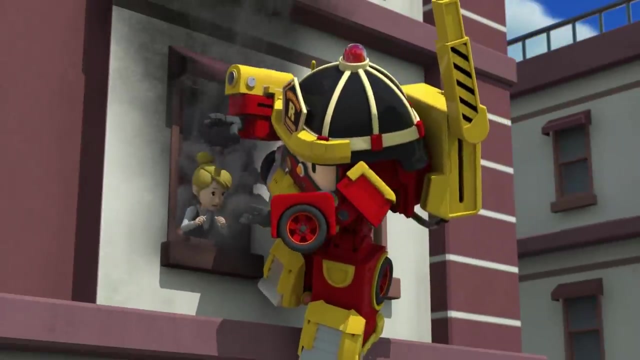 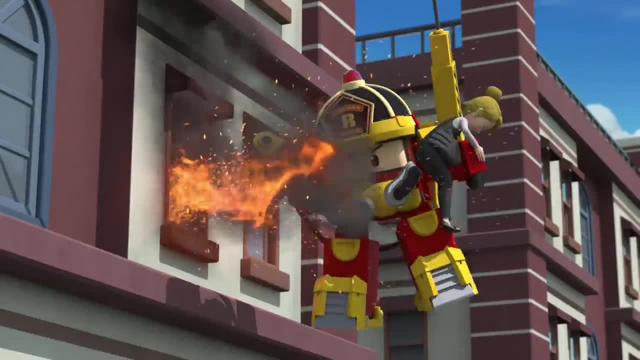 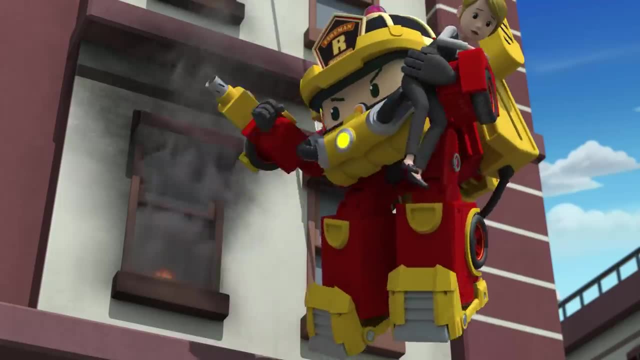 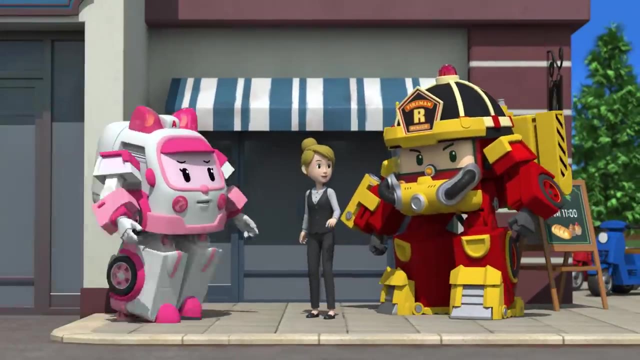 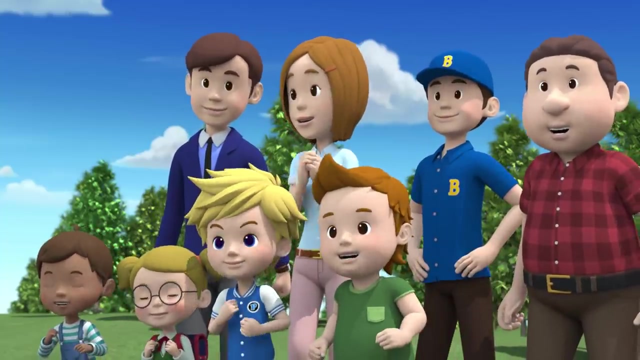 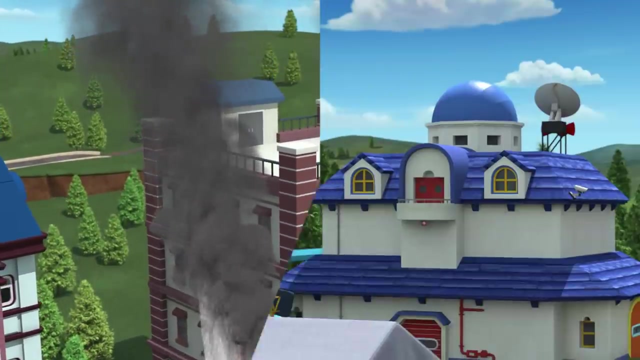 Amber, Amber, Amber, Amber, Amber, Amber, Amber, Heli, please see to the rest Ten-four. Did you get injured at all? I think I'm fine, thanks. Thank you so much. Yeah, Today's topic is scary but useful fire. 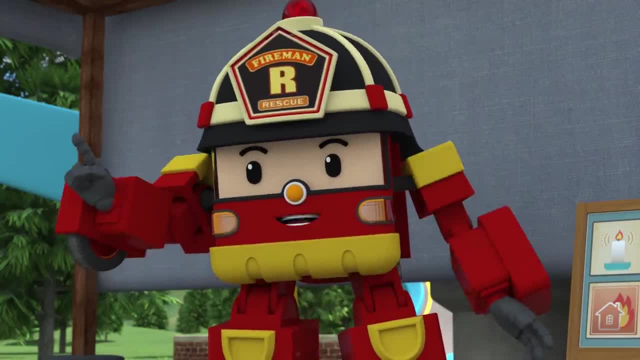 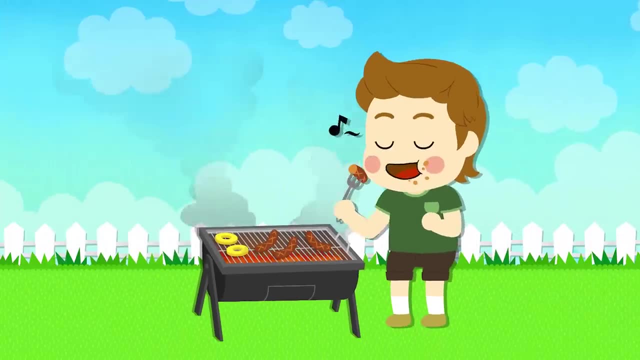 Okay, Roy, Fire is a very powerful and useful element. It lights up the darkness, making life much more convenient. It also heats and cooks food and keeps us warm when the weather's cold. But when a fire gets out of control it can become a very scary thing. 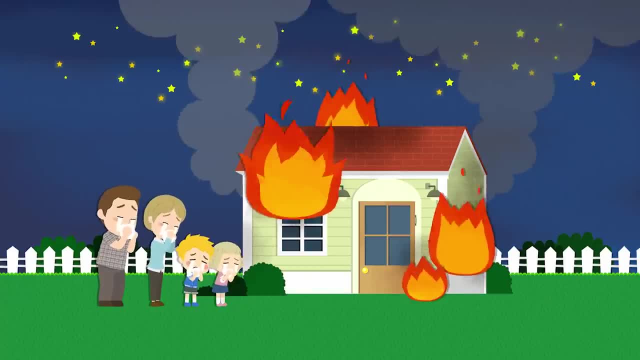 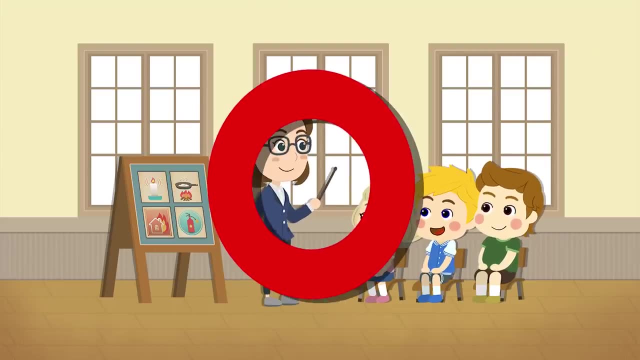 It can burn up not only the stuff we love, but the very house we live in. So it is very important to be properly educated in both fire safety and fire prevention. We must always be alert. A fire can break out at any time. 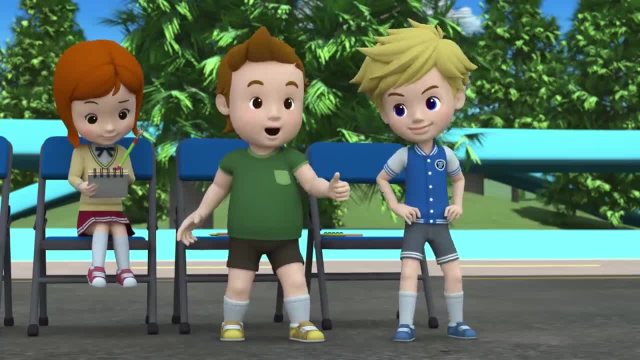 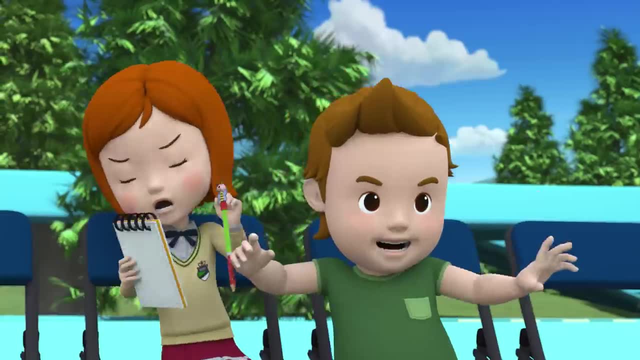 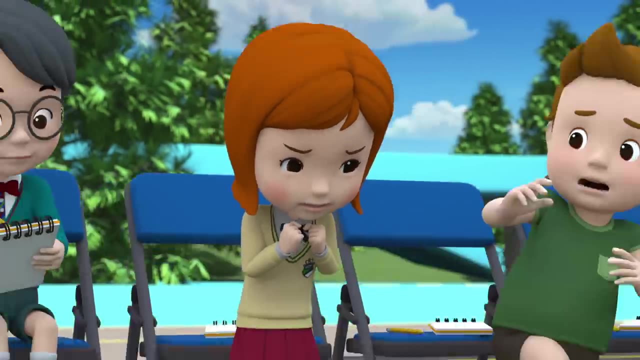 Yes, sir Roy, what you did before was so awesome. Oh yeah, You heroically and bravely saved that trapped clerk When you put out the fire. it was just the best, Johnny darn it. I love that pencil. 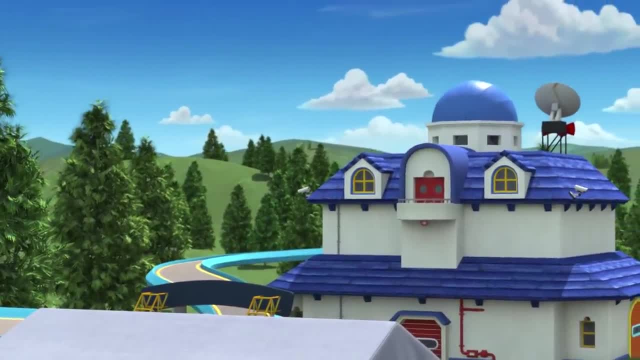 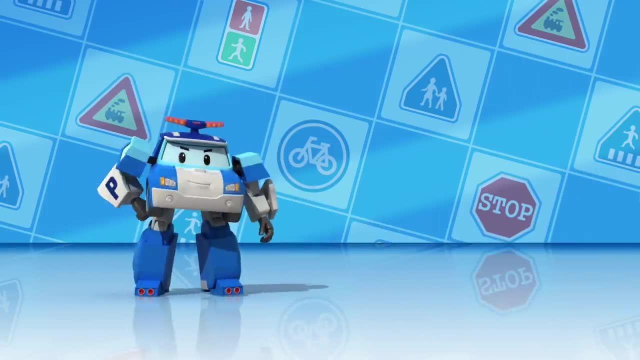 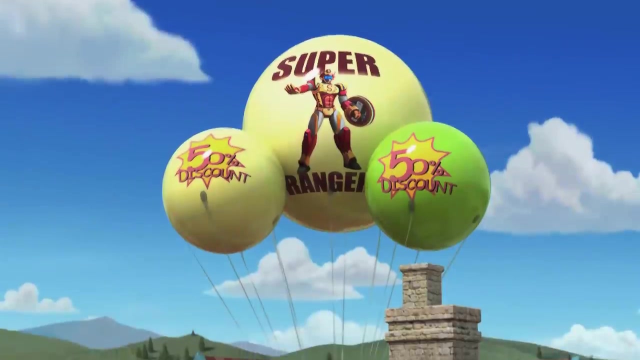 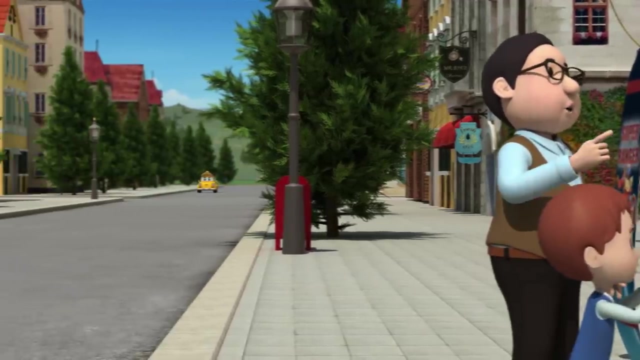 I'm sorry, Cindy, Come back. Uh, Jai-Walking is dangerous. I'll take one, please. I want one too. Wow, 50% off Super Ranger today, while supplies last. That sounds like a pretty good deal to me. 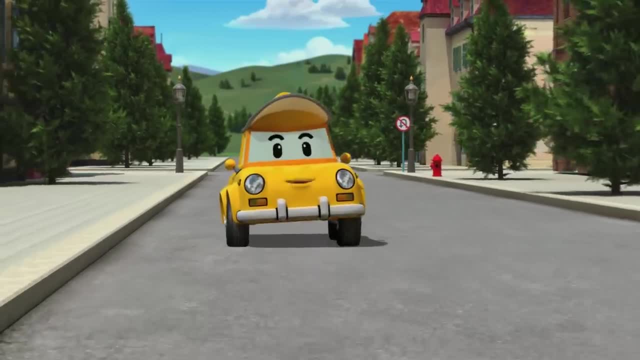 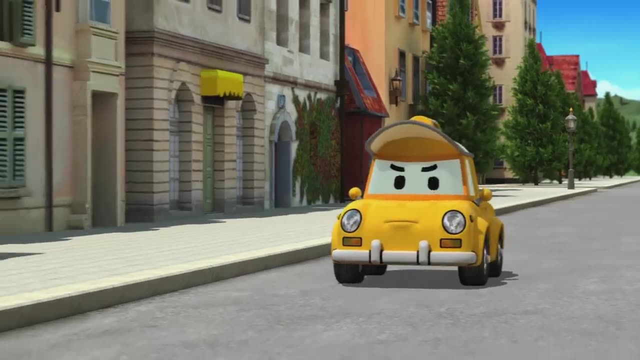 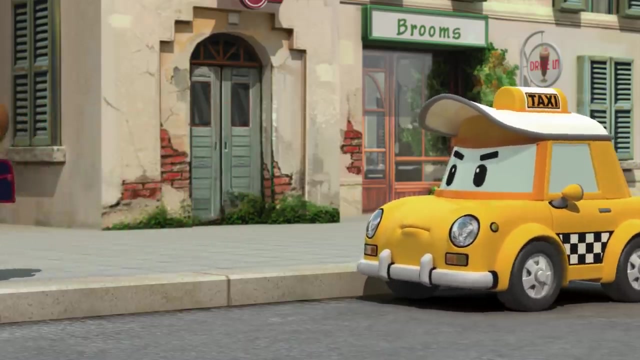 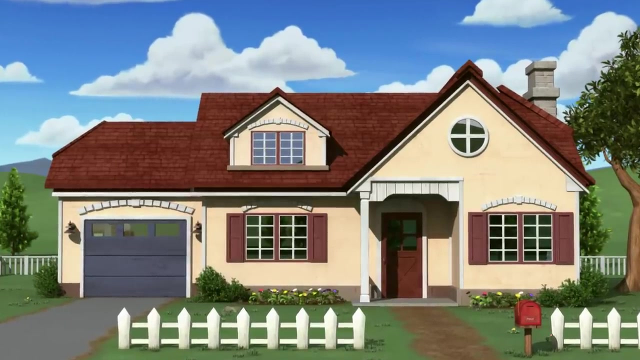 These are the last ones. A Super Ranger half-price sale. Oh hey, don't you know that's dangerous? This is awesome. Pay attention, You know, this isn't a crosswalk. This is a bad situation, Mom. I just have to have a Super Ranger. 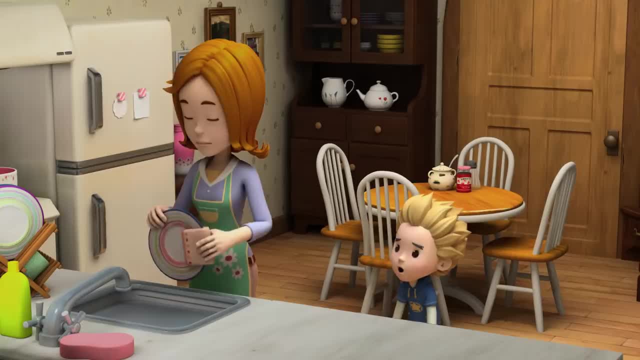 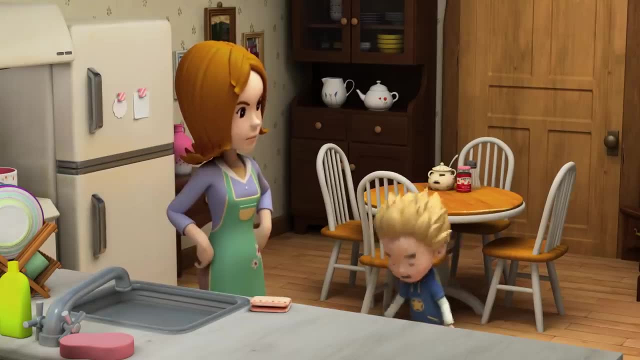 Please, If we don't get to the store today, they're all going to be gone. No way, Why not? Why not? Why not? Because I bought you a new toy last week, But, Mom, that wasn't the Super Ranger. 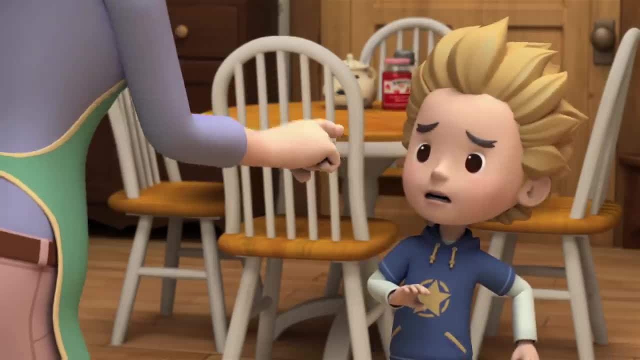 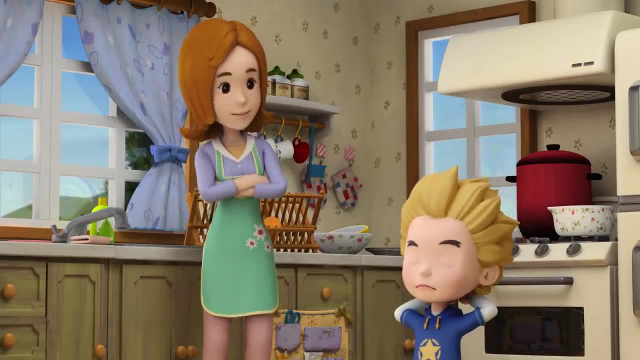 Hey, you promised me When I got you that toy. you said you'd study hard, play with your sister and put all your toys away. Remember that? Not really Okay. Well, if you can't remember, then I'm sure you'll forget all about Super Ranger in a day or so too. 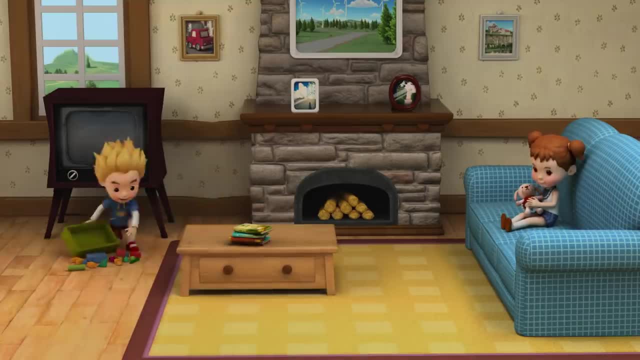 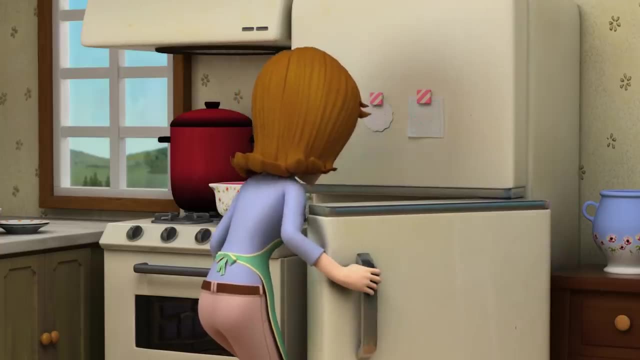 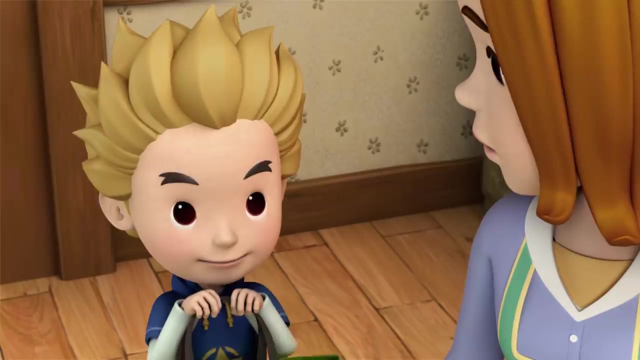 I remember: Oh my, We're out of vegetables. I need some juice and a quart of milk too. I suppose I'll have to go to the market today. Huh, Come on, Mom. We better hurry, Kevin. what's all the rush? 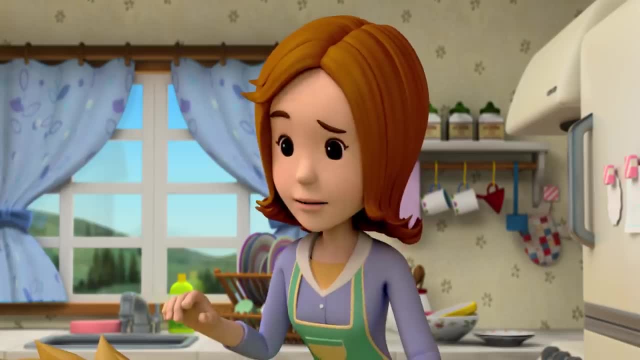 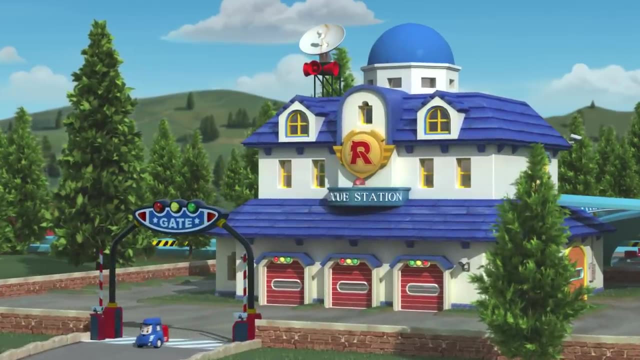 Well, I thought we could stop at the toy store on the way there. Uh, I don't know. You're the best Mom. Oh, my Hooray, I finally got it. What is that, Jin, This? 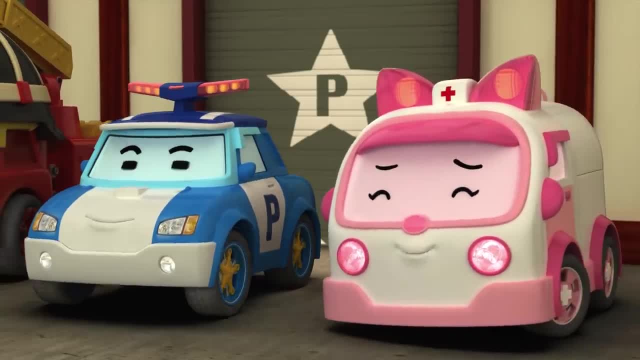 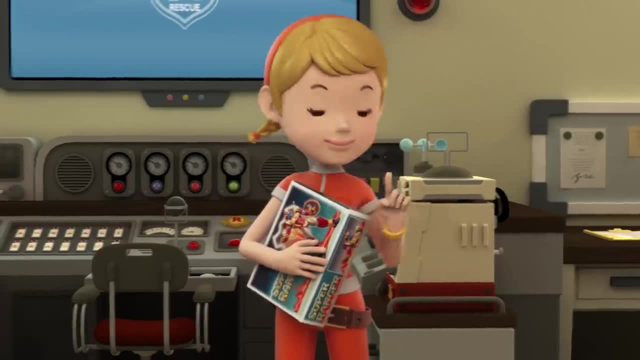 Ta-da, It's Super Ranger, But, Jin, you're not a kid, Amber. for your information, adults can be fans of Super Ranger too. Huh, Rescue team. this is Jin Hiya. Jin, Oh hi. Cap. 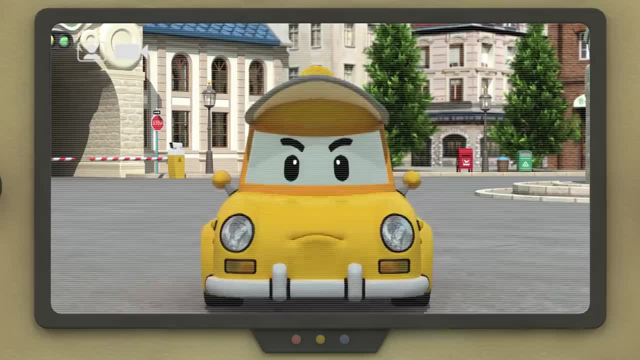 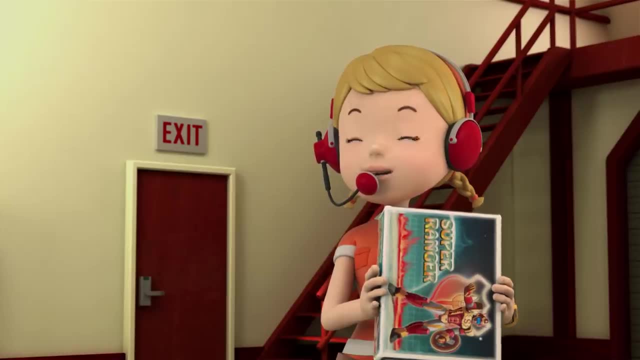 Guess what? The store's having a Super Ranger sale. That's why I called. There's lots of people going to the store and some of them aren't crossing a- Oh no- The crosswalks. If we don't do something, there could be an accident. 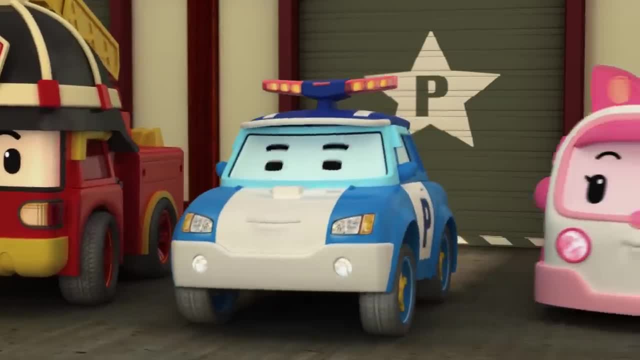 We're on the way. I'll go Jin, Me too, Polly. First stop: toy store. All right, but you have to keep your promise, Don't worry, I will. Ah, One left. That's the last one, Mom. 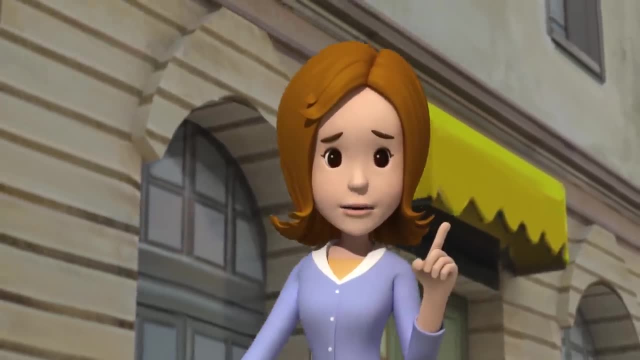 Let's hurry. Huh, No, Kevin, We have to use the crosswalk. Huh, I don't see a crosswalk. I see it, I see it. No, I don't. I don't see a crosswalk. 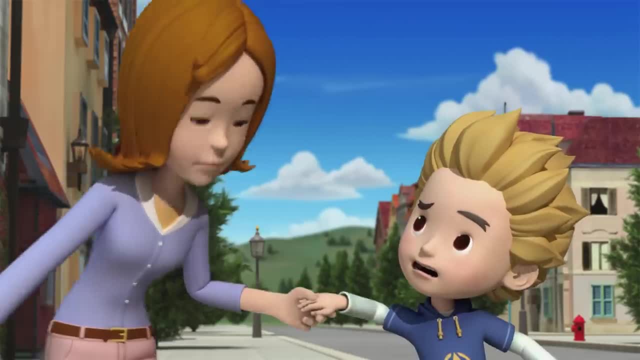 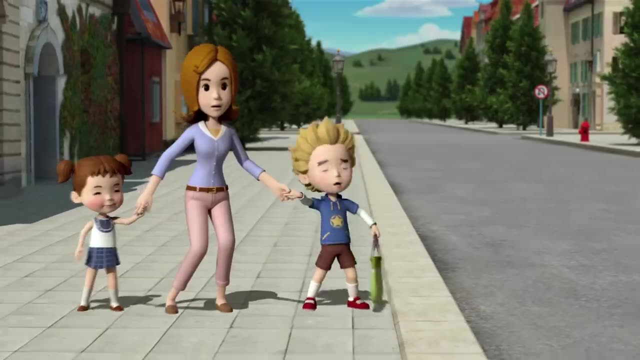 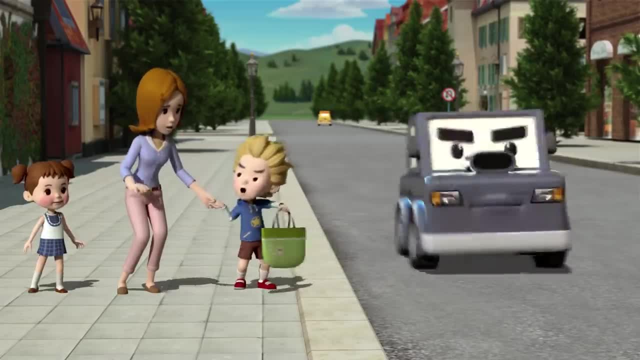 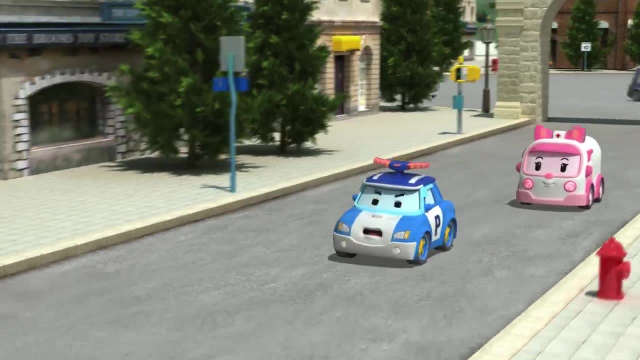 Kevin, wait, What's that? Oh, that's too far. Hey, that guy's not crossing at the crosswalk. How come we have to? Oh, no, I'll take it. Ah, No way, Polly Look. 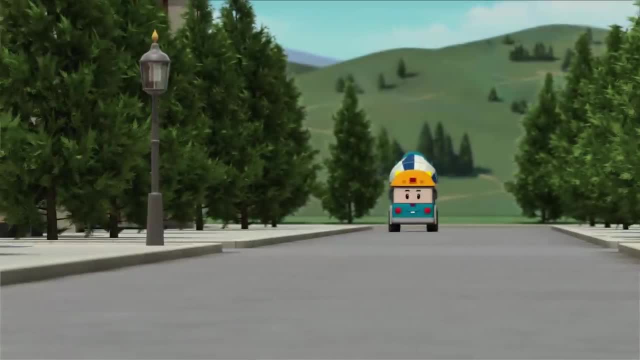 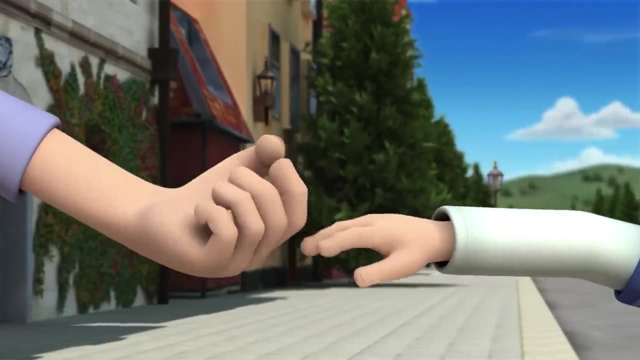 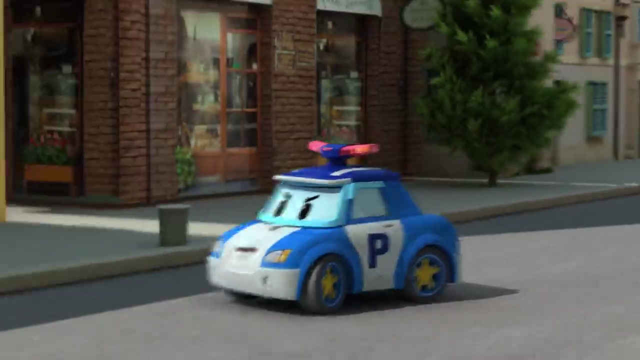 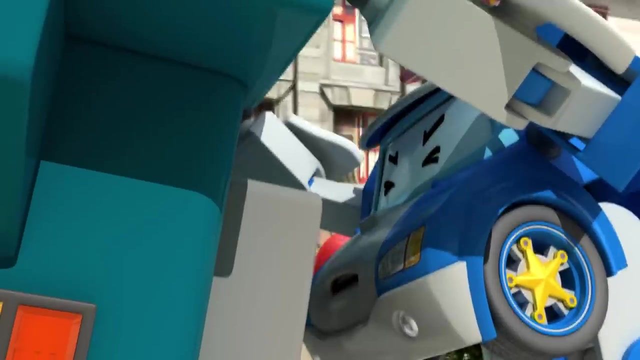 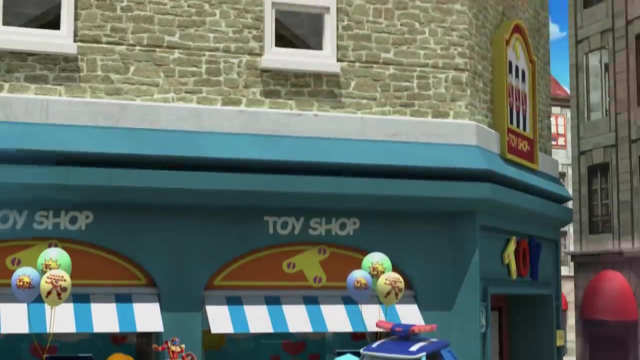 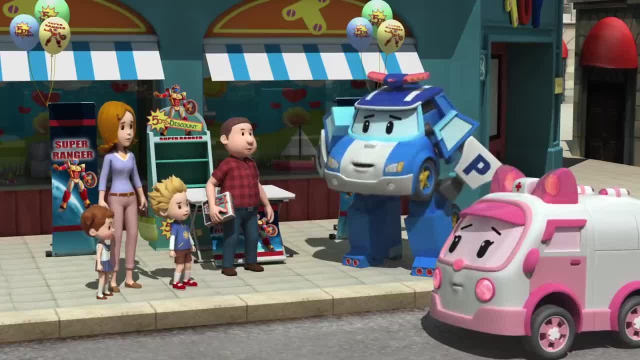 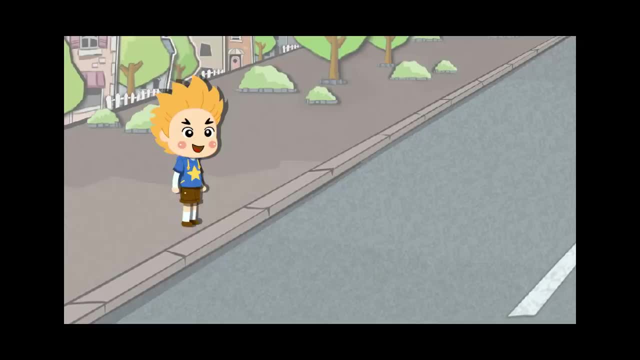 Jaywalking's not only dangerous and such a bad example, but it's illegal. Guess, I wasn't thinking Polly. When children see adults jaywalking, they think it's OK, And that could lead to some terrible accidents. Gah. 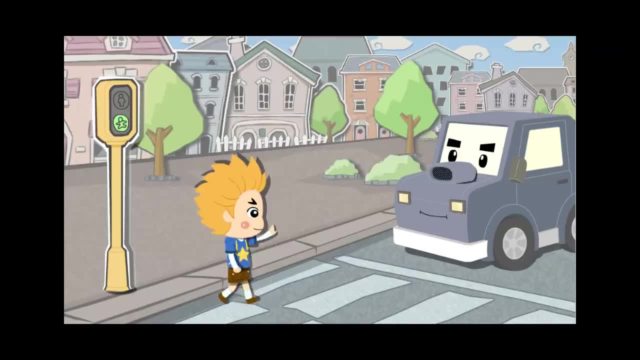 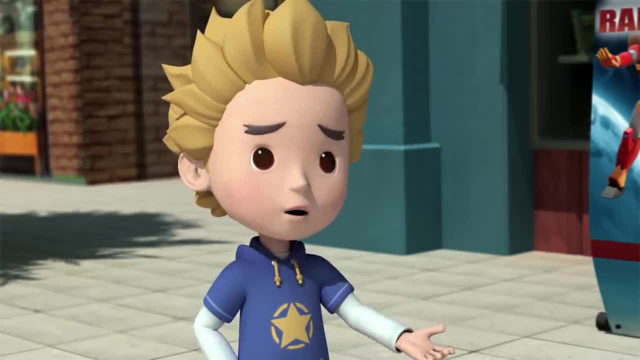 Remember, Kevin, be smart whenever you cross the street. Use a crosswalk, an overpass or an underpass, And always obey the lights. Yeah, but what if the crosswalk's really far away, Polly? The important thing is safety. 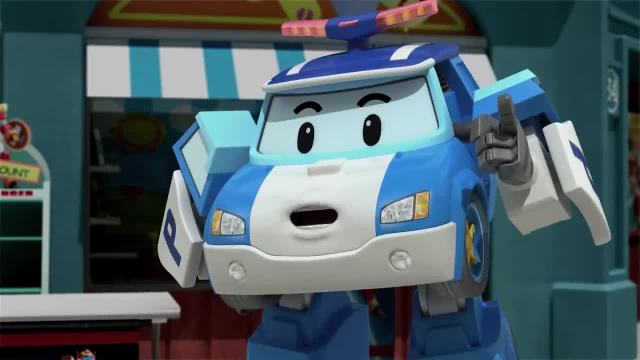 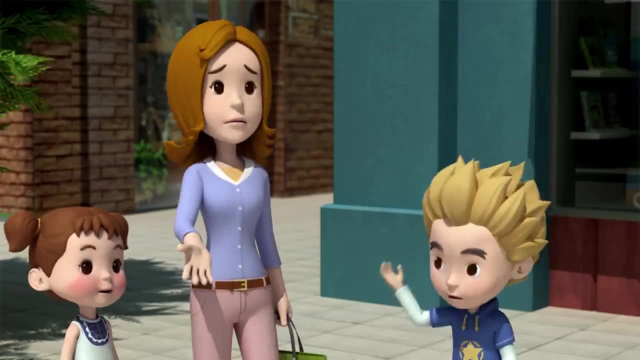 Even if it takes more time when you're in a hurry, it doesn't matter if a ball rolls into the street or if someone's calling you. There's never a good reason to jaywalk. You're right, Polly. I was holding his hand, but somehow he got away. 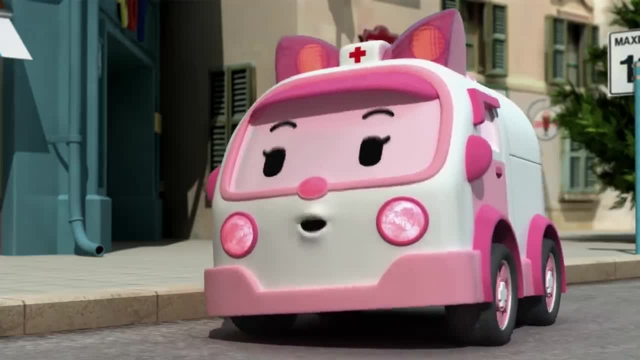 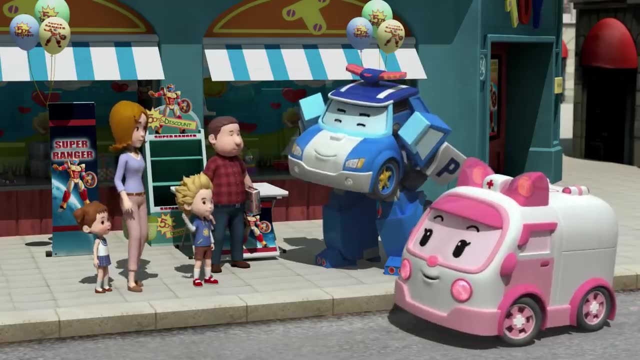 That happens quite a bit, ma'am, But there's a much better way to hold on. It's pretty easy for kids to get out of hands, So hold their wrists for a better grip. I'm very grateful to the both of you. 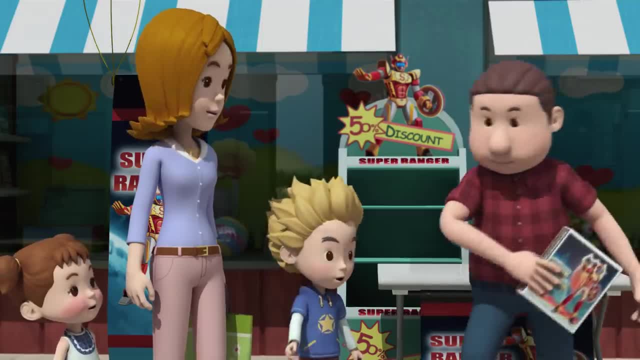 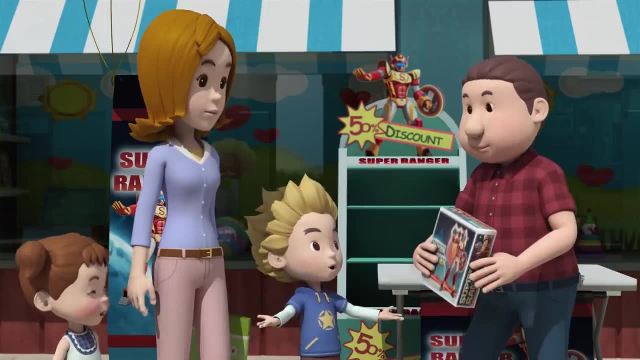 Yeah, me too Here. this is for you. I'm sure he's your hero, That's really nice, but I want a bigger hero than Super Ranger. What Bigger than Super Ranger? Yep, Now I want my very own. 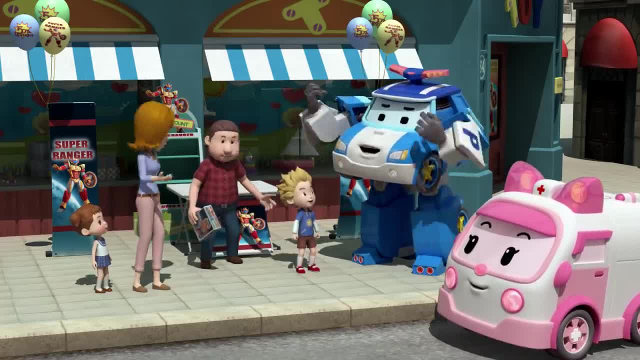 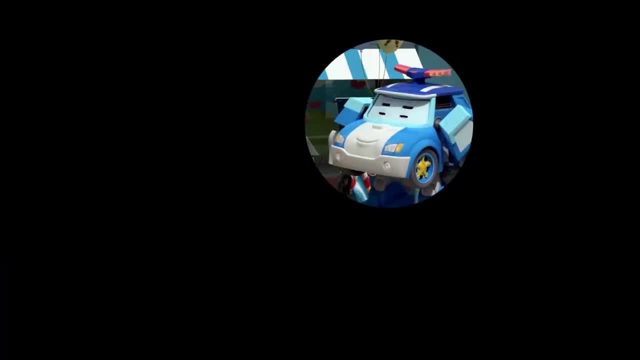 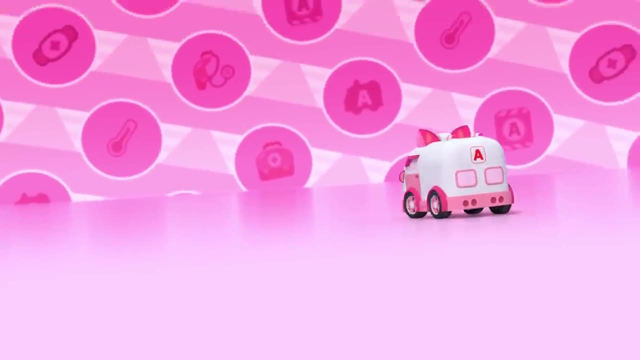 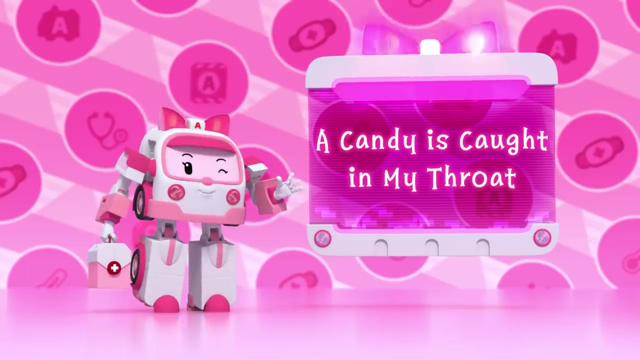 Polly. Sorry, Kevin, but I'm afraid I'm not on sale, Then I'll pay full price. Never jaywalk And always cross at the crosswalks. See you next time A candy is caught in my throat. Hello, Mr Wheeler. 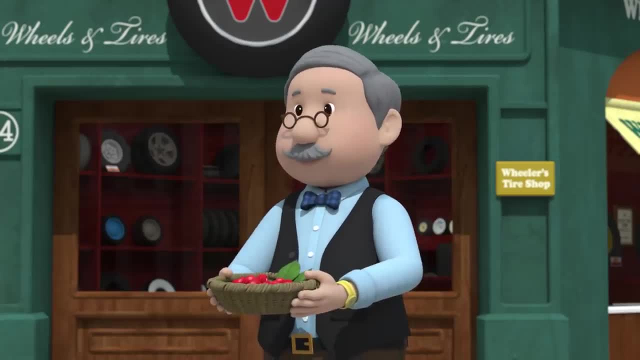 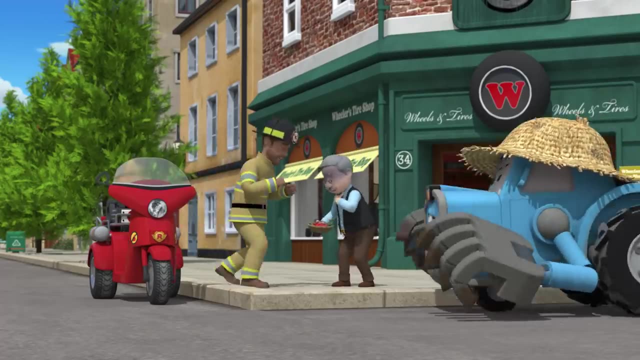 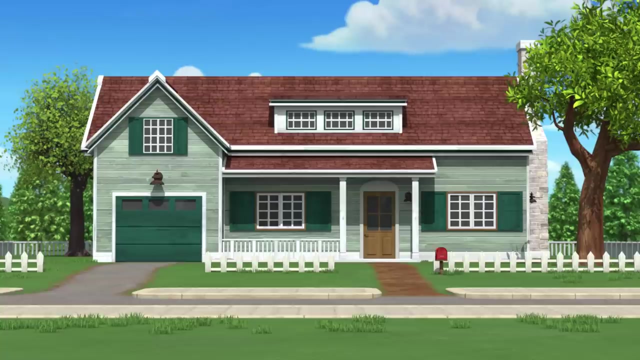 Hi, Tracky Morning. Tommy, You're just in time Have one of these fresh raspberries. Tracky gave them to me. They're just heavenly. Mr Wheeler, I'm all right. Thank goodness you're fine. Lucy, check this out. 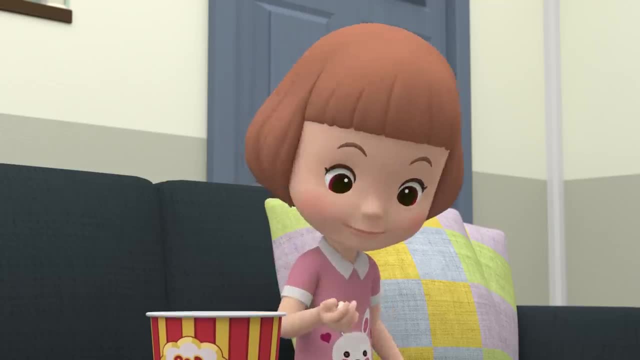 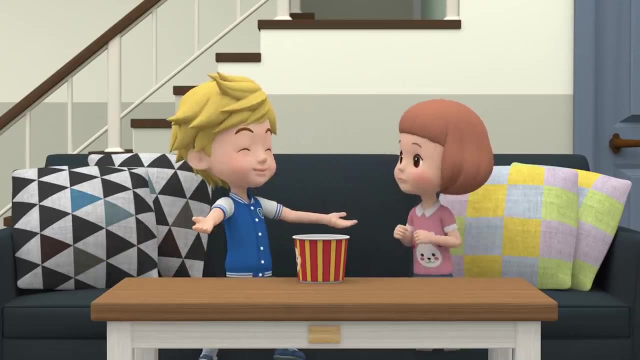 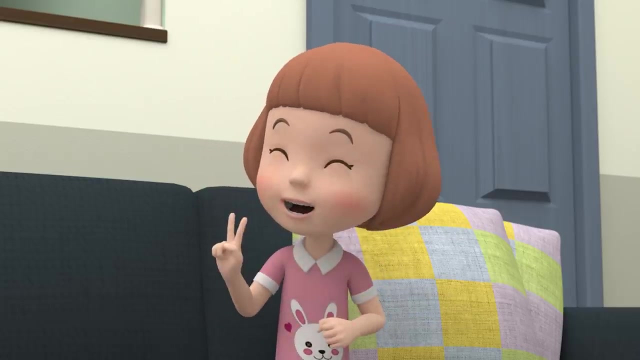 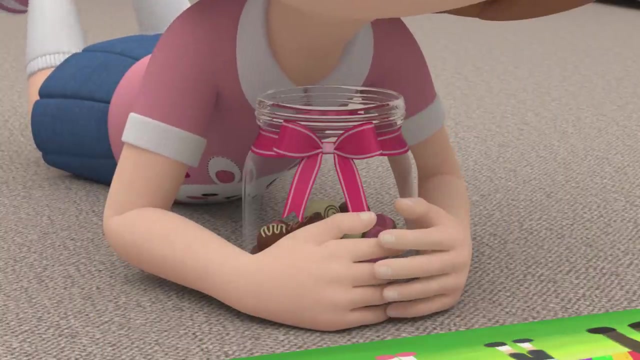 Who's the best? Wow, I want to try it. Aw, Watch what I do. Ta-da, I'll do it this time. All right, Huh, Peter, how could you eat all the popcorn? Lucy, can I have one little chocolate? 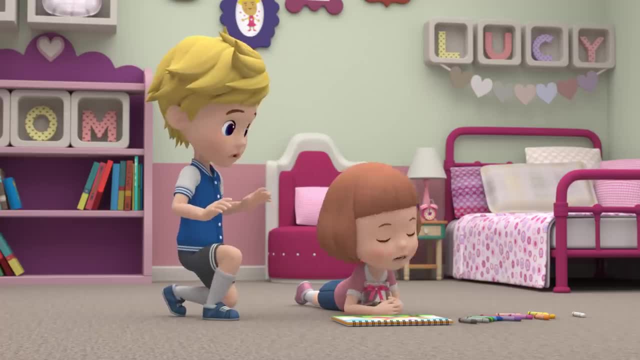 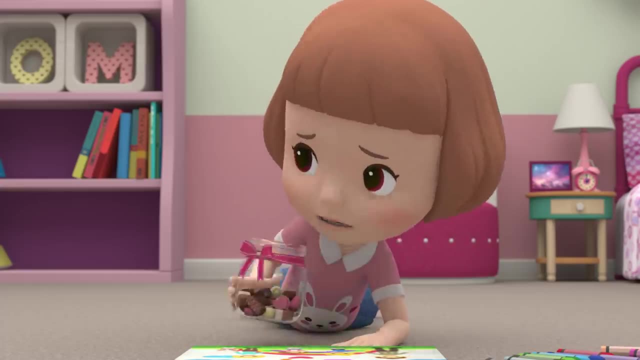 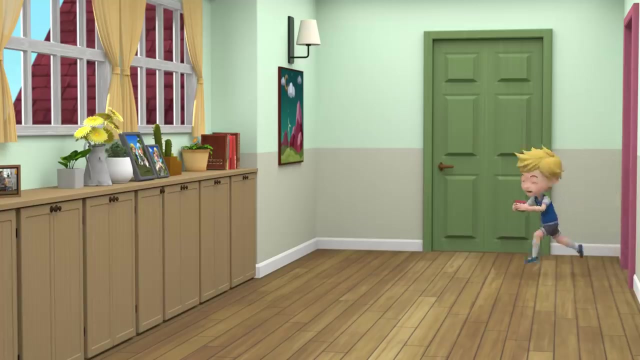 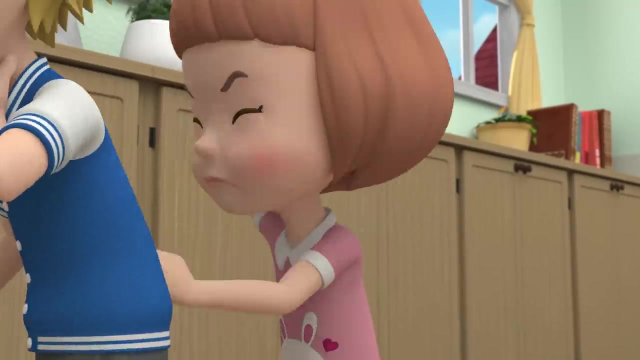 Sorry for before. No, just one. Nope, that's not going to happen. Only one, I'm begging. Hmm, Huh, Fine, I'll have one. Hmm, Hmm. Thanks, sis Peter, Just give it back. 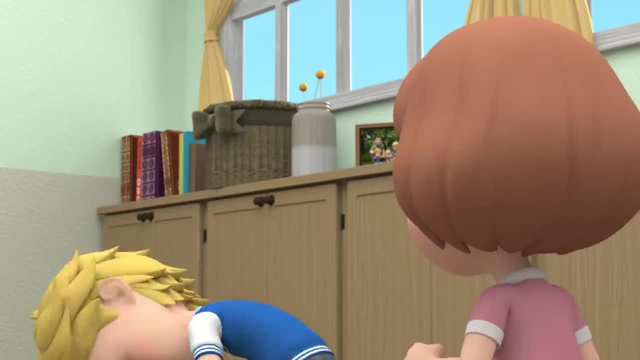 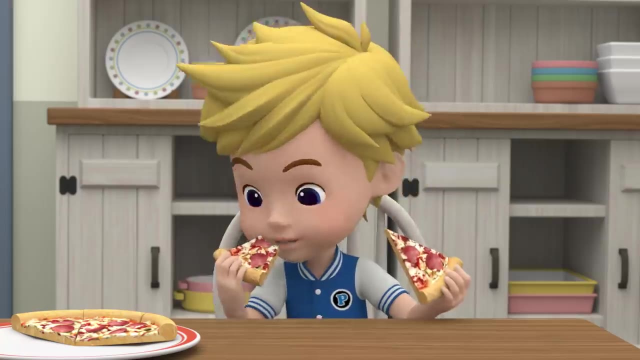 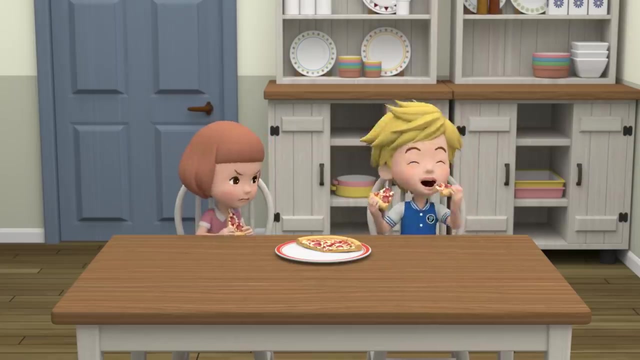 Whoa, that felt bad. Lucy, you want to eat this? Ew, that's gross Kids pizza. Yes, Peter. Oh, You ate two pieces at once. Stop, You can eat just like me if you want. 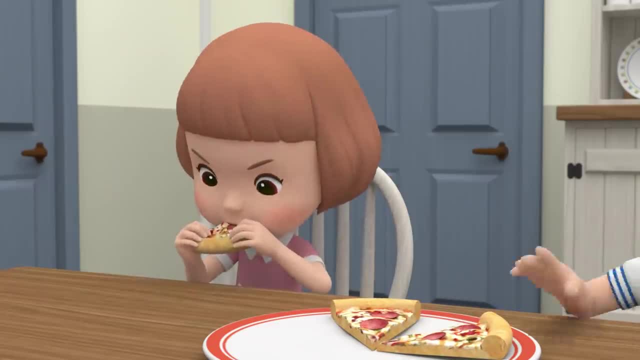 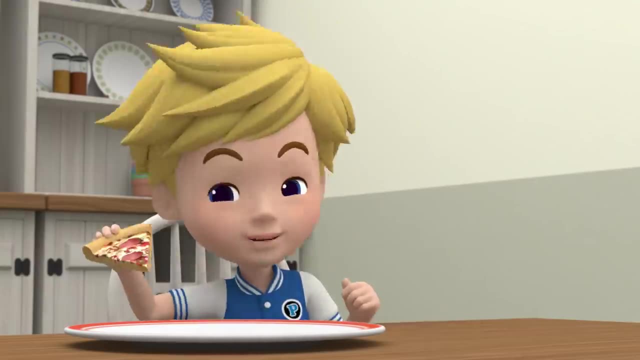 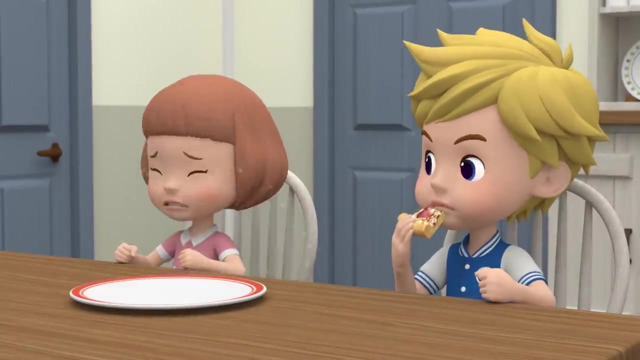 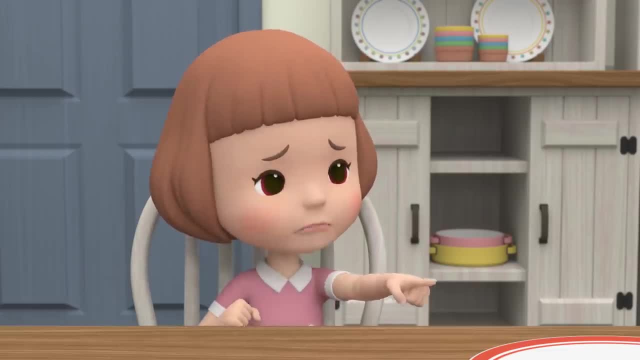 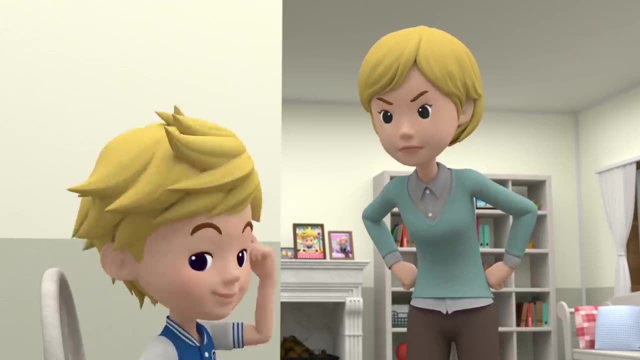 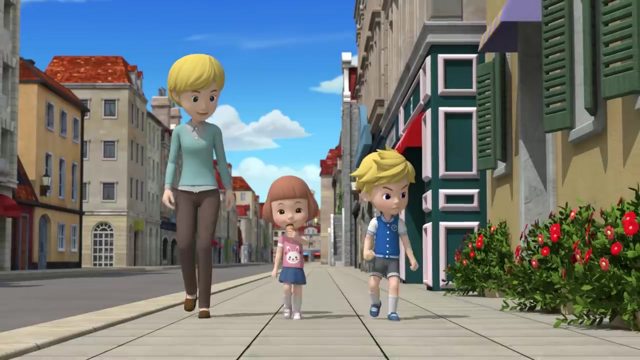 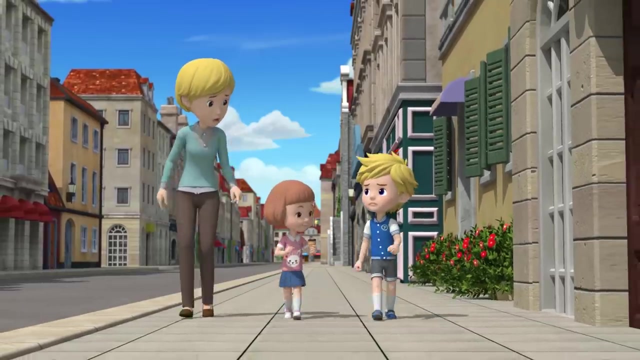 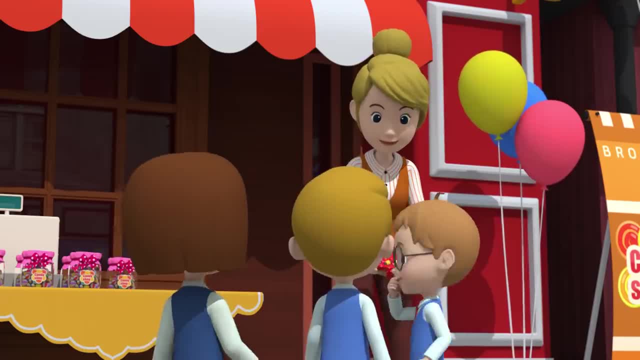 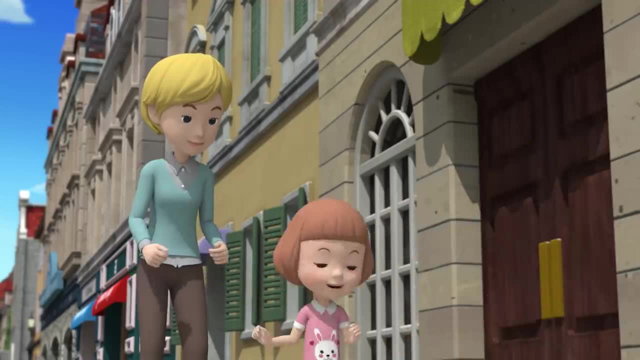 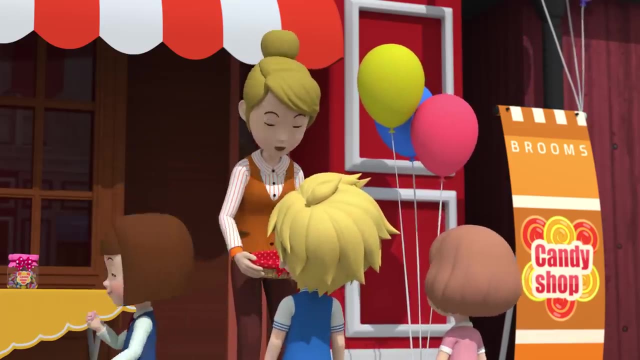 No, sir, you ate too many snacks already. Yummy, Can I have one Me too, Of course, Here, Whoa Free candy, And they're off. Welcome, Help yourselves, Thank you. Oh, Yummy free candy, please, ma'am. 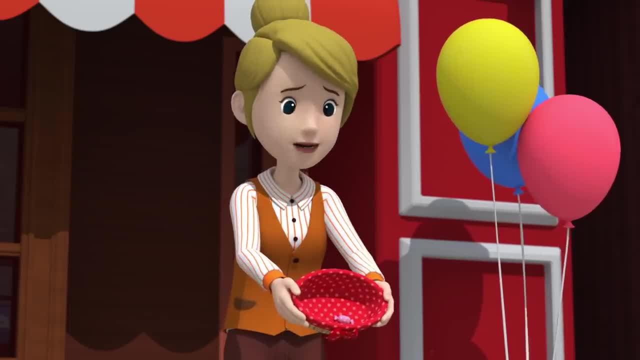 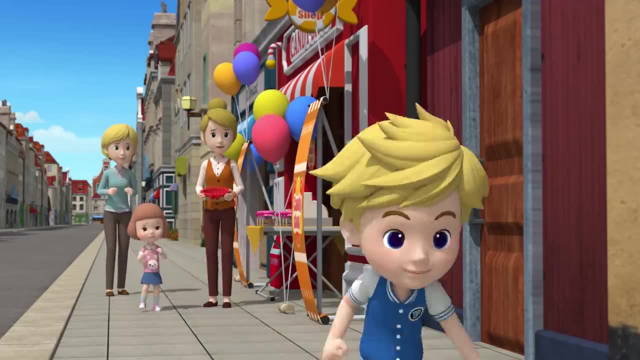 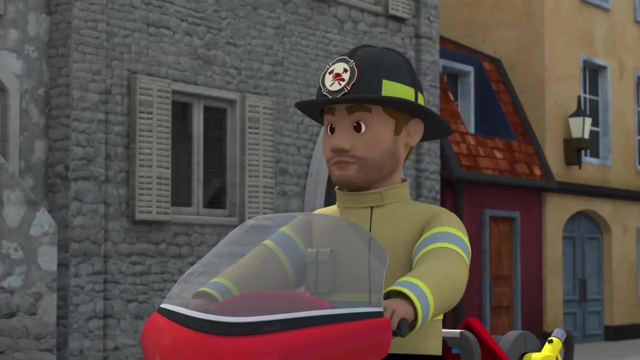 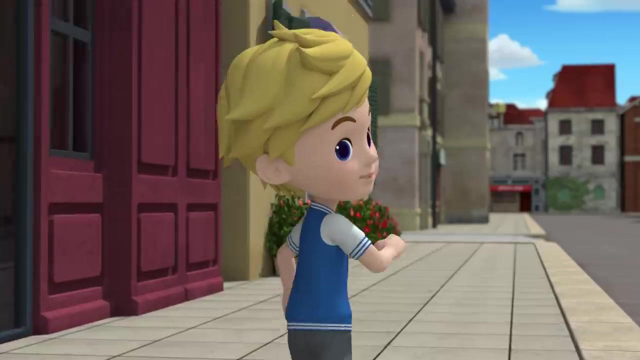 Me too. Oh dear, It looks like there's only one piece left, Only one. This is mine. Peter, Peter, Lucy, Stop, Peter, What's this? Hey, Stop. That piece of candy is mine. That's funny, Then why is it in my mouth? 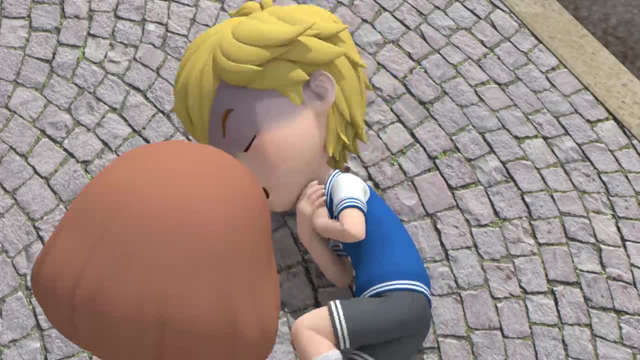 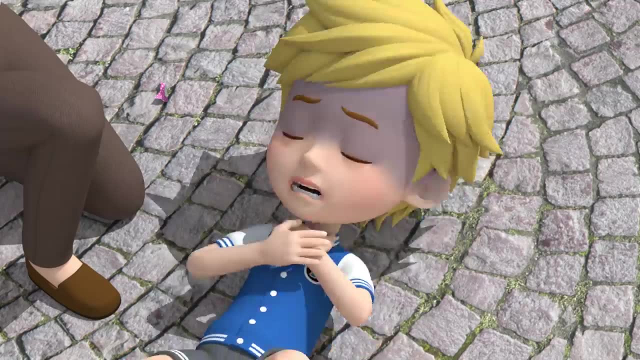 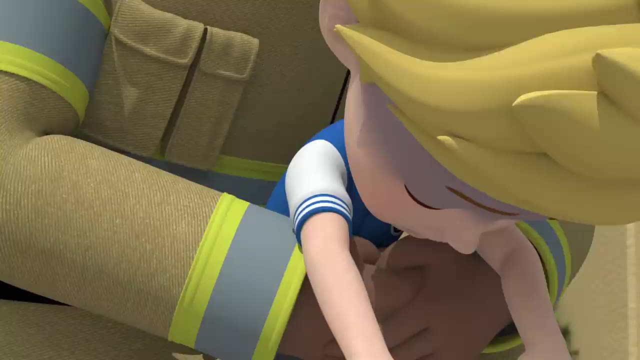 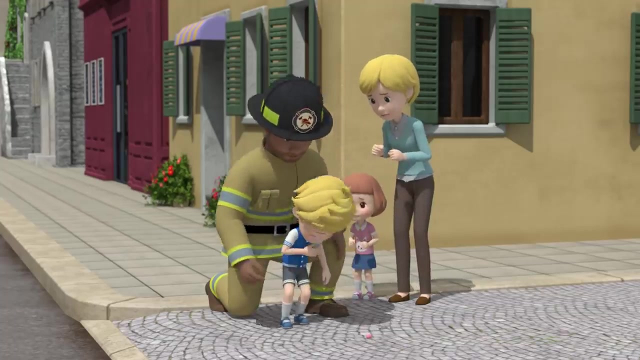 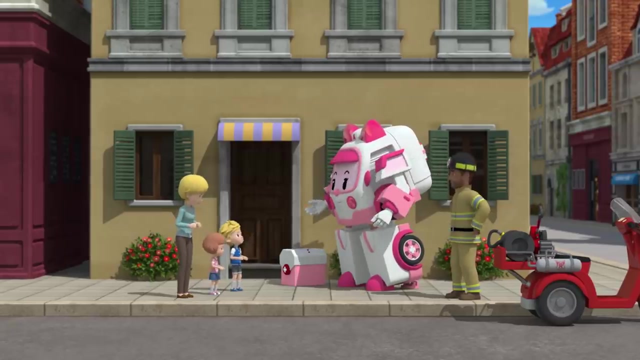 Serves you right. What's wrong, Peter? What's wrong son Peter? The candy must be stuck in his throat, Peter. Hang in there, Peter, Feel better. Yeah, Phew, Thank you so much. You're lucky. you're all right, Peter. 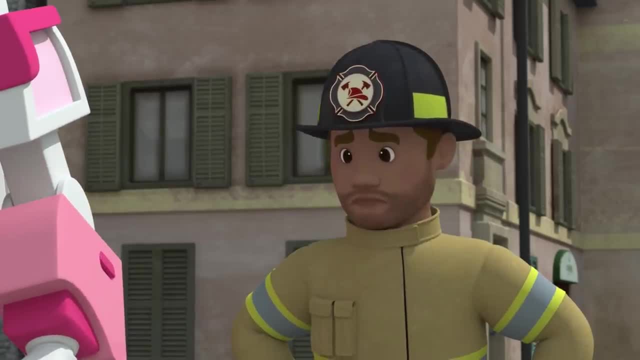 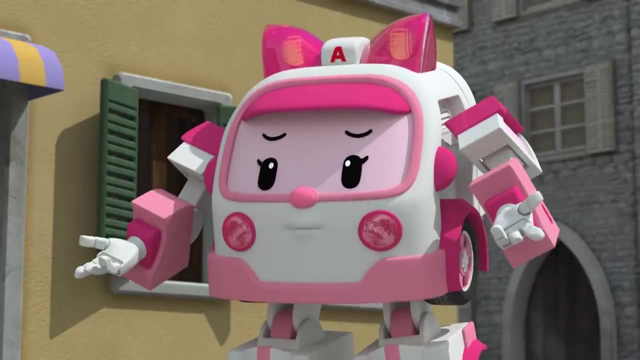 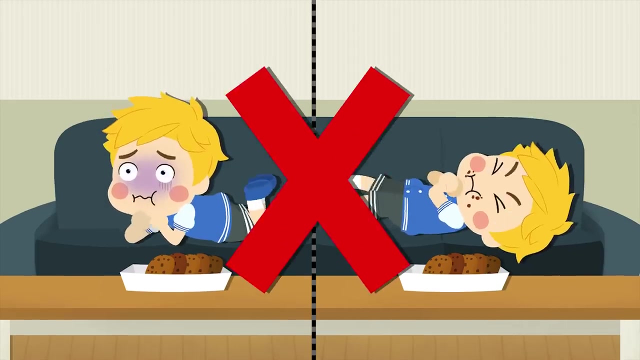 Thank you, Amber. You're very lucky I happened to be near. That was a really close call. I'll be careful from now on. Peter, getting food caught in your throat is quite dangerous because it makes you unable to breathe When you eat. you can't do it lying down. You must only eat sitting up straight. 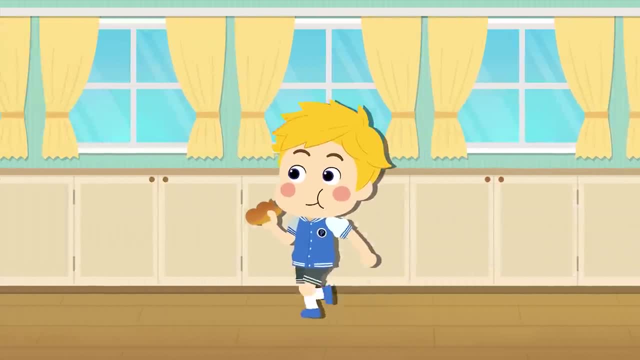 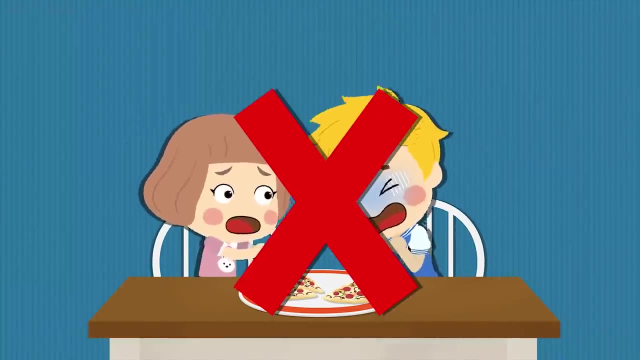 Never eat while you're walking around. Don't talk when you have food in your mouth, because there's a chance the food will get caught in your throat. If food does get caught in your throat and you can't breathe, you should let someone know right away. 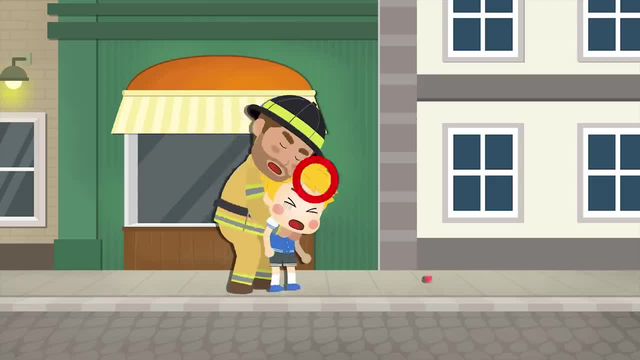 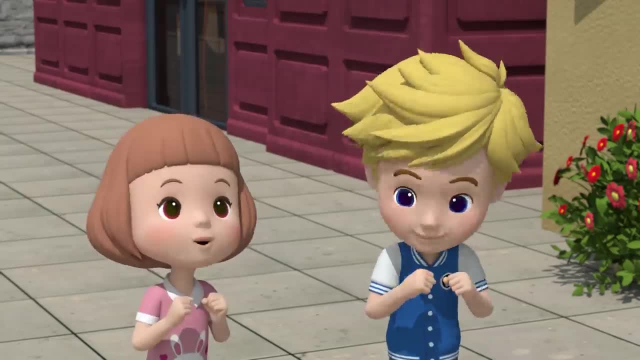 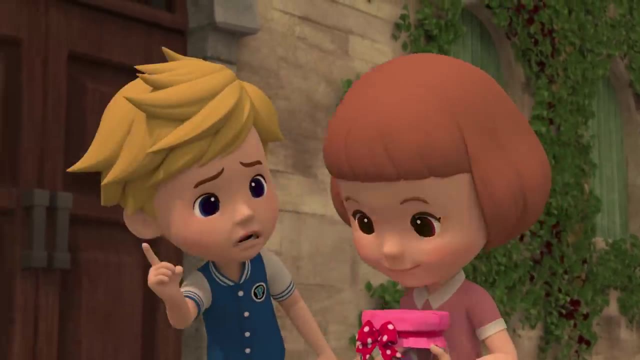 If you can remember that everything should be fine, all right. Oh, I will Amber, Me too. This candy's all mine, Lucy. can I have one? Just one, Amber, just finished explaining to you not to eat while you walk around. You already forgot. 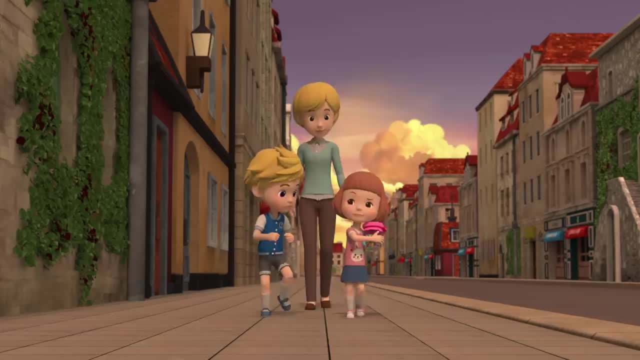 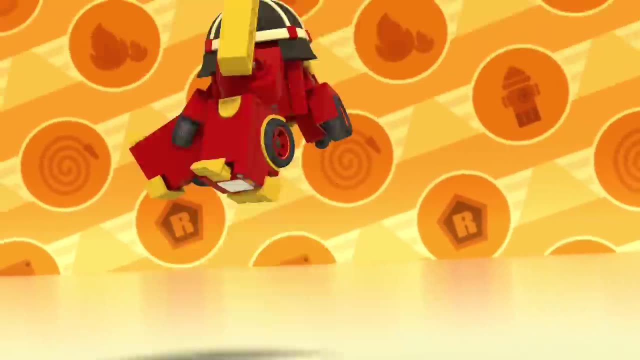 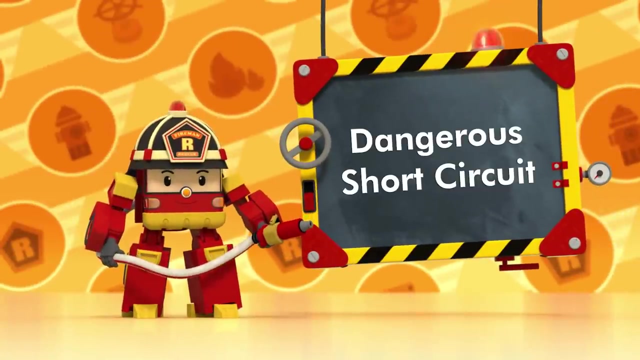 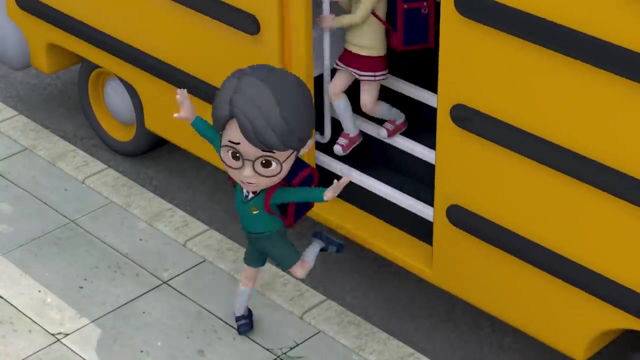 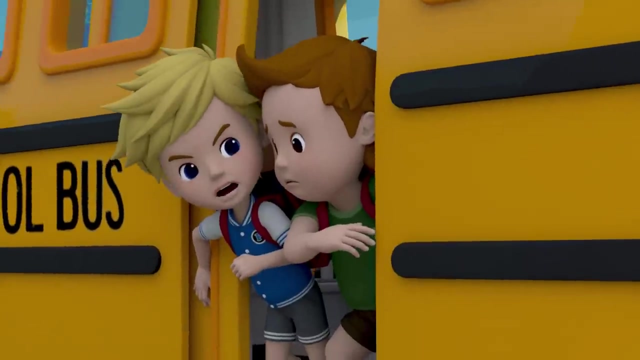 Can I have one at home then? Not a chance, Lucy. please just give me one Please. But I'm begging Dangerous Short Circuit. Goodness, Scooby, are you sick? No way, I'm all right, Let me off first. 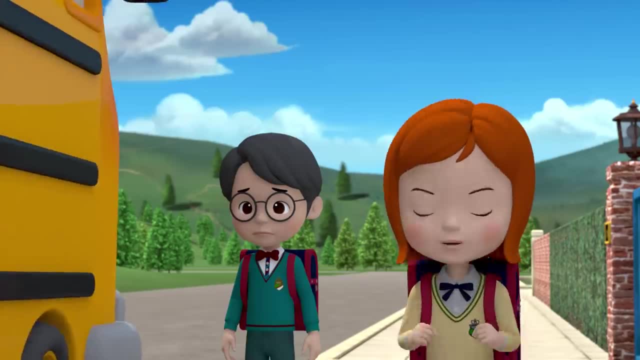 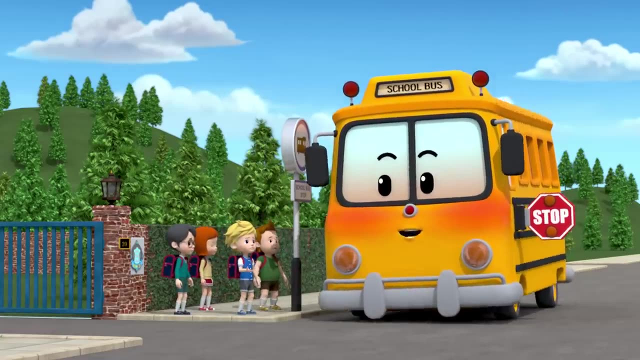 Geez, I got here first. Just let me off. Cut it out. You guys are making Scooby feel even sicker. What Scooby are you sick? Thanks, but I'm all right, guys, You don't need to worry at all. See you after a while. 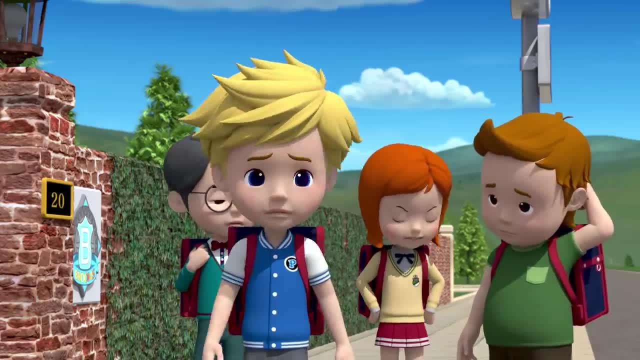 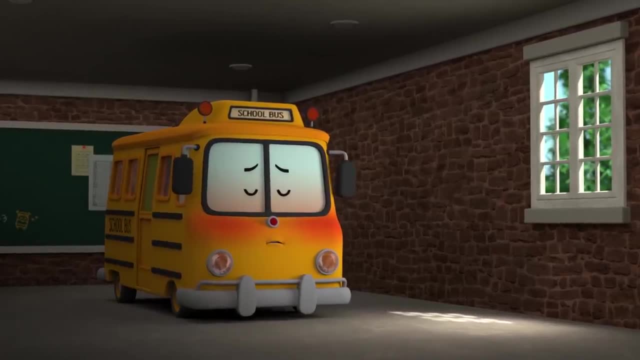 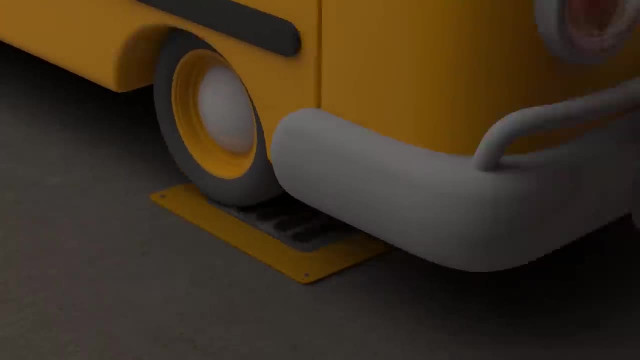 Scooby doesn't look good at all. We made him feel even worse. Nice work, Hmph, Hmph, Hmph, Hmph, Scooby, Scooby, Huh Kids, Hey, Scooby, Scooby, Scooby. we were really worried about you. 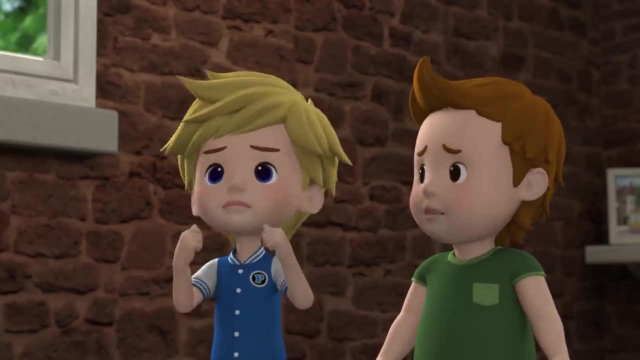 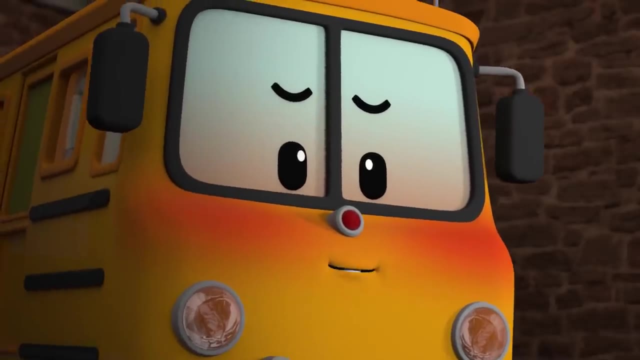 You were Scooby. we're sorry for earlier. Yeah, we're sorry. I didn't know that you were sick. It isn't your fault at all, guys. I've just got a little cold. I just need rest. But thank you all for coming by. 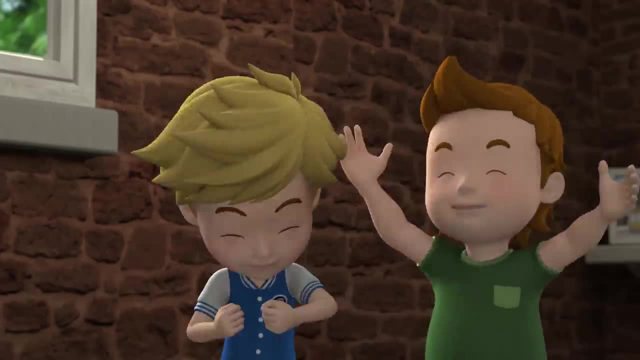 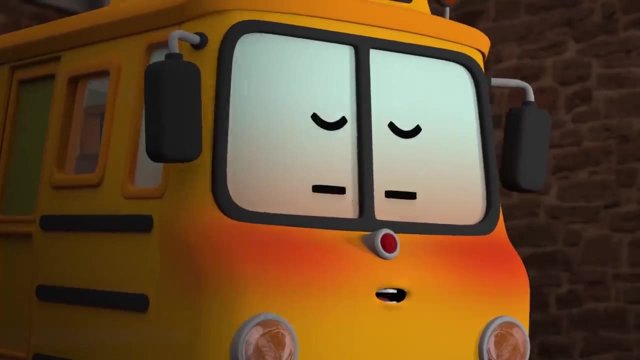 Scooby, Wait, There's more What We brought you, some Get Well stuff. Huh, Just leave it to us, Scooby. We'll take good care of you until you get all better. Yes, we will, Hmph. 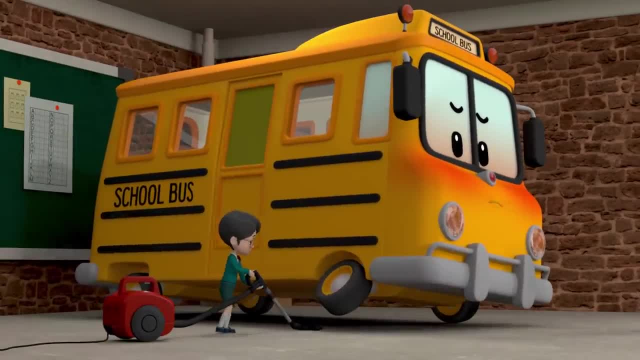 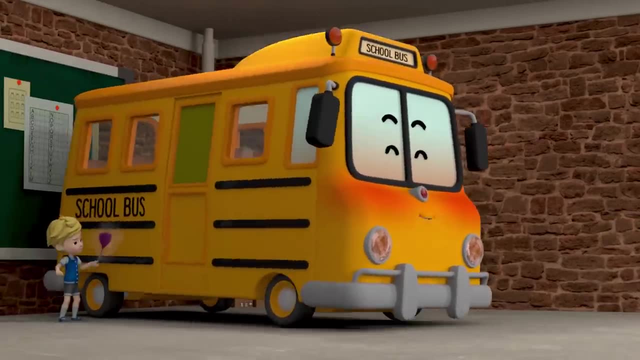 Scooby, can you please lift your tire up? All right, Scooby. where do you put your garbage? Just right beside the door there, Hey, that tickles a lot. There's dust everywhere. We'll freshen you up, Scooby. 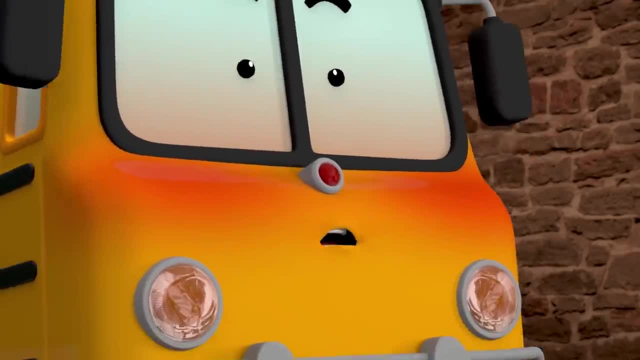 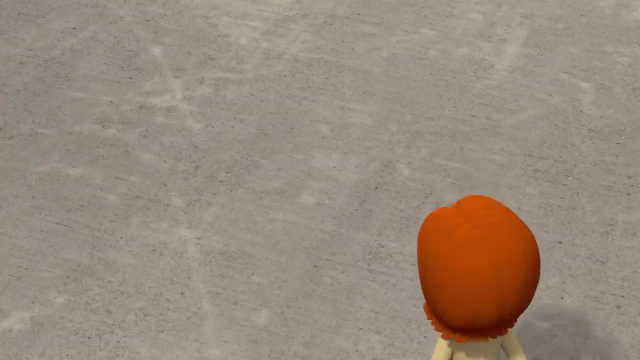 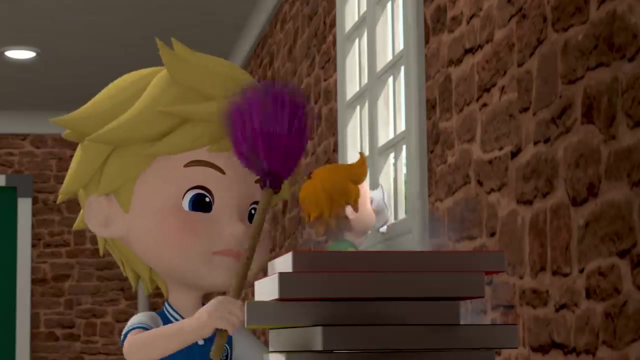 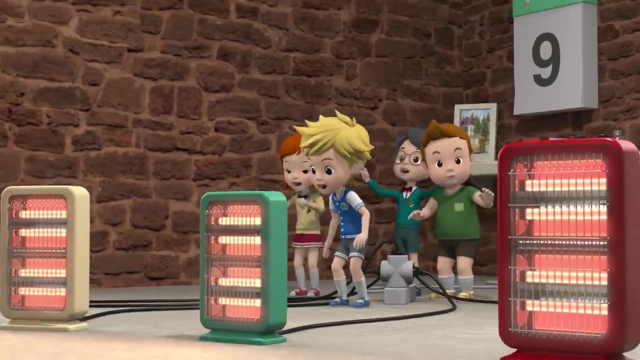 I can't take it. you guys Stop, That's cold. Huh, There, Scooby, How does that feel Cool? That feels nice. Leave everything to us today, There. Yeah, Great work guys, Nice and warm. 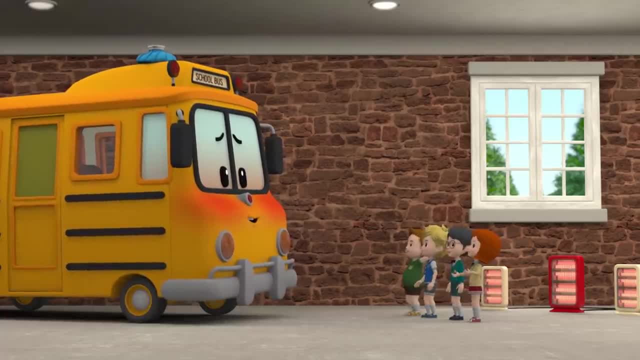 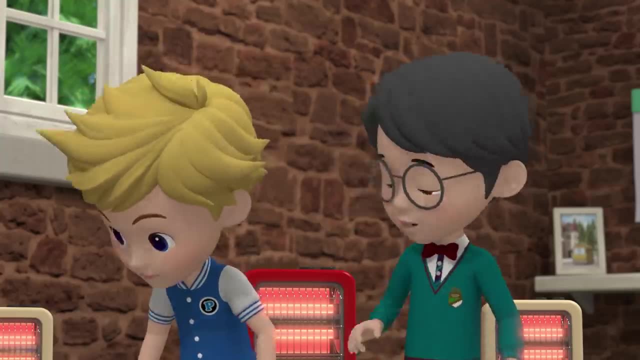 Thanks very much, you guys. You're very welcome. Feel better, Scooby Goodness, I'm really hungry, Me too. Yeah, Good thing I thought to bring A whole bunch of awesome snacks. Ha-ha, Yeah. 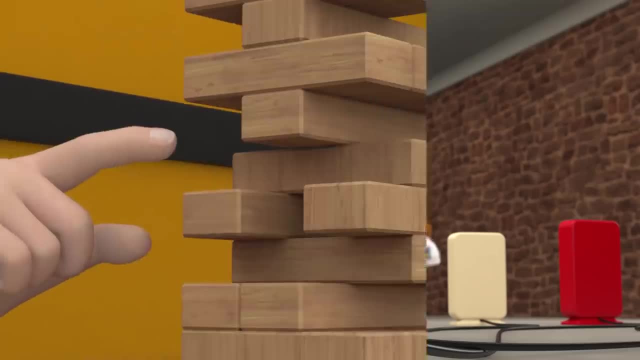 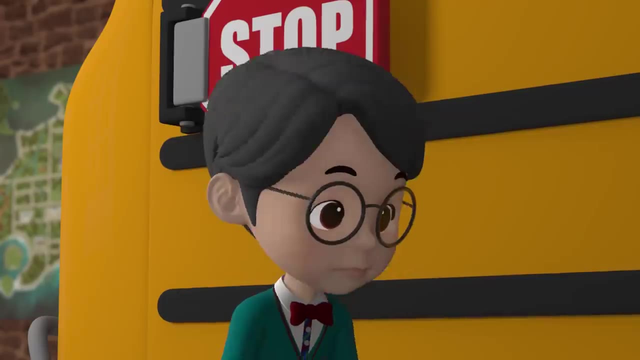 Don't eat food. You're the best, All right, Oh, Oh, And there it goes, Ha-ha-ha, Ha-ha-ha, Ha-ha-ha. Hey guys, Anybody else smell that? Johnny, stop eating bead dicks. 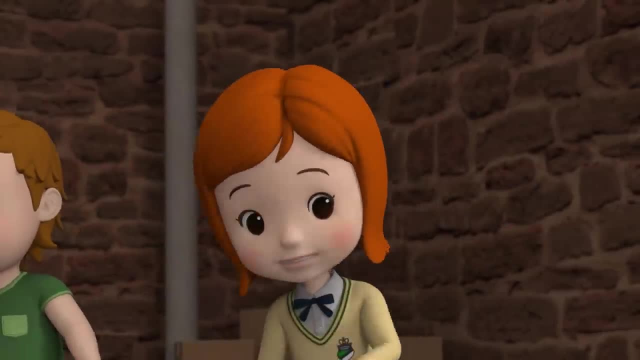 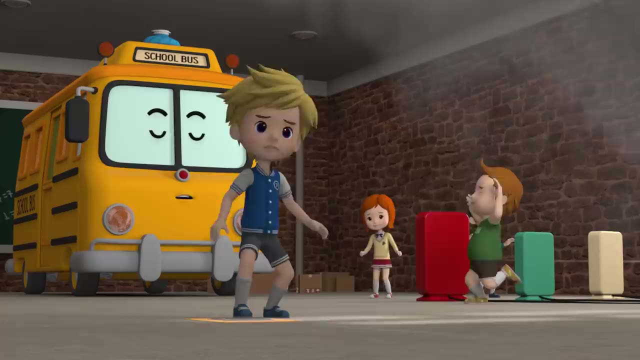 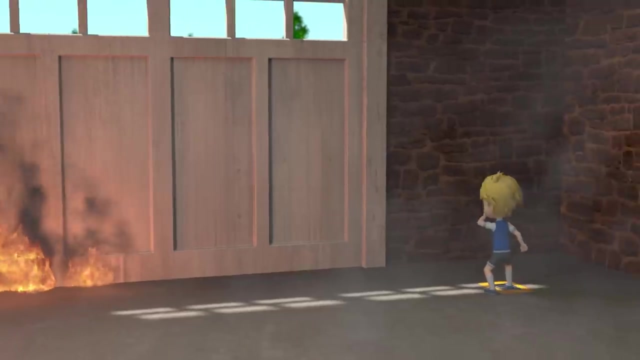 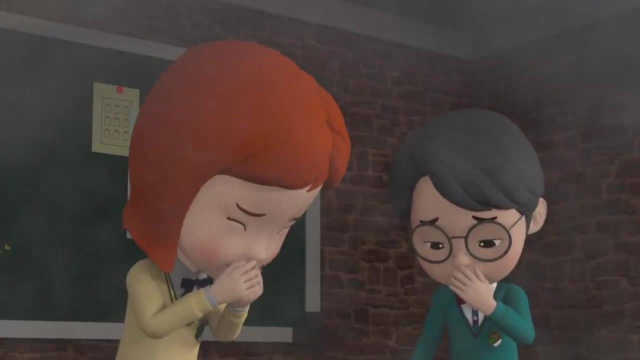 Hey, It's not me. Huh, It smells like Fire. Huh, Scooby. Oh, please wake up. It's a fire. The door won't open. Scooby Children, Hurry, Climb aboard. 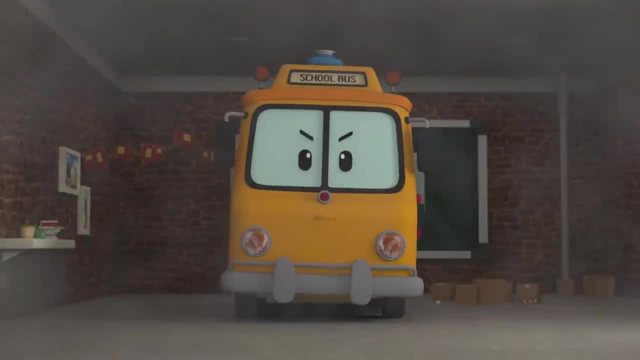 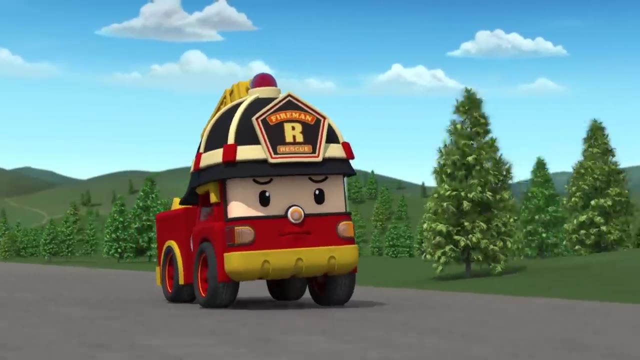 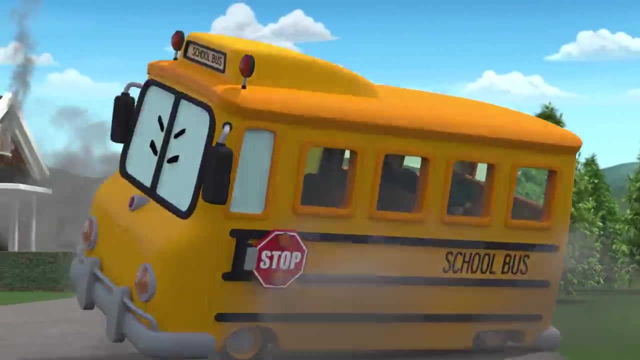 Now put on your seat belts and hold on tight. All right, Huh? Smoke Seems to be coming from Schoolby's place. Look out Now. please take the children somewhere safe Right away. Oh, Oh, Oh. 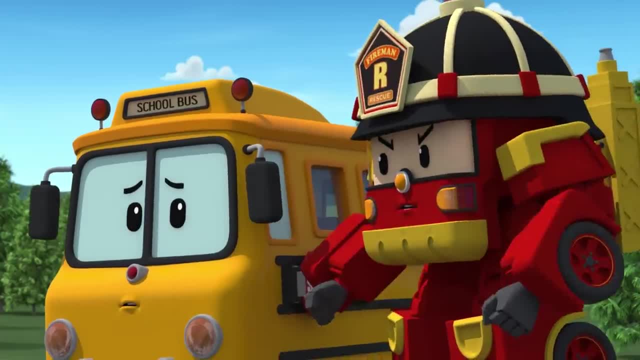 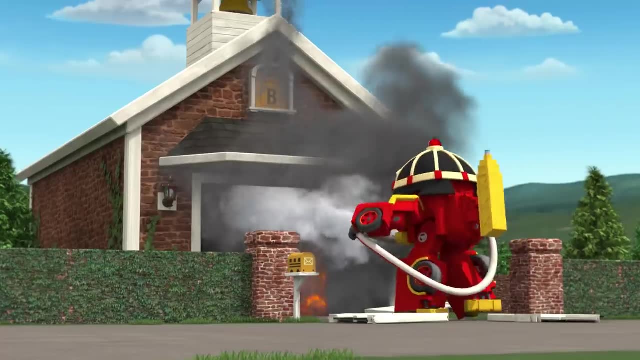 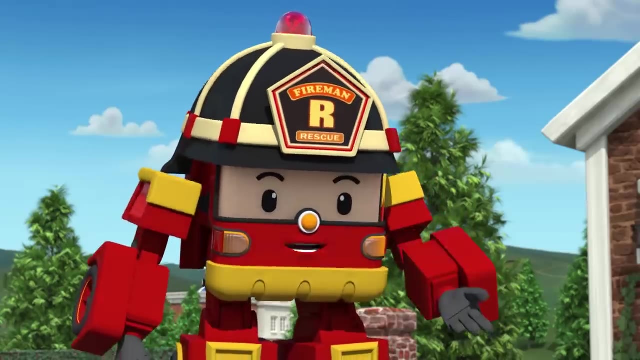 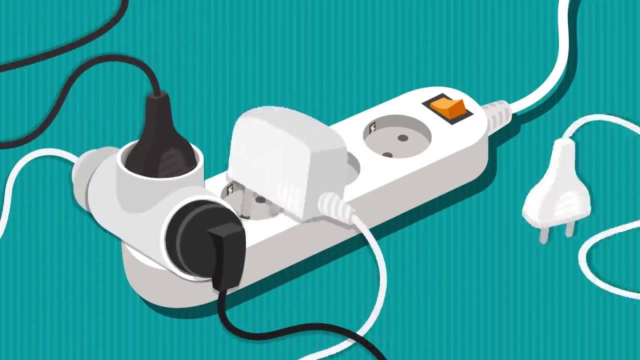 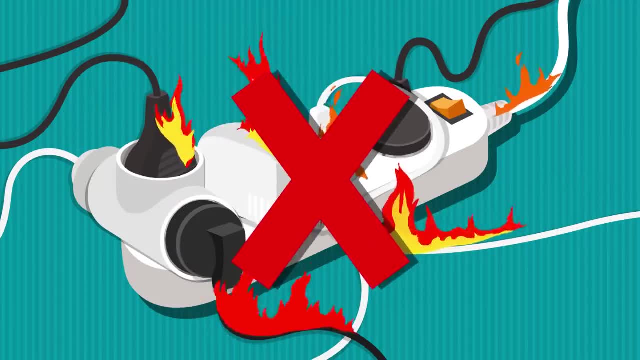 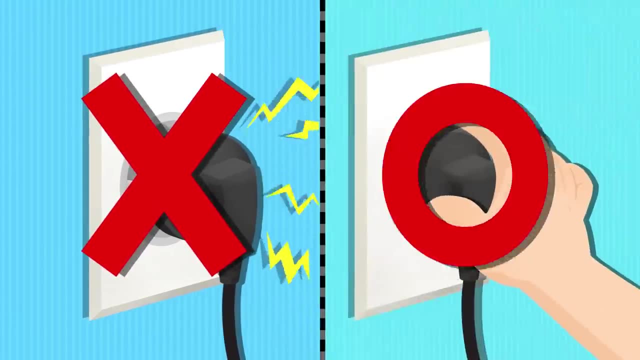 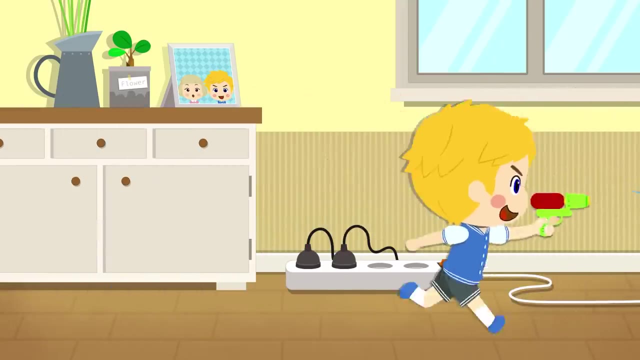 When you plug in devices, don't plug in too many at once. That much current flowing can overheat the outlet, which can lead to a fire. the way can cause sparks to occur, which can also start fires. Lastly, make sure the insulation on the wires doesn't peel off and that water never gets in the 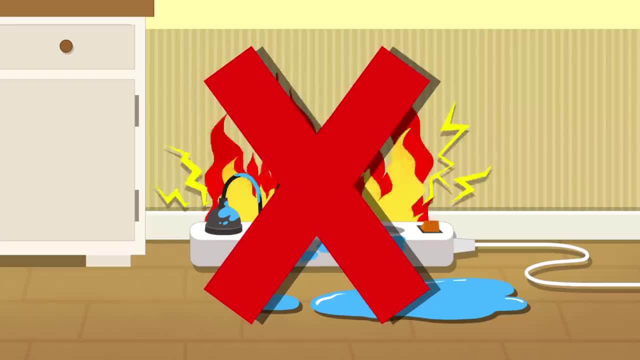 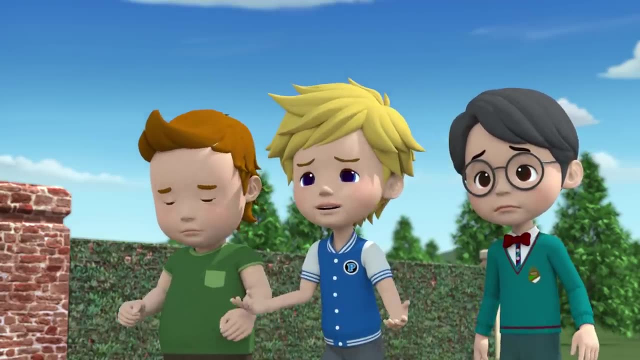 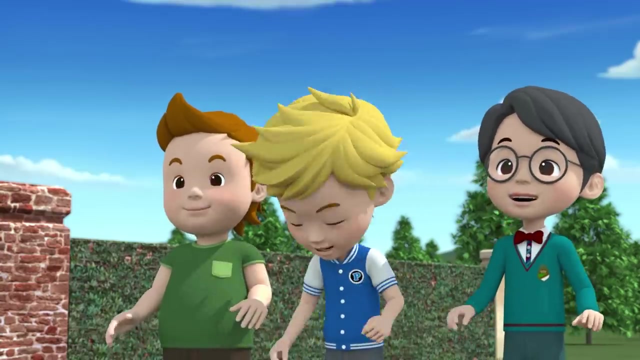 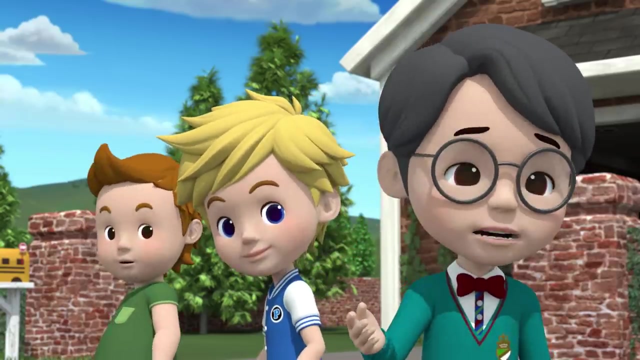 plug. A short circuit can cause a fire too, Do you understand? Yes, Thank you, Roy. Sorry, Scooby, I only wanted to help. It's fine guys. You made me feel so much better. I'm not sick anymore. You're not. It looks like you might have come down. 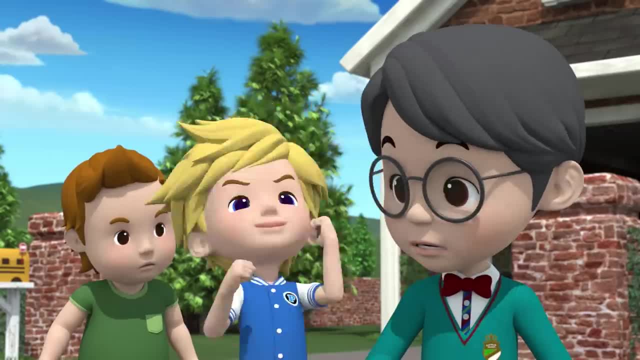 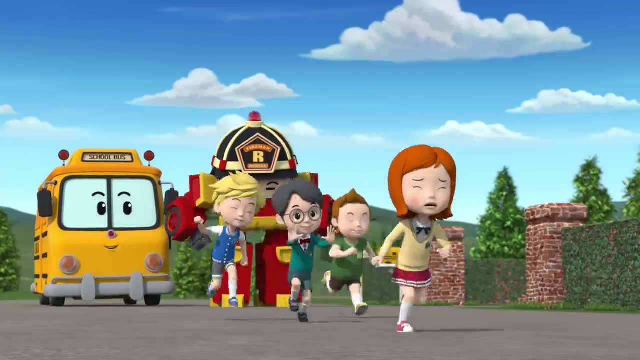 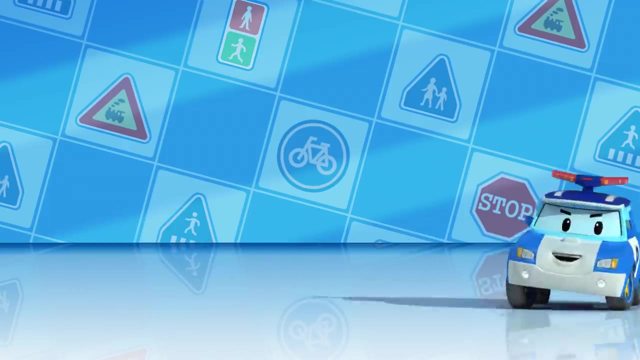 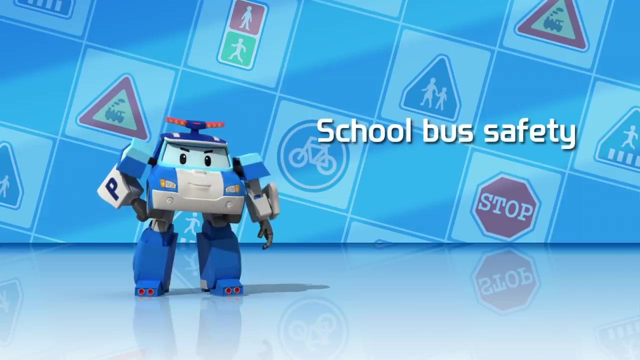 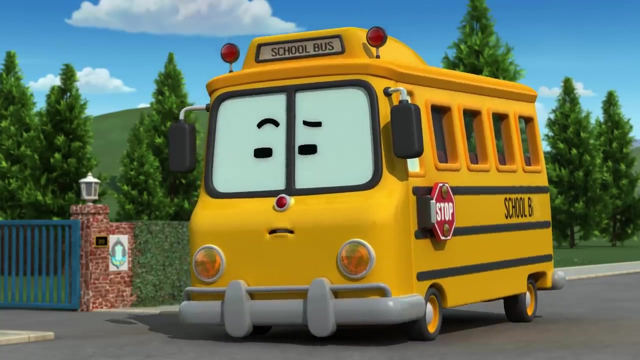 with Scooby's cold. Yeah, guess it's Cindy's turn right, Cindy, we're here to help, I'm fine. thanks, I'm very fine. Oh, I sure wish Gin would hurry. The kids will be out soon. 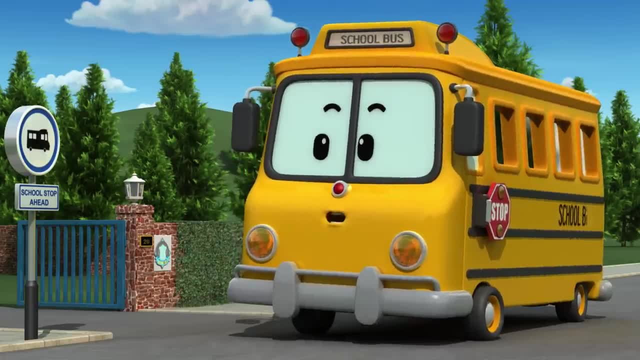 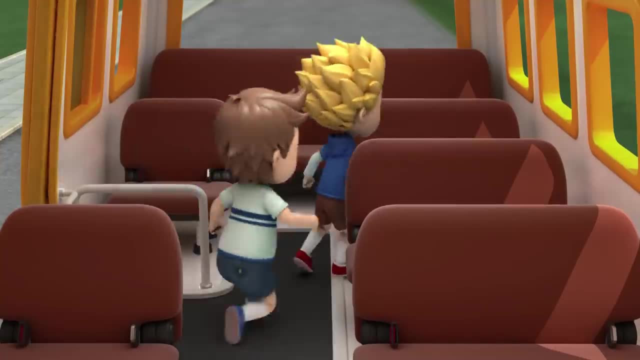 Look, Kevin and Doug are here. Hi, Scooby, Been waiting long, Scooby. No, not really, I get the window No way. Excuse me, It isn't safe to misbehave on the bus boys. 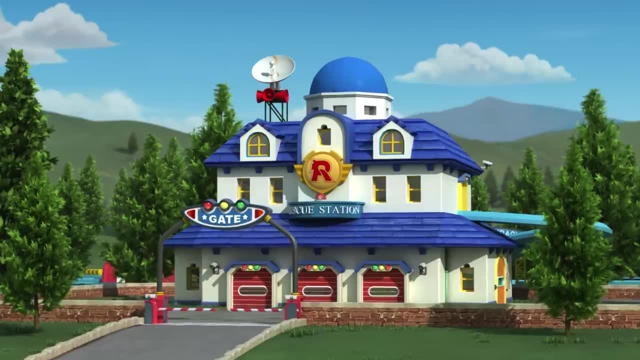 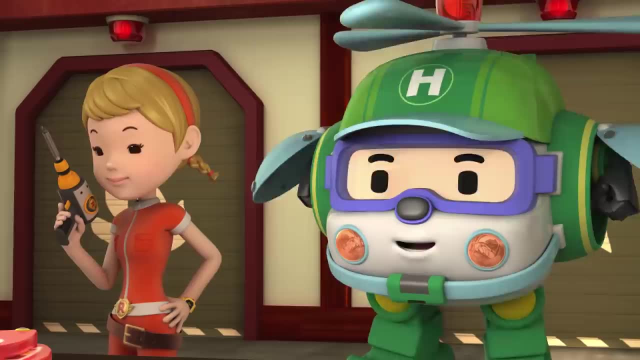 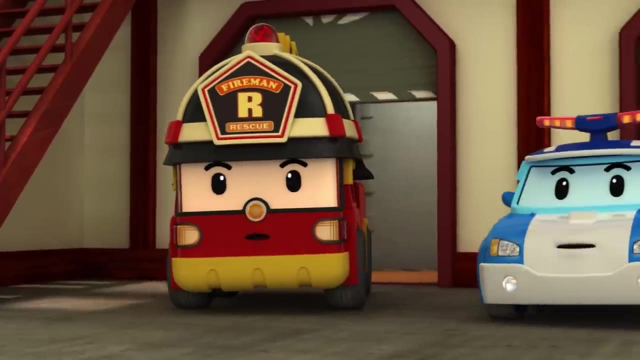 All right, that should do it. What did you make this time? Gin Scooby asked me to come up with a boarding guard. so What's a boarding guard? Well, it's a safety device that'll help kids get on and off the. 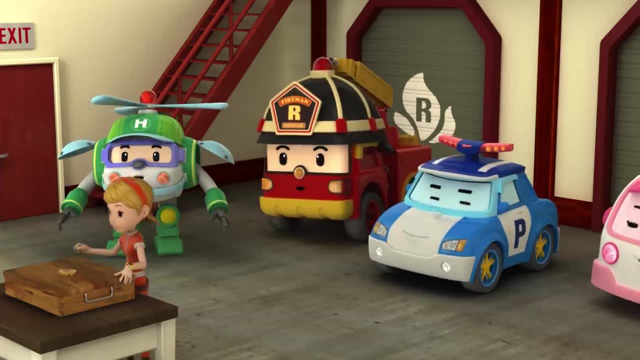 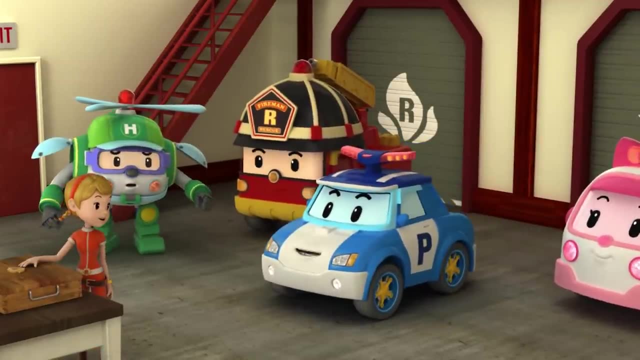 bus safely. Oh, what time is it? I was supposed to get this to Scooby. I'll take it to him, Gin. I'm going out on patrol now. Thank you, Polly. Scooby will be so pleased. I hope so. 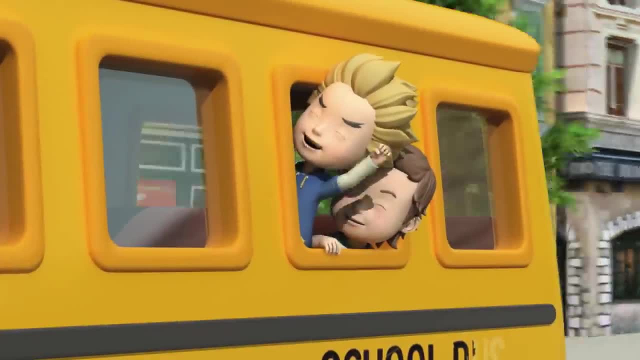 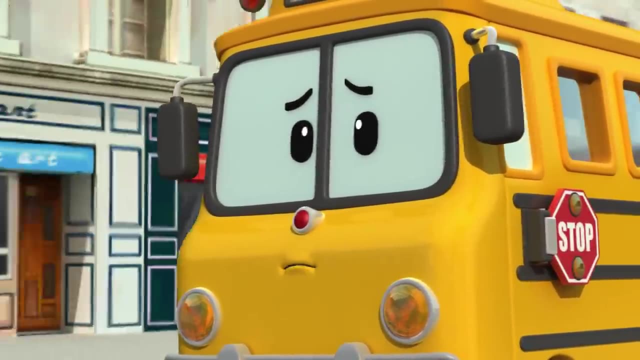 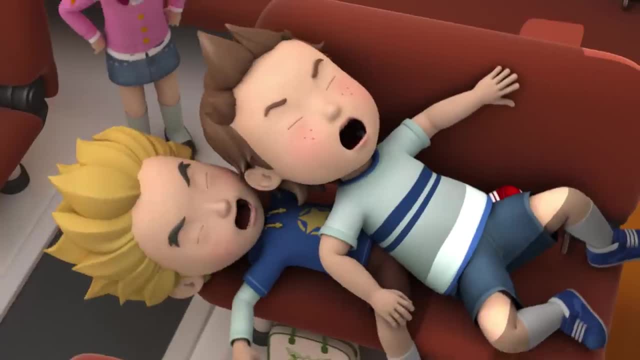 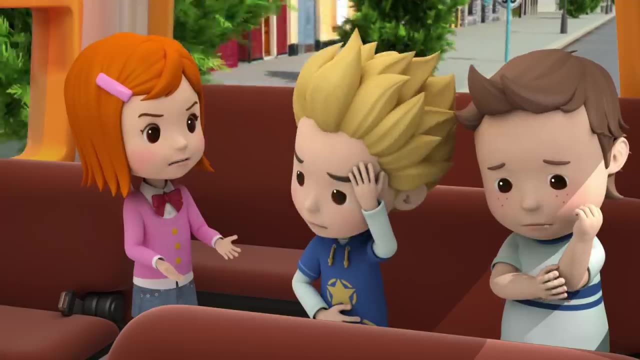 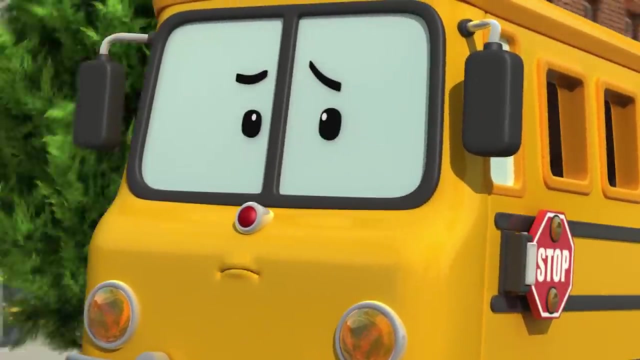 He was right, wasn't he? Yeah, Why can't you two just sit still when we're in here? What's the matter with you? I'm listening to you. Please settle down. I need to focused on driving. Please get back to your seat, Ginny. 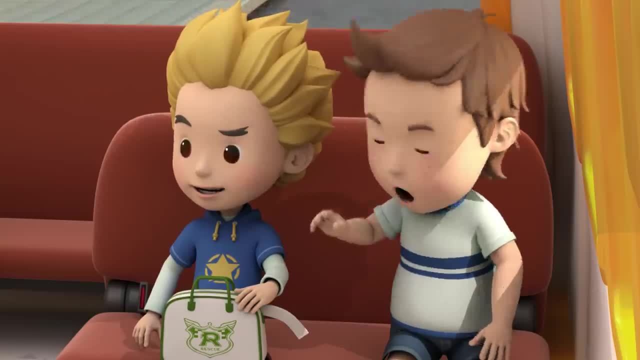 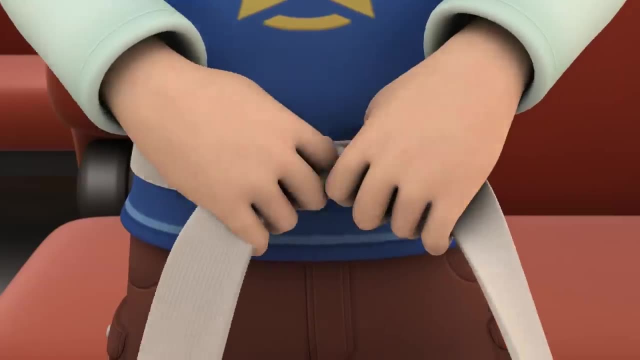 Yes, Scooby Kev, what's this? Hey, Don't touch it. Oh, This is the belt I wear for Taekwondo. Taekwondo, Yep, I'll show ya Taekwondo, Oh yeah. 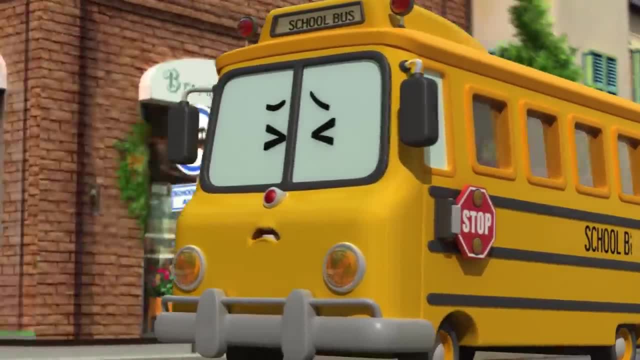 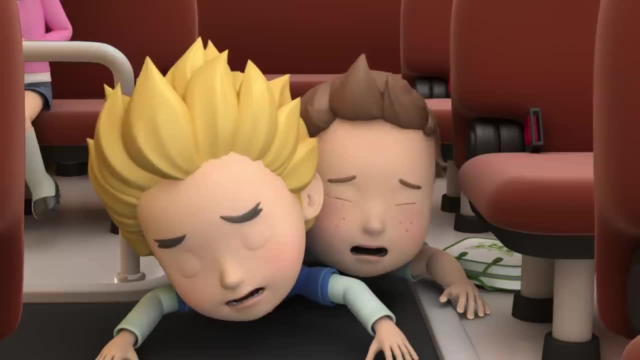 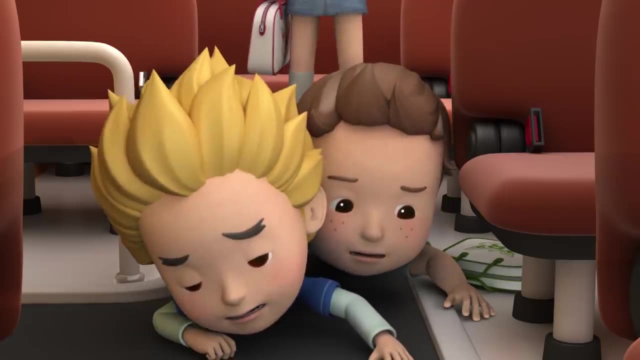 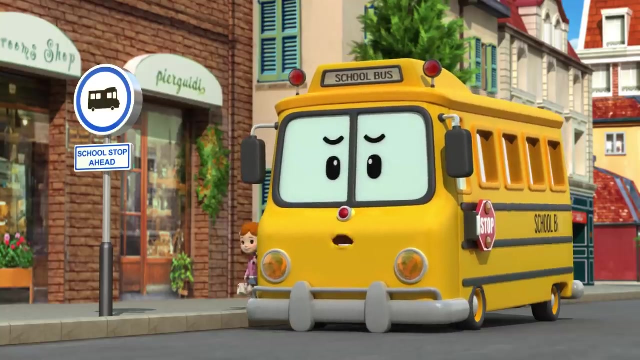 Oh, oh, Please stop it. boys, Scooby, I get off here. Oh okay, Jenny, Scooby, Are you all right? boys, Excuse me. Huh, Whoa, A red belt. We're at the gym, Kevin. 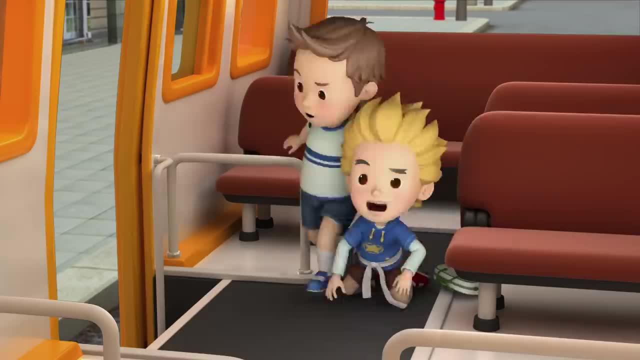 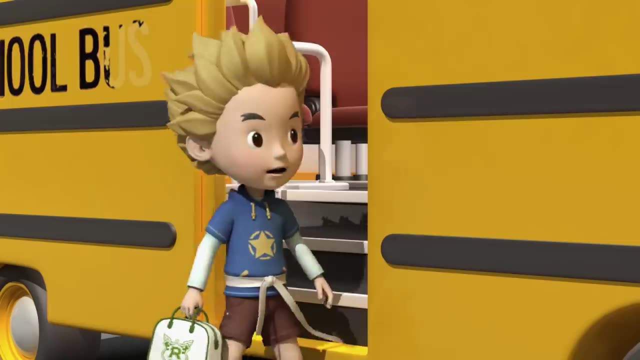 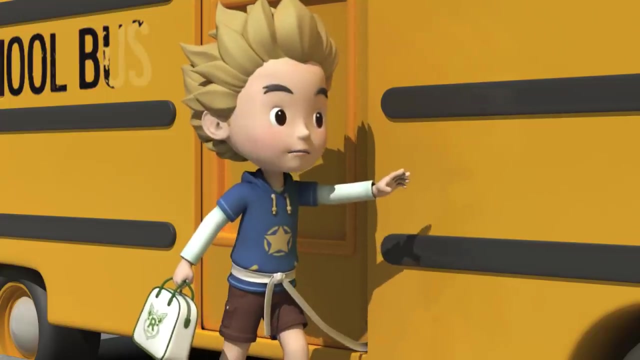 You need to get off here too. That's right, Me too. Wait for me. Oh, Doug and Kevin are off. What a relief that is. See you tomorrow, Scooby. Oh yeah, Hey, wait up guys. 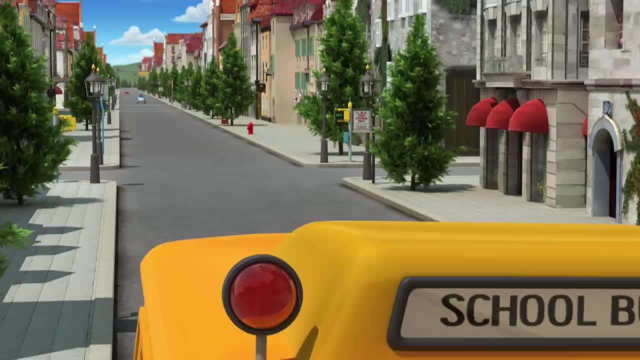 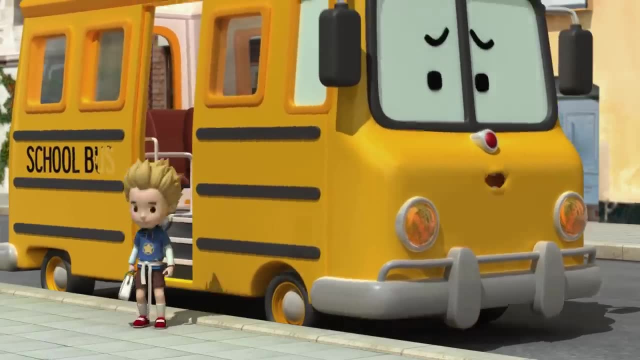 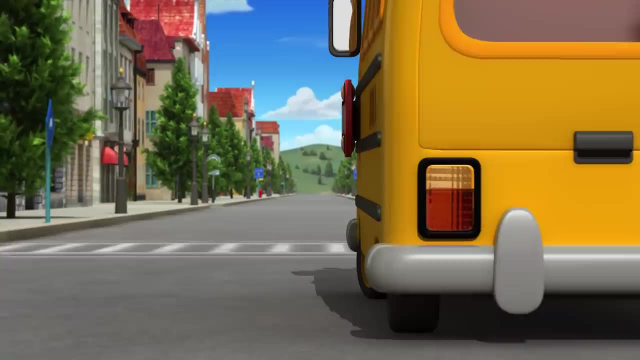 Oh, What's wrong, Kevin? Oh, Scooby, Sorry, Didn't see your belt get caught, Are you okay? Yeah, I'm okay. Hey guys Wait up. No, Kevin, Wait, Whoa, Whoa. 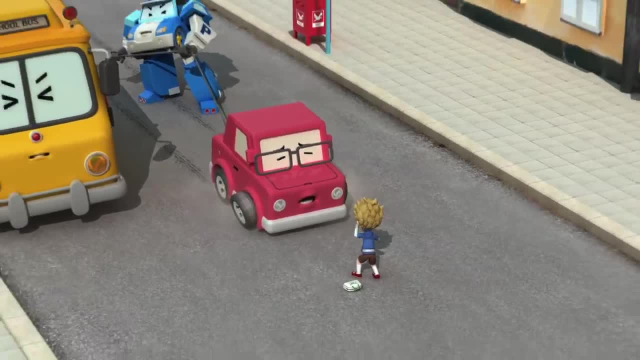 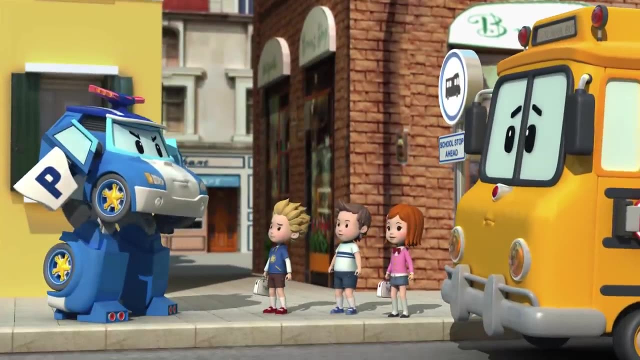 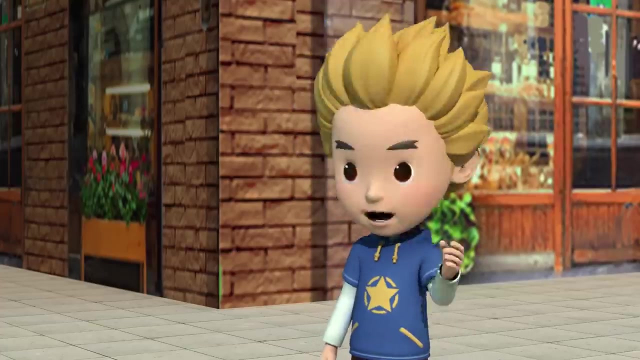 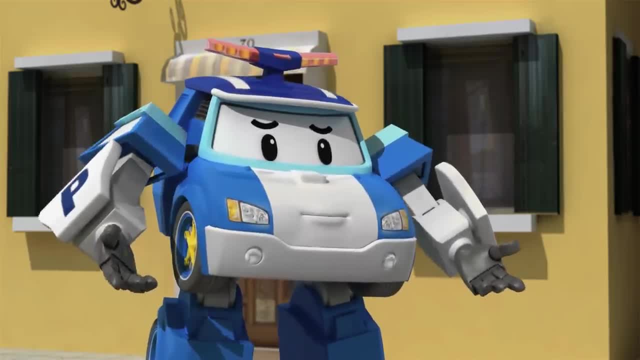 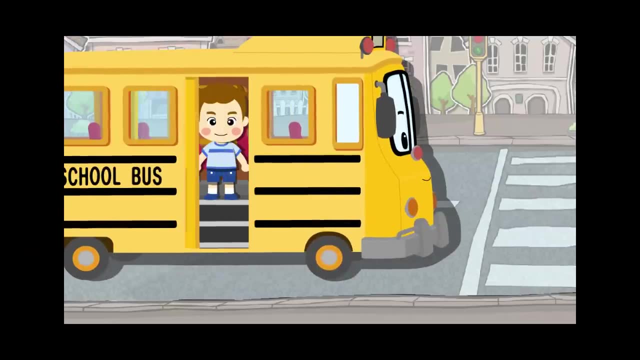 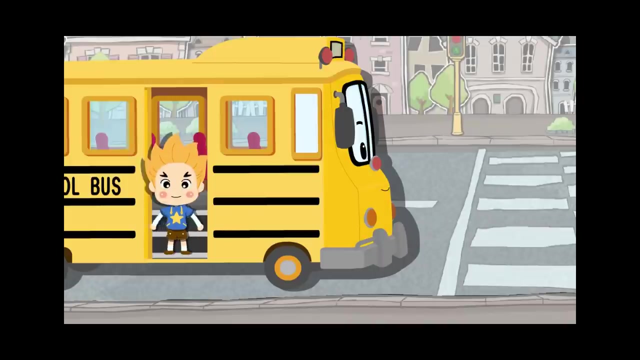 That's my point. You didn't follow the safety rules. Okay, can we go through them again? Yeah, When you get off the bus, a motorcycle or bicycle might be coming. Always look both ways first, then get off slowly After you get off the bus. 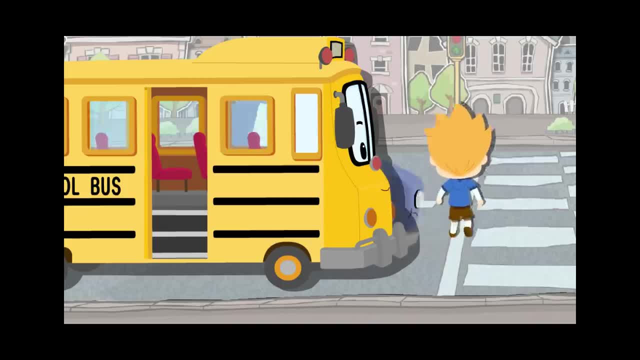 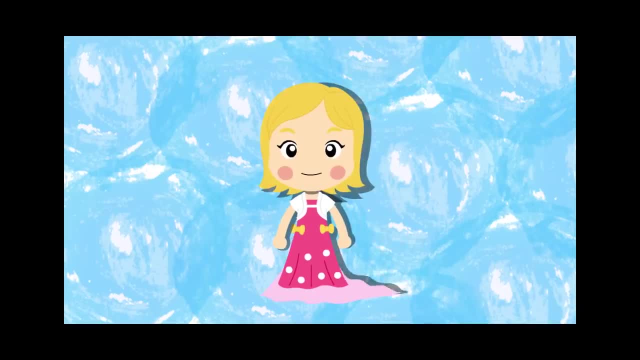 never run around the front to cross the street. Drivers can't see you, and that's dangerous. Always remember that the doors on a bus or van can be very dangerous too. If loose clothes or bags or even belts are hanging out, they can get caught in the doors.